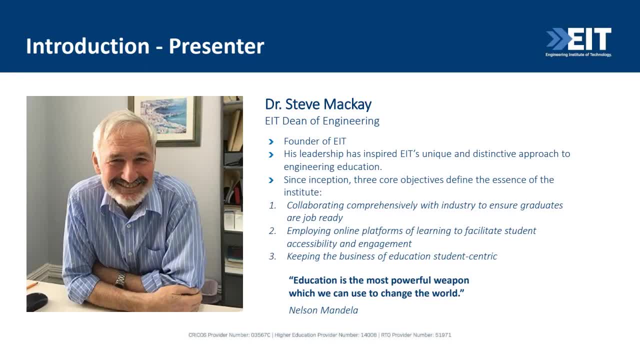 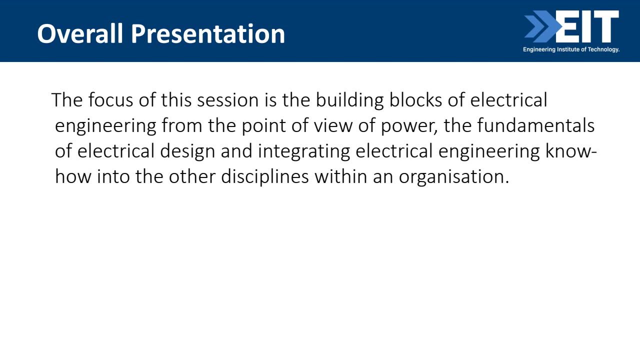 What we've got today is about a huge amount of material. Obviously, I want to do the whole of today's session in 45 minutes. 45 minutes is what we want to do today. If I talk longer than that, I'll bore you. guys and ladies, There's about 140 slides. Obviously, I won't cover every. 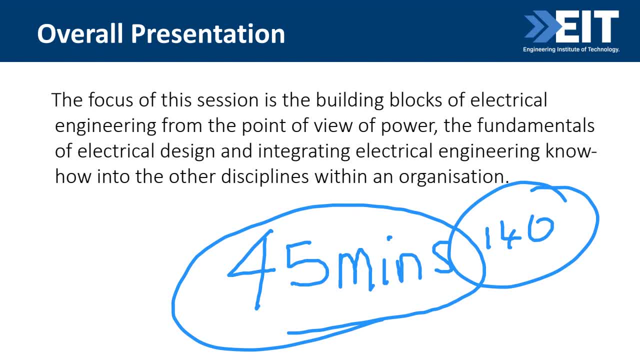 slide. I will cover the key ones, but you will get copies of all the slides. Don't fear, Everything will be provided to you. You will get the whole lot. In fact, it forms part of the larger three-month course. I've just taken the key bits Now also, I just want to tell you now that you 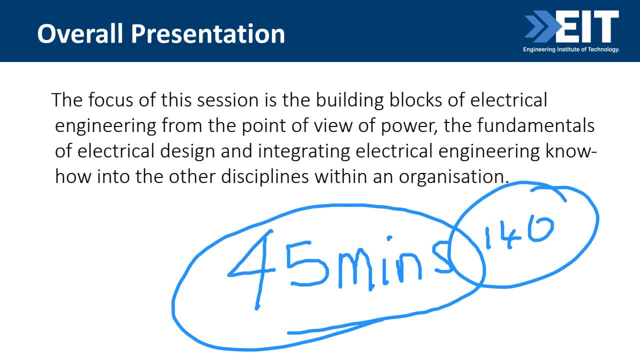 won't become a electrical engineer after 45 minutes- although I'm sure there are many electrical engineers amongst you- but you will become a little bit more knowledgeable And if you go through the slides and the additional learning materials we give you, you will become very knowledgeable. 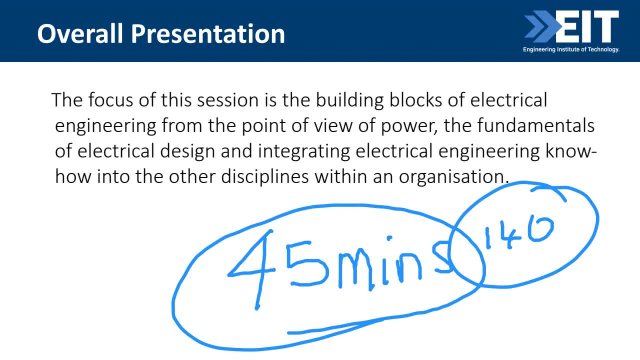 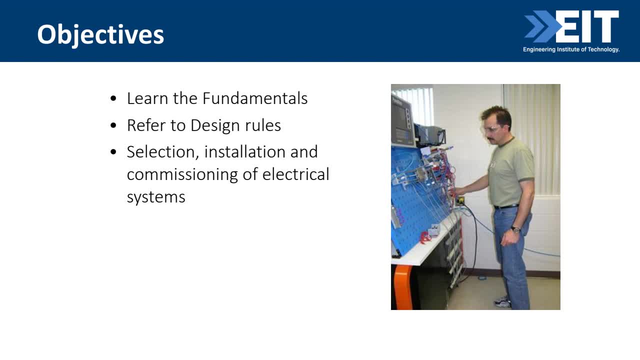 So don't fear that this is a waste of time. So I'm going to cover the key elements, Fundamentals- and I'm sure there's lots of engineers here- Design rules And commissioning of electrical systems. Now I just want to just also again mention we are 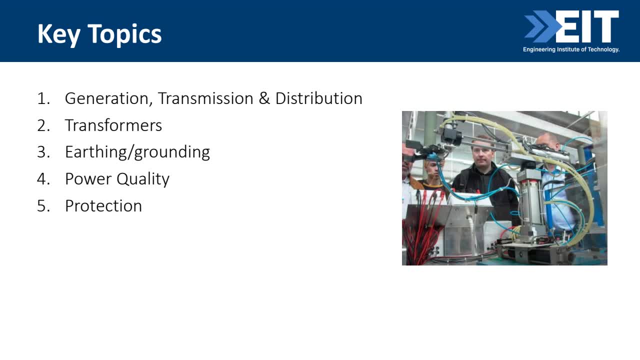 covering the IEEE standards, which is the American standards, the IEC and also I'll be specifically mentioning Australian standards as well. So there is a mixture of standards. So please don't say, Steve, it's wrong, This is the right standard. You know, you've said 1 ohm, It's actually 25 ohms, for. 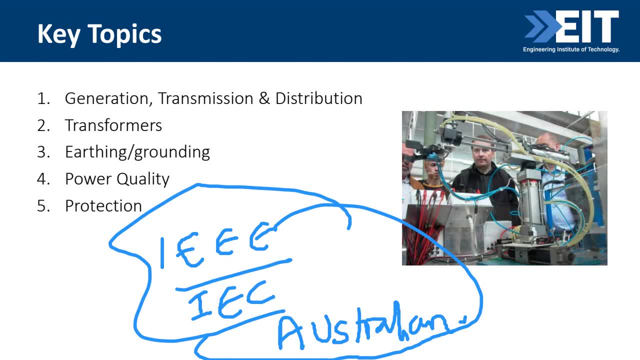 earthing resistance. I am trying to globalize, of course, because you people out there are all from all over the world, So I want to try and be as general as possible. So please forgive me for being a little bit perhaps generalized. It's not always a good idea. but I will cover the different. 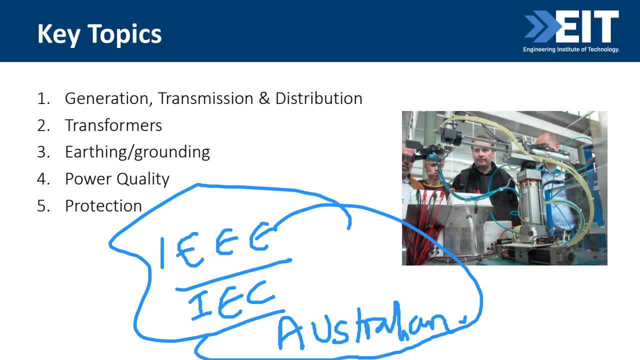 standards And, as I said, I want to do it in 45 minutes, but there's plenty of materials here to go well beyond that. And after each section I've got a little quiz And in the quiz I want you to be able to answer in the 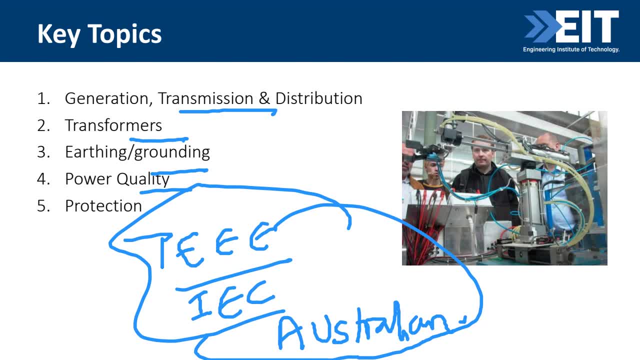 chat box. So please don't talk, but you can say hello, Let me just say chat. You can all see the chat box. Please answer the quiz here, Okay, And if you disagree with anything, please put it in the quiz and I'm all ears and I will reproduce it. So what we're going to be doing today is 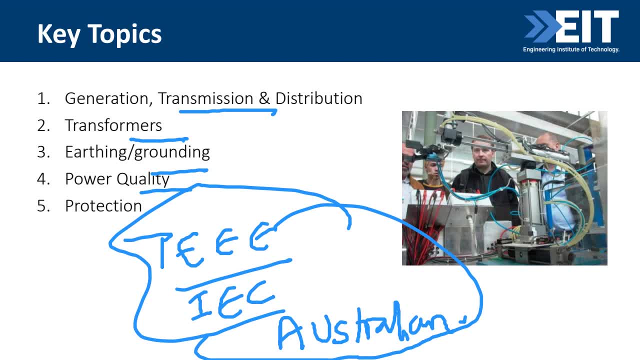 first of all, generation transmission distribution. I just want to talk about what that is: Transformers, those curly devices which have very low losses. Earthing and grounding, which is a topic after my own heart. In fact, we just 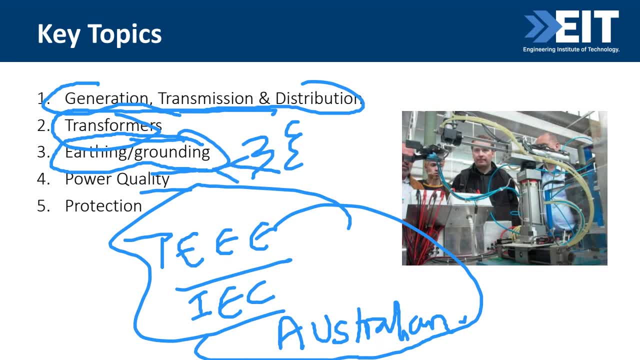 run a conference in Birmingham in England on that topic: Power quality and then protection. So those are the main groupings today And, as I said, we will be going through lots of material, but I will just go through the key things Now. 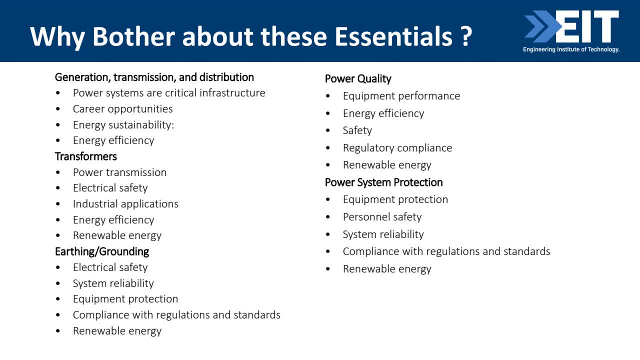 the first question you should ask is: why bother about these topics? And I've listed, I've headed all the topics here: Generation, transmission, transformers, earthing, grounding. Why bother? Well, there's a reason here. Obviously, power systems are critical. Your career opportunities are. 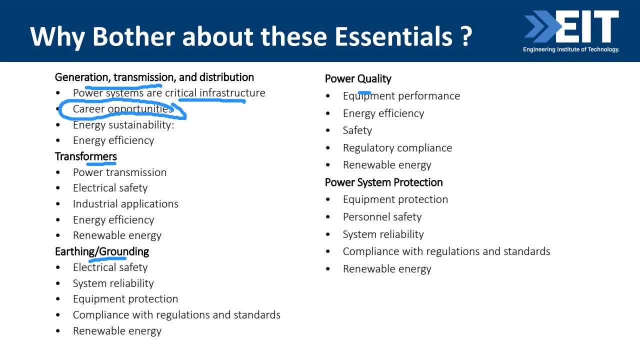 related to power generation, particularly particularly in the solar and wind- and renewables. Energy efficiency is really, really important. If you look at transformers, they are critical in power transmission, Energy efficiency, renewable energy- they're becoming important as well. Earthing and grounding. why is that important? Well, you've got things like safety very 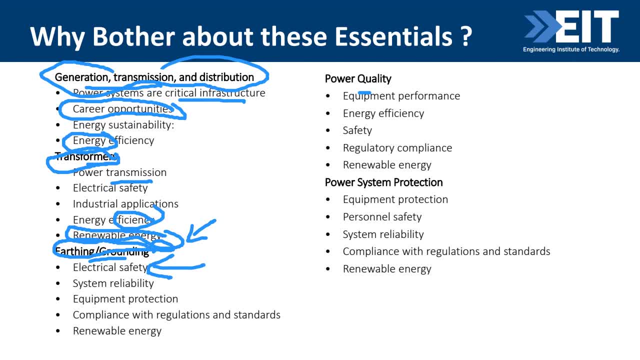 important, One of the most important things in life is making sure you look after your fellow man and woman in terms of safety- Absolutely critical- And system reliability, equipment protection and, obviously, compliance, regulations and standards. And the other thing, which is earthing and grounding, is becoming important, is is: 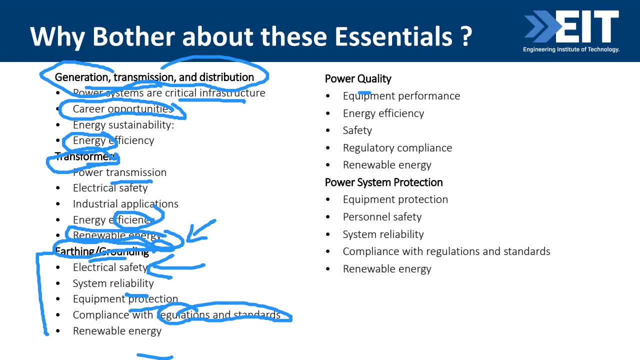 renewable energy because it's a completely new bunch of generation issues. Power quality has been around in a long time, and why is that important? Well, again, energy efficiency. You'll find that renewable energy is causing some dynamic issues with power quality and then power system protection. why is this important? well, protection. 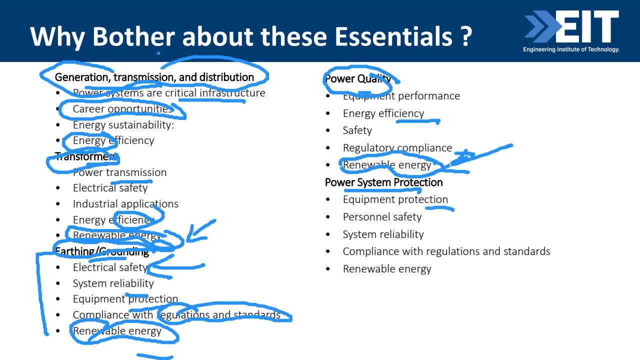 of your equipment so you don't blow it up. obviously, safety, so you don't get killed or hurt. and again, renewable energy is becoming an issue as well, so hopefully these are all reasons for you listening in for the next 40 minutes. so, first of all, power generation, transmission and distribution. 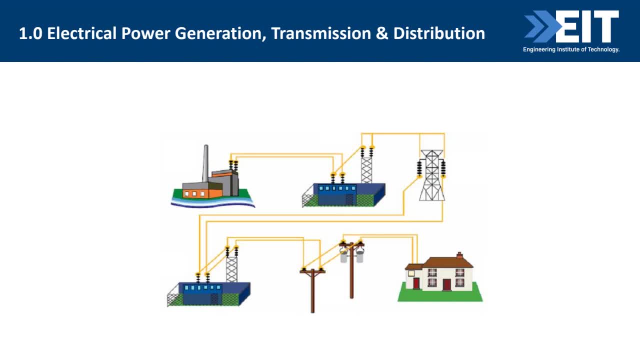 this is the first topic and I've got it here. boom. and, by the way, we had about 1,700 people registered today. unfortunately, we can only take about 400, so the people that can't get in will be getting a copy of the slides and obviously the recordings, as you will, so don't fret, we've got. 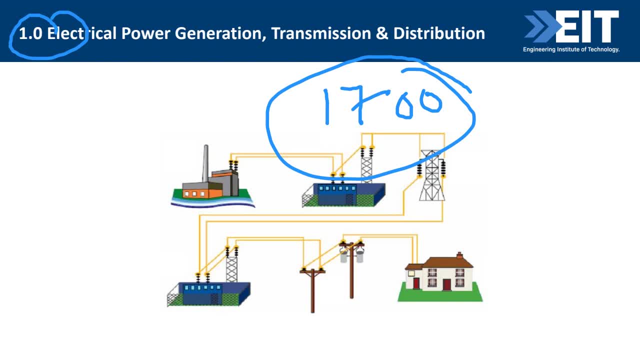 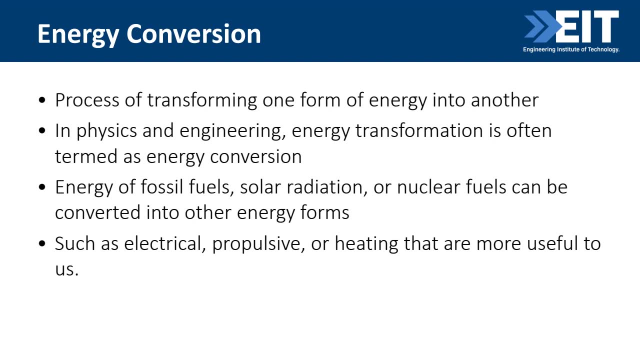 about 300 here now. so welcome, welcome to the team. so obviously you you. energy conversion is transferring from one energy form to another. that's important, and obviously one of the big focuses today is solar and wind and obviously nuclear is another really, really interesting one. now, at the risk of being shouted down by every dog in town, 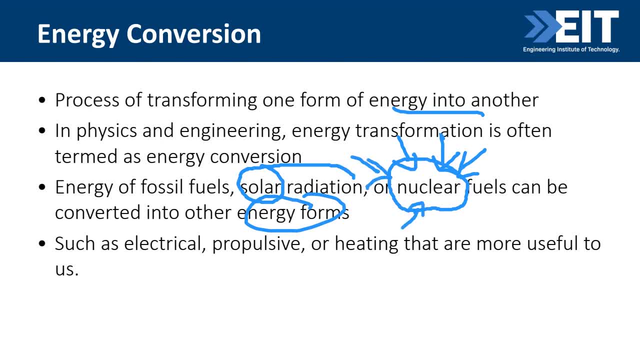 everyone in town. please bear in mind: nuclear should not be discounted. please think intelligently about nuclear power. it's not a stupid, dangerous idea as many people think. it's not a stupid idea as many people think. in Finland, the Green Party is even supporting nuclear power, so you know. 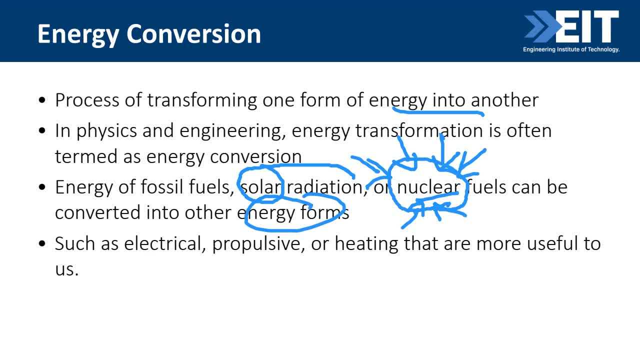 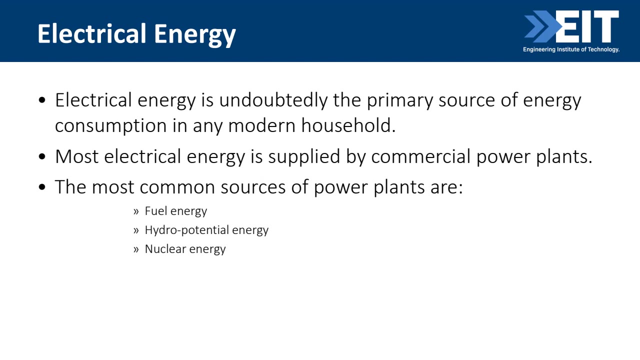 this. there are potential issues there where it's useful. unfortunately- and that will be one of the quiz questions- is fossil fuels is a very much a key builder and it is poisoning our lives, but again, there are some issues there. so electrical engineering is what it's all about and the most important sources of 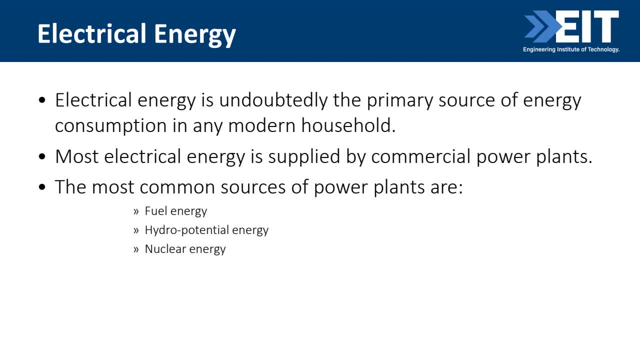 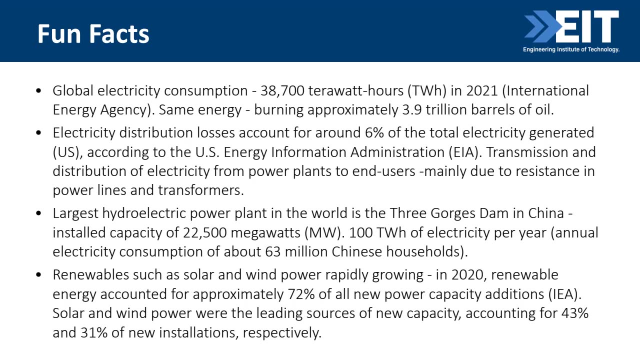 power plants are coal and hydro and obviously nuclear. as I said, you can be a little bit irritating, so there are few facts here just for you to think about and to reflect on, if I can ask you to reflect on it. Mr Shaheed Hussein Rizvi, welcome to the team. some of the global facts is: 38.7 terawatt hours. how much is it terawatt? please put in the box. 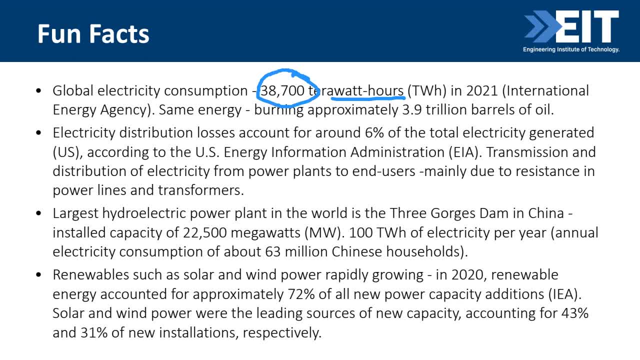 please tell me how much is the terawatt 10 to the power of 2,, 3,, 4, 5,, 6,, 7,, 8,, 9,, 10, 12? yes, thank you, Mr Raj. Mr Raj, thank you very much. 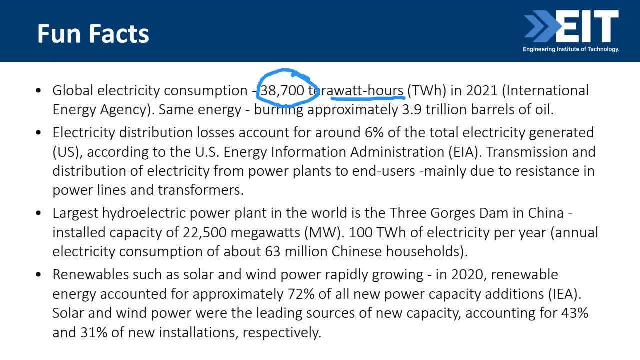 absolutely 10 to the 12. so 10 to the 12 is what it's all about. that's a huge amount of power and it also is equivalent to 3.9 trillion barrels of oil. can you imagine the pollution with all that oil? not that oil is bad. we do need energy. 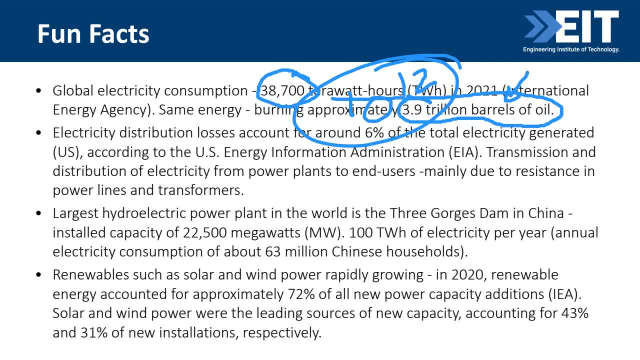 we do need energy. I'm not saying it's bad, we do need energy, but it does create a huge problem for emissions, so it is worth replacing with something. electrical losses are 6% of that is wasted. 6% is huge. get your calculator: 0.06 times. 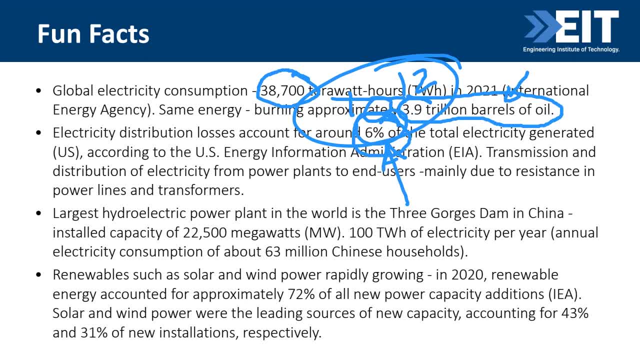 38,700 times 10 to the 12, that is a huge amount of energy wasted, and so that's a big issue for you as a designer. the largest hydroelectric power plant in the world is 3 gorgeous dam in China: 22.5 gigawatts. 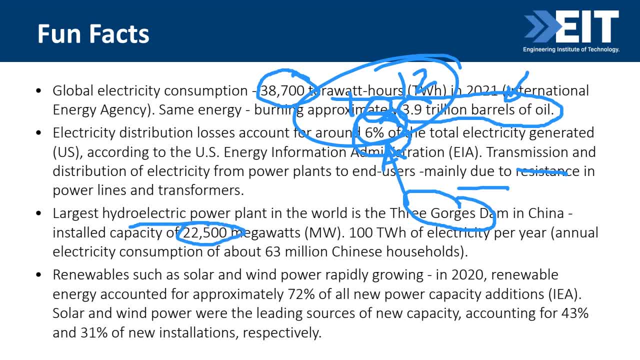 good gracious me 22.5. it is horrific how big that is, and it's hydro as well, so it's clean. now, if you multiply 22,500 megawatts times 10 to the 6 times 3, 5 days in a year times 24. 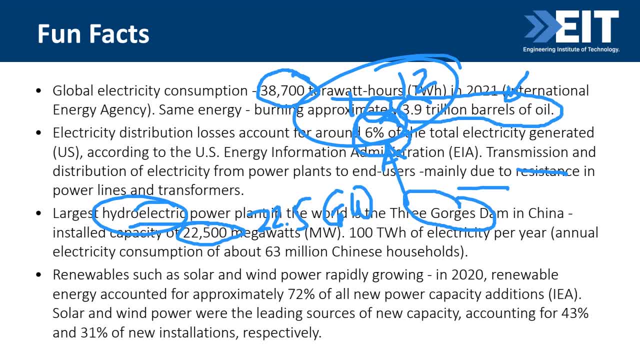 you won't get 100 telewatts, you get 190. so there's. so this power plant isn't running all the time, 100%. so those of you I just want to ask you to always check. and obviously, the other big thing is renewables: 72% of new capacity is renewable. 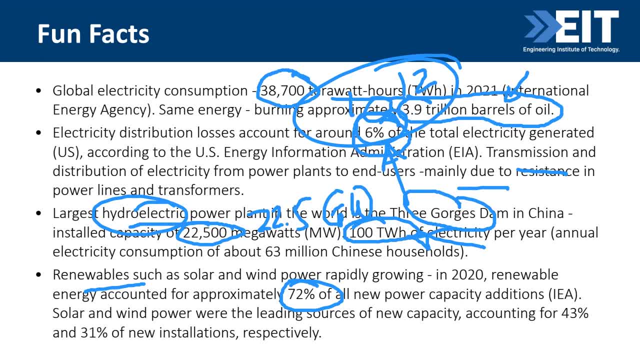 so this is the big baby on the block, the big one that's going to blow us away solar and wind. that's growing fast. so that's always good to see. there's one problem with thanks, Rahul. thank you very much. one issue with solar and wind, obviously. 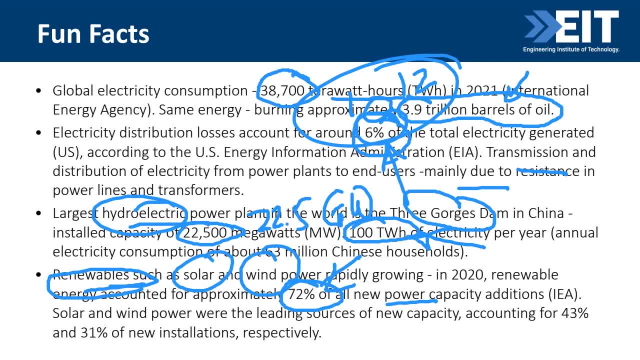 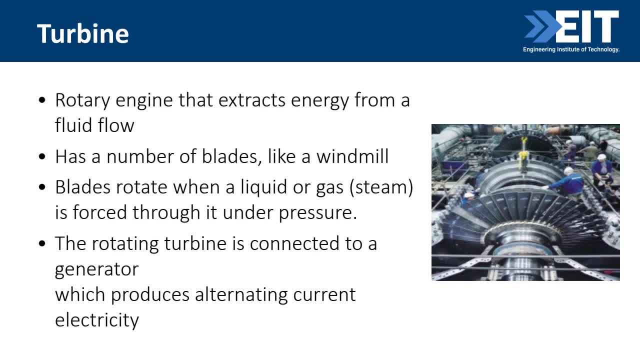 and I'm sure someone will be complaining shortly. it's not a base load. in other words, it's not like a coal station going. it actually goes up and down depending on whether there's wind or light or sun. dear sun, please shine on my, my panel today. 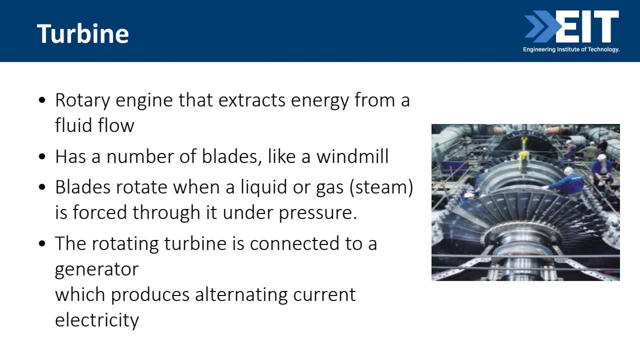 so turbines are a critical part. and that extracts energy from the fluid flow. so fluid flow could be water or gas, or indeed steam, so you could have any of those. so it has light. so that's the critical driver for our, our energy creation. and then you have a electrical generator. 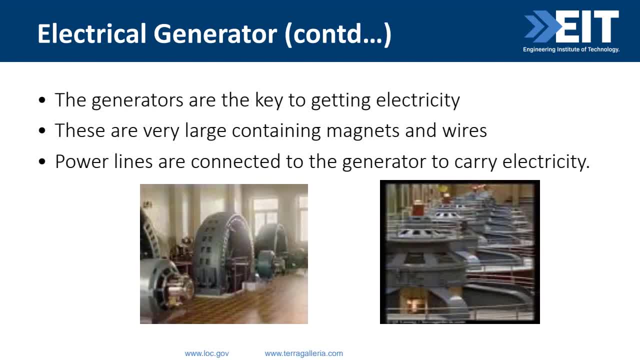 which you'll see here. these are just the two of them. these are just the two of them, generators, and this is there's a little diagram here which I'll show you. here's a diagram for a generator. so this is obviously one of the critical builders we've got. 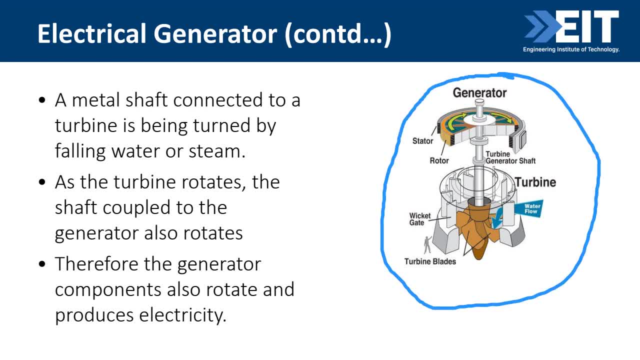 water flow coming through, you've got a shaft going up. and you've got water flow coming through, you've got a shaft going up and, of course, you've got a stator and a rotor. these are the two terms you often hear used in a generator or indeed a motor. 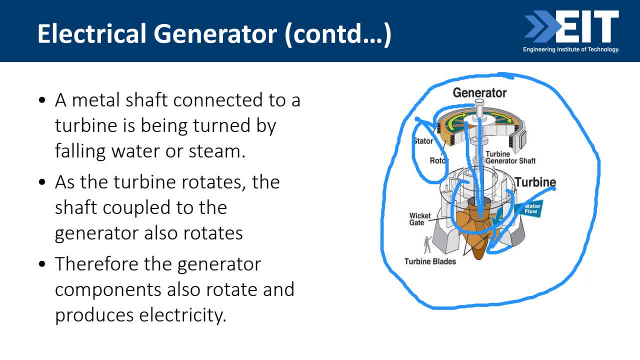 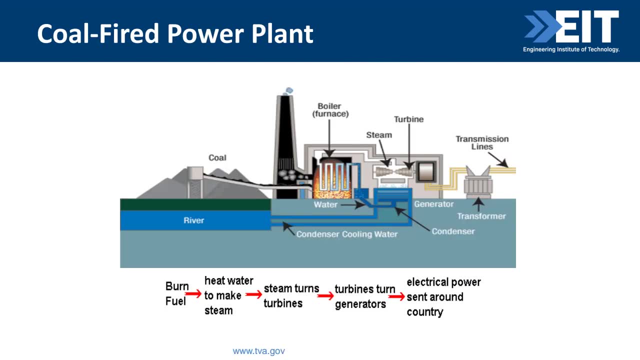 and then you've got a generator and that generates electrical energy because it's rotating around and around and it could also be water, gas, steam, etc. so this is the critical driver for creating of energy. and here's a coal-fired power plant and unfortunately this is very bad. 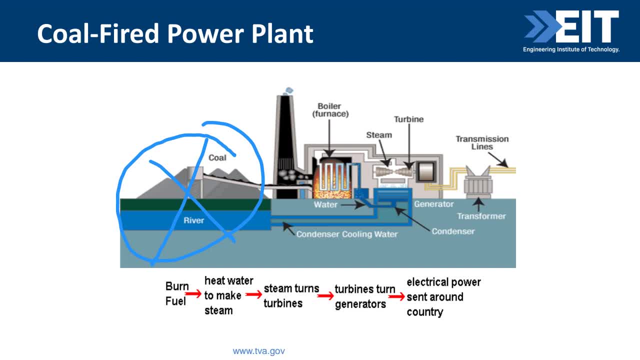 because obviously lots of pollution coming out of here. so this is bad news, so that's why we wanted to talk about this. so this is bad news, so that's why we wanted to talk about this. so this is bad news, so that's why we wanted to talk about this. 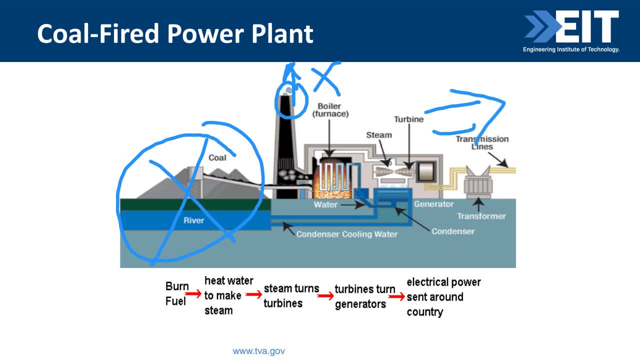 we want to send you the, so that's why we wanted to say that's a bad news. so that's why we want to try and move to something a bit more sensible, because you've got again. you've got your steam coming through here, so you've got. 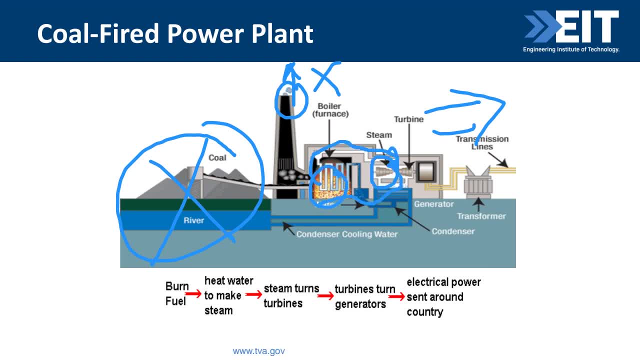 a boiler, a paper, 있어 steam and turbine, and then of course, that's a bad news. so that's a bad news, so that's why we want to try and move transmission lines, and this is where you get transmission, and this is where you get transmission, and then eventually you get. 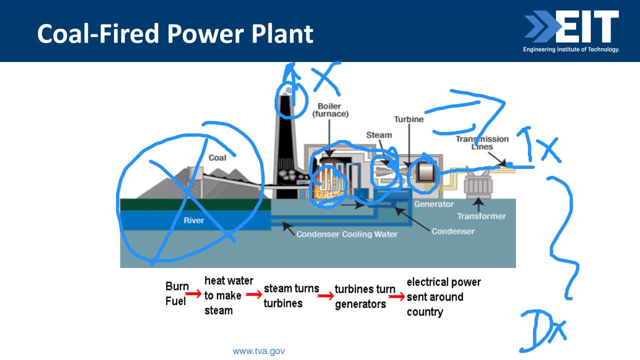 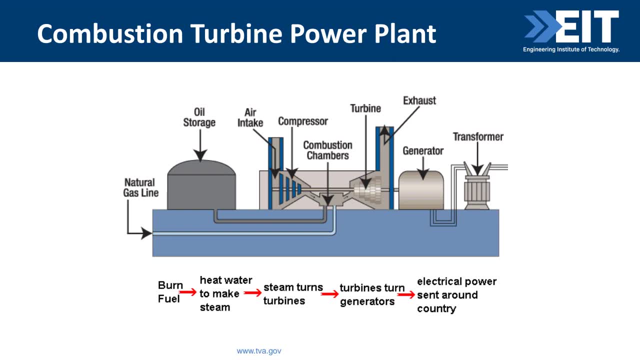 theiqua lights as well. uh, here's a uh turbine power plant and and can anyone ask? can I ask anyone out? um, can anyone ask? can I ask anyone out there what is the advantage of power plants? what is the advantage of a gas turbine? what's the advantage of a gas turbine? so here's your gas. 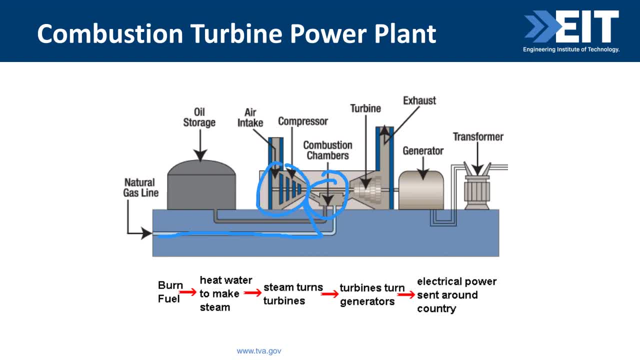 turbine combustion chamber and, of course, you've got exhaust and you've got again energy generated. hello, better efficiency. uh yeah, 50 of emissions of coal. yep, yep, yep. what's the other big advantage? it could be cheap. if you've got cheap gas, yep. if you've got expensive gas can be very expensive. 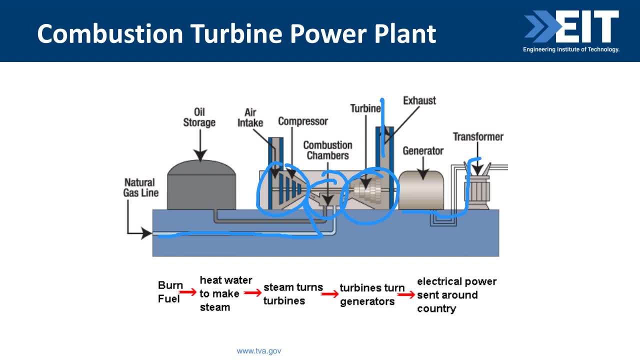 um, the other thing is: yeah, it's dependable. um, the problem is with gas turbines is it can be very expensive to maintain, but they are very quick. boom, you've got no energy. you push the button and you've got energy boom. whereas with a coal power power station it's a long, drawn-out process. 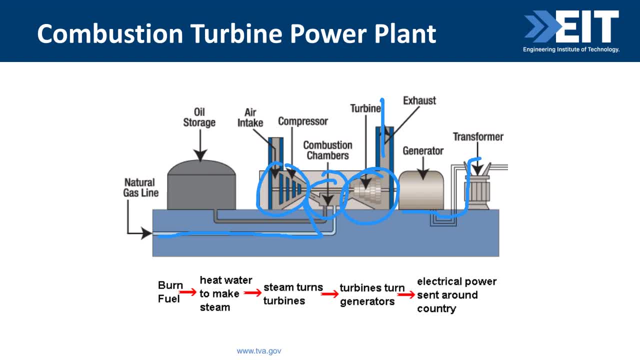 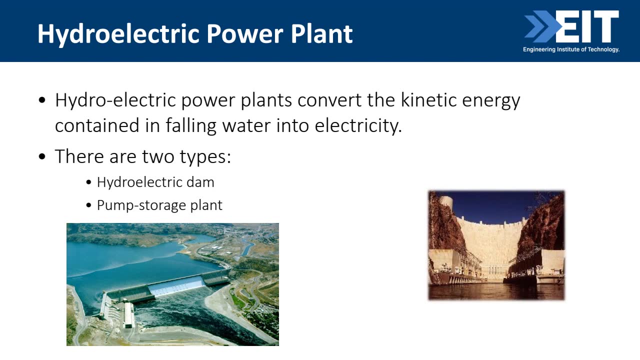 so it's a huge process. quick start. thank you very much, moses. quick start, absolutely right, thank you. so. thanks very much everyone for being so interactive. you, you out there, are teaching me, thank you very much. okay so hydroelectric power plants um two types: pump storage and um obviously. 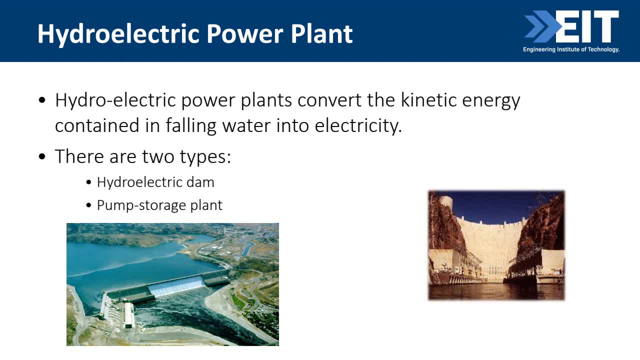 the usual traditional hydroelectric. so in australia, in tasmania, um, we have a lot of hydroelectric power plants in australia. we have a lot of hydroelectric power plants in australia, mania. so here's australia, there's tasmania and there we've got a lots of hydroelectric plants. 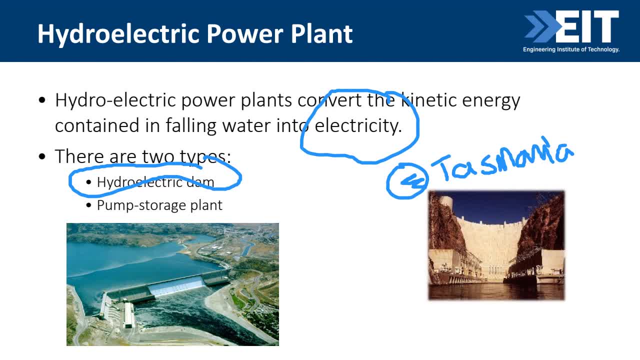 what's the problem from the greenies point of view? what's the problem with the hydroelectric plant, can you tell me? i mean, hydroelectric plants to me are a no-brainer, it's clean energy, it's from the thing. why do greenies not like, yeah, flooding, you destroy. a whole towns you destroy. 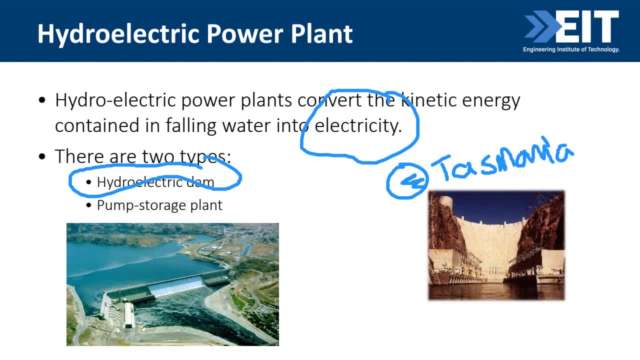 beautiful wildernesses, so people obviously aren't always so enthusiastic about them. land use and absolutely- and you do get thanks- takes lots of land. fish migration, absolutely, you destroy all the traditional things, and what is better than the natural world? please, i'll ask you what is better. 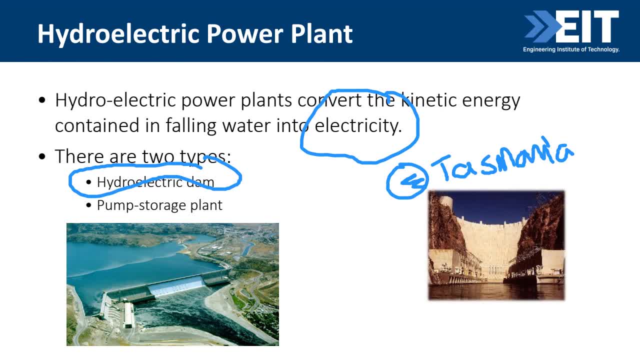 than the natural world, walking amongst the trees, the forests, little rivers running through. it is beautiful. we don't want to destroy that, but anyway it's population displacement. thank you so much, everyone. um less water, no energy? yes, absolutely, and roniel's hit a very good point. 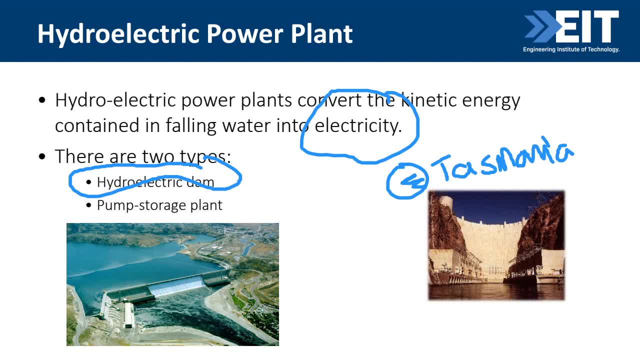 new zealand had a huge problem a few years ago. they depend on a lot of hydroelectric schemes and suddenly drought. no more power, mate. sorry. no power, what the hell, gee? that's incredible. so you know we've got to be wary that that everything we have is got an issue. 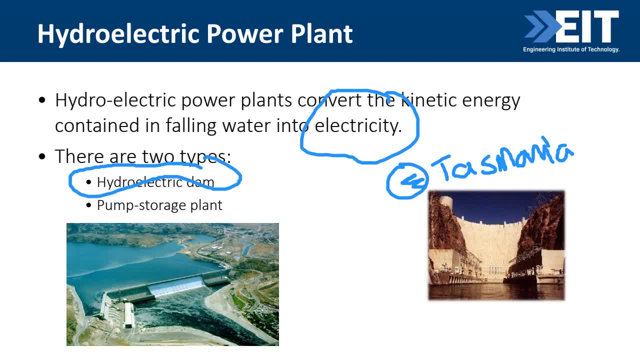 there's no free lunch in life, um, and then obviously, pump storage plants are quite useful, because, um, in south africa, for example, pump storage plants are quite useful. you've got a lot of storage and you can pump the water up and then it's like a big battery. so it's quite 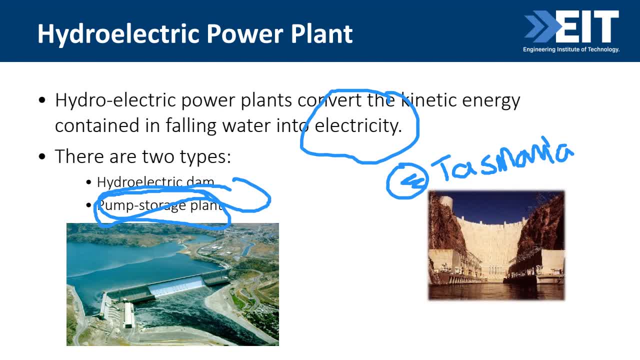 a good idea and you can then when, when electricity is cheap, you can pump it up, the water up into the top, and then when it's expensive or you desperately need it, or peak usage, you can then let it run. so it's quite useful and pete says it's a balance between the natural world and unnatural humans. 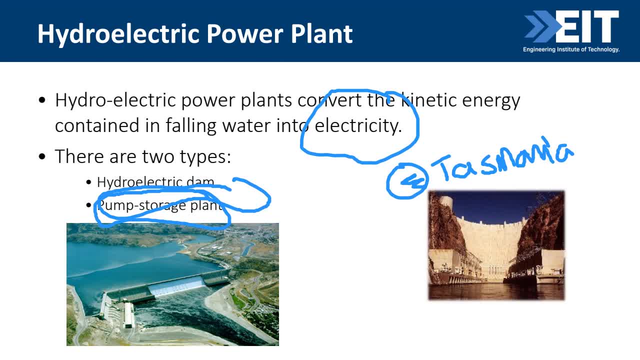 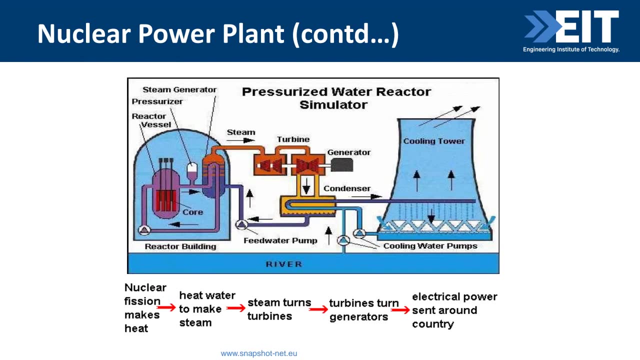 living in it. yeah, pete, you've got a very- it's a very tough view on life, but yeah, i suppose um, having no humans is probably a good thing for the environment, but let's not go down that way. the effect on aquatic life is also very damaging for hydroelectric schemes. thank you very much, guys. 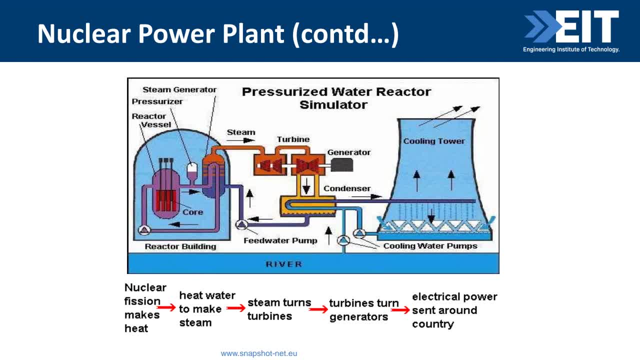 and ladies. so the nuclear power plant is another interesting one, and, um, i just want to say, look, the minute that i open my mouth and say nuclear power is good, i will get shouted down. please do shut up. no bad news. but please, i want to beg you, look at it intelligently. nuclear power can actually 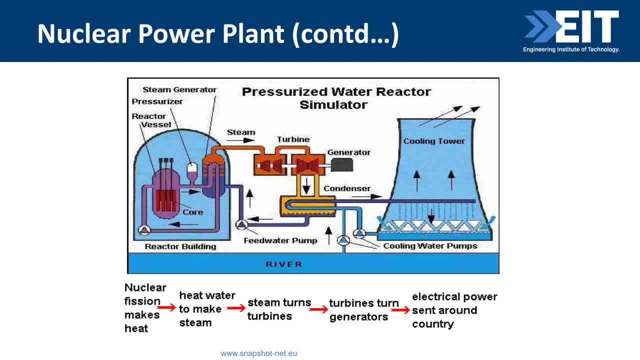 offer some opportunities. obviously you don't want a churnable situation where the whole place is leaking radioactivity. that is an absolute catastrophe. but the good thing about nuclear power is: what is the good thing about nuclear power compared to renewables? high amount of energy, absolutely right. and again you've got your. 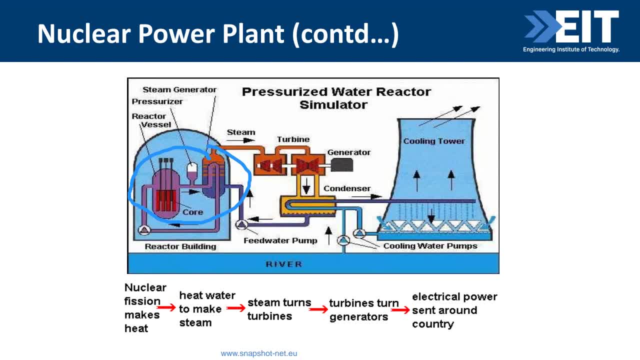 turbines long lasting- yeah, 25 years maybe. constant output, absolutely, as nicholas muschietti says, constant output. it gives you a nice, solid, something which we really do need today, a base load, so that is really important. and clean energy, yeah, well, let's not dwell on. uh. thanks, uh, suman. yeah, let's. 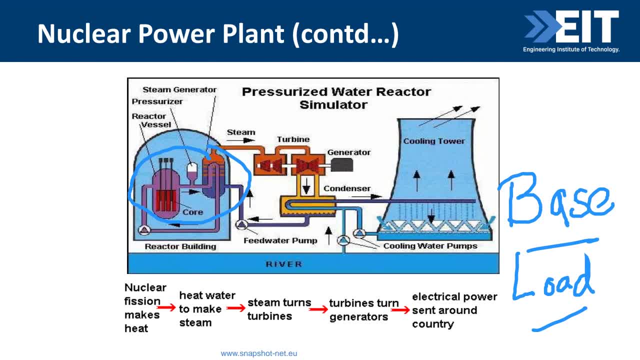 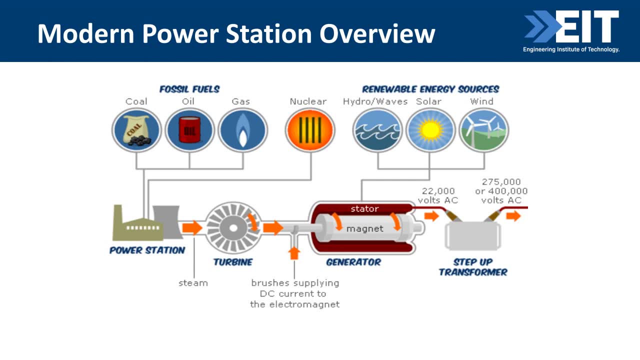 not dwell on clean energy. there will be some kickback there, but it does have some real opportunity, especially nuclear energy. today there's some really clean alternatives. obviously a fukushima built, um, you know, in the 50s or 60s in japan is bad, bad news and that precipitated a whole catastrophe. 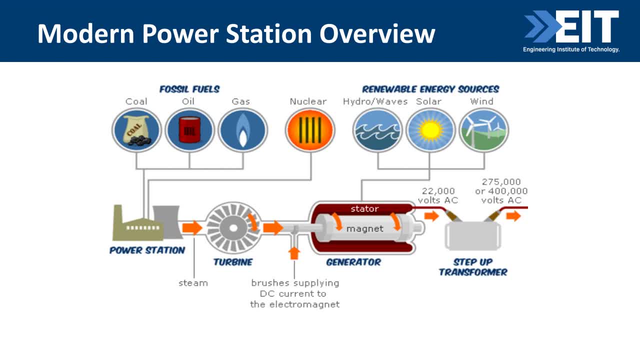 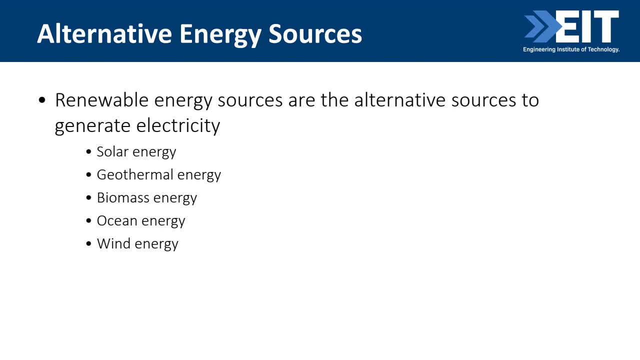 that's why the germans said: look, we've had enough, we're not having any more nuclear power, so it does have. there are issues, so let's just talk about alternative energy sources. uh thanks, high energy, please, everyone. i want to urge you, please look at the chats going on if you can't see chats. it's really important. chats, chats, chats. 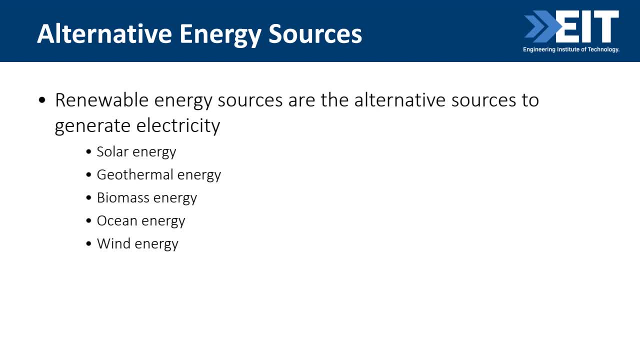 i'll just put a little thing there: chats, chats, the chats are fantastic. they're very powerful. you will learn a lot from people making comments there. i don't have all the answers. in fact, you out there know far more than i do, so please look at the chats. most of them are very, very good. if 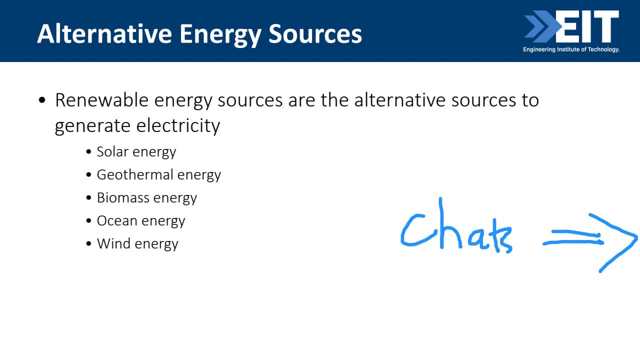 i find anyone that's not chatting properly, i'll make a comment, but they all look very, very knowledgeable. i'm learning a lot as well, by the way. so the solar, obviously the um. we've got a whole lot of opportunities here with solar energy and wind energy. those are the big ones, um, ocean energy not, has been a little. 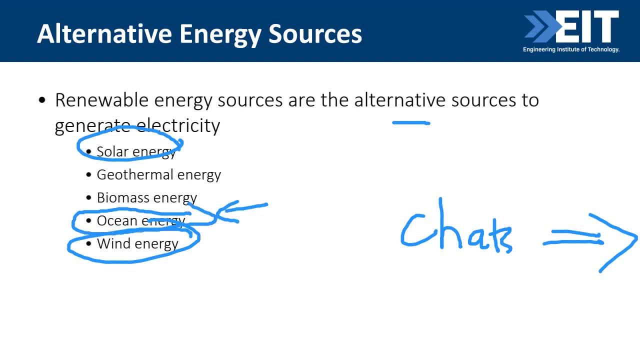 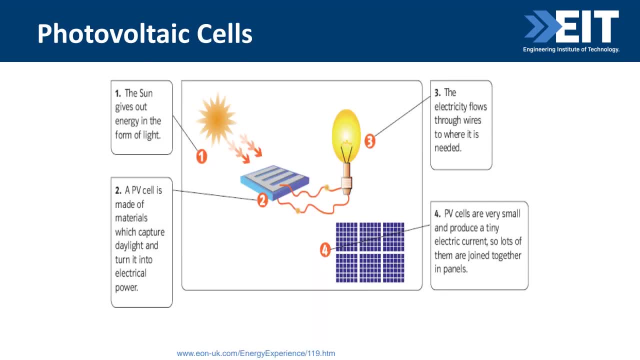 bit tricky, like tides, um very damaging on equipment, but certainly wind. so solar energy um is very simply very powerful and i've got a few statistics here in a tick. but obviously you have energy from the sun hitting that and then you get energy there and your electricity flows to. 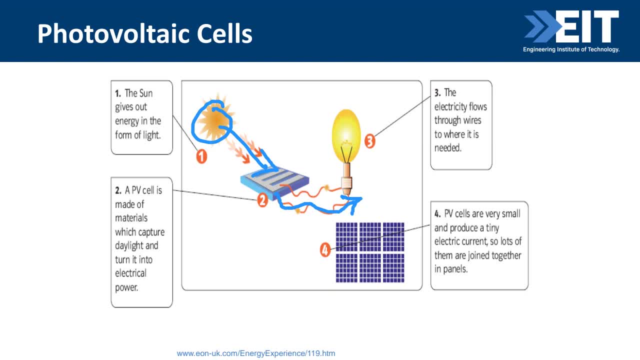 where it's needed and very small and away you go. one of the biggest problems when you put solar panels on your roof. i'm not sure if many people are aware. can you tell me what the biggest challenge is when i say you're getting a certain amount of energy from your solar panel? 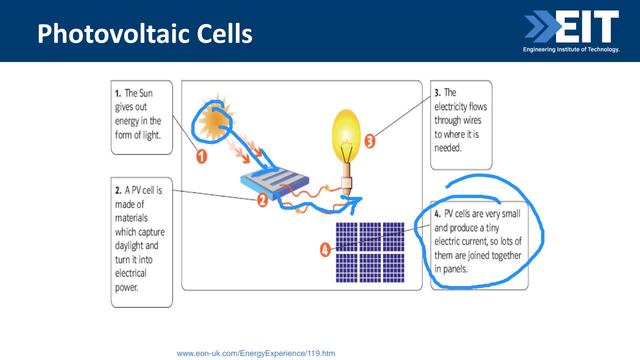 space? yep, definitely space. you take a lot of space, so you need to make sure that the structural engineer does an assessment of your roof. if you've got an office building and got lots of panels- because- and please, i beg you, don't make the mistake we made where the guys putting the panels 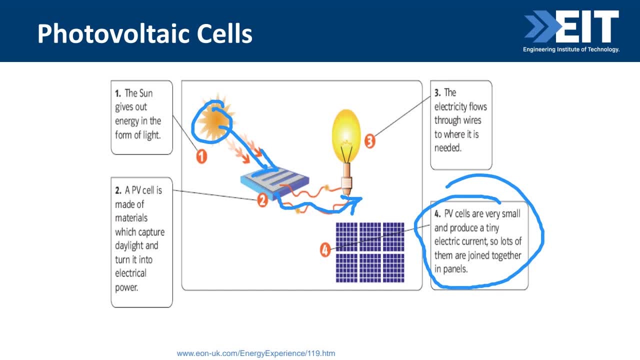 on the roof made nice holes through the roof which then punched at the roof, which we meant when we had rain, we had rain and water everywhere around the office. um, roof orientation is important. yes, vibration effects. no shading on the panels. no one's mentioning this. actually impact on the hd. 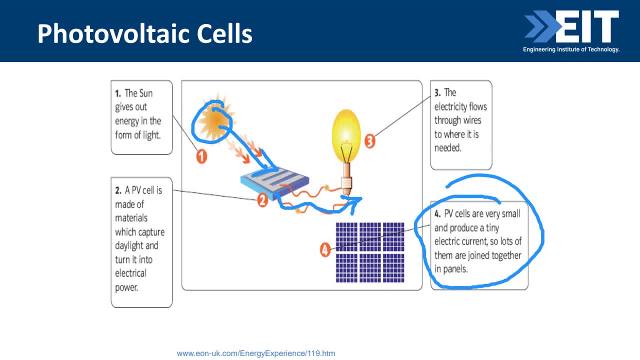 yeah, impact on the lv network. that's really important. one of the biggest challenges is the voltages are rising so we can't put. get everyone to put in there correct direction is really important. no one's mentioned why would i lose? i'll give you a clue: i don't think anyone's. 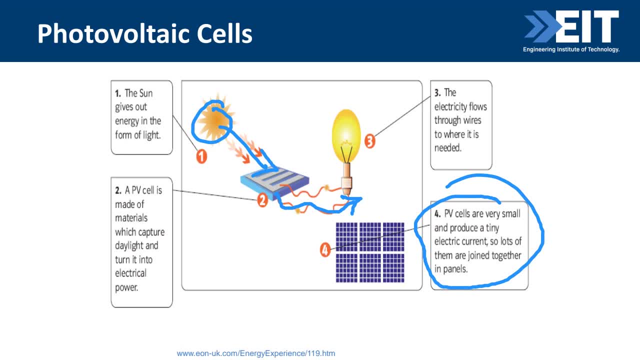 mentioned it. everyone's putting there: recycling is a big issue. um, from the time you put your panel in and you look back a year later, why has the power dropped by 10 or 15 or 20 percent dust? thank you very much for cash. absolutely right, you need to maintain them. so if you think, 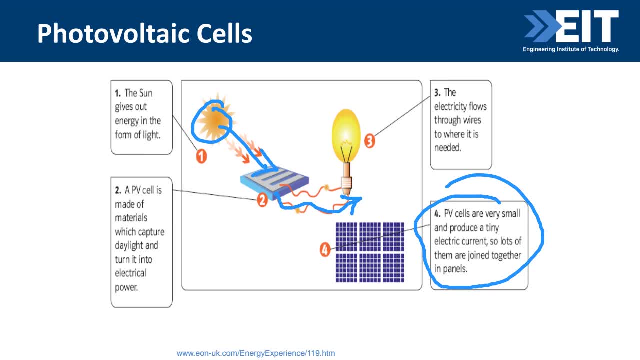 you're going to get so much power every year, you in for a bad, bad surprise, because you get dust and rubbish building up on it. you need to go clean it. please watch out, and faulting is a must: go away. it's a must go if you're not sure, and you're not sure if you can't, could you get? 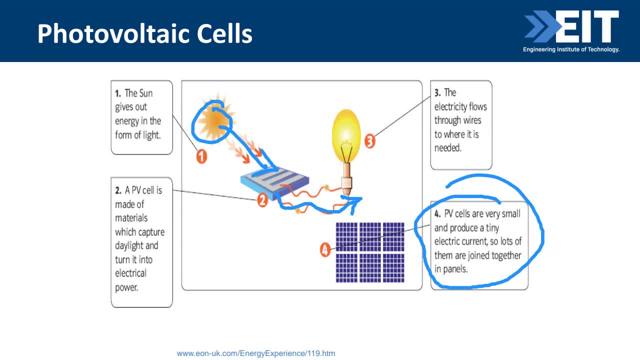 something done and put it back there and verify that you can't. and there's something wrong with the panel. so if you put it on the floor, the panel would be a mess, and so if you need to go clean, then if you don't do that, it you're not going to get a good result, so i'm going to put this aside. 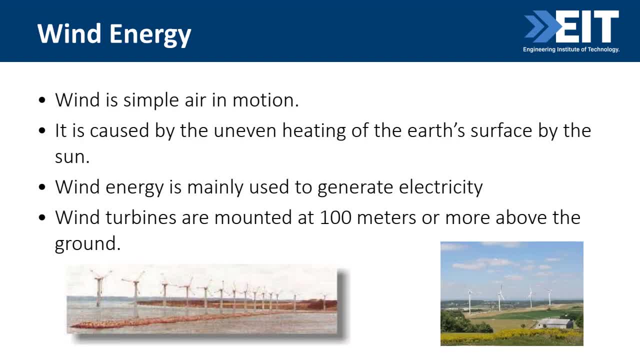 so the next one is a roof connection. okay, it's a good idea to, once you have the roof, немножко of a roof, you're going to have a roof that's fixed up again so you can say: no one's touching the roof, don't say anything, don't tell anyone, and then you can, then you're. 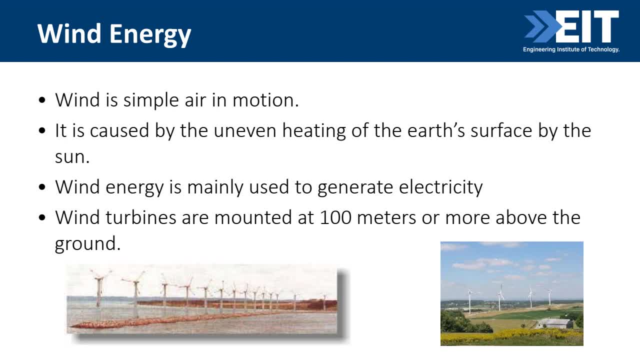 the roof you're trying to do something up and then you've got to come back to it and everything works. put auto wiper and spray for cleaning. yes, you've got to clean, clean, clean, clean. if you don't clean your solar panels, you'll be disappointed. so wind energy, interesting enough, has 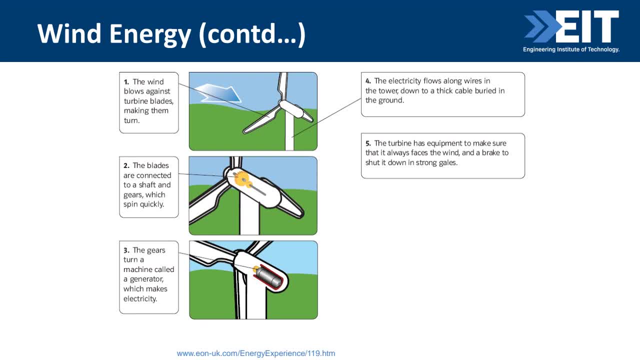 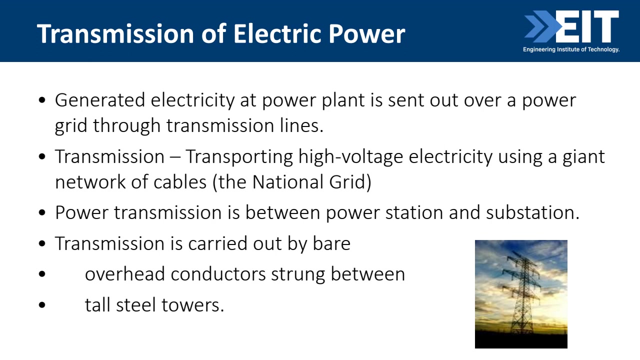 a as a v, the volt, the velocity cubed is the effect for power. power is proportional, that. so as the velocity goes up, your power goes up dramatically. so it's a very powerful form of receiving energy. um, okay, so now we're going to talk a bit about the transmission of power. so you've got, obviously, 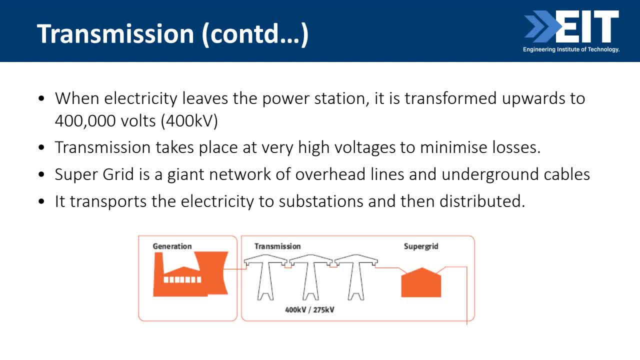 you're going to transmit it up at a higher voltage. now why would you want to run it at 400 kilovolts, for example? in europe? affinity laws- yep, yeah, that's right. no, from pumping, yes, no, you're obviously a mechanical engineer. to avoid losses, why would you uh. 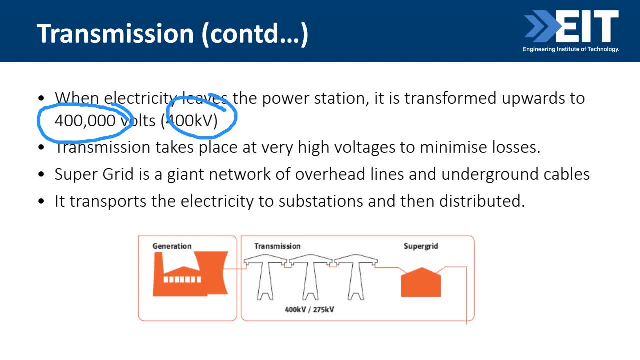 yes, yes, there's some very good comments there. please read the comments are very, very powerful. why would you want to transmit at 400 kilovolts? why not just transmit it thousand volts? size of conductors reduced. yes, yes, as we had commented there. basically, when you have this: 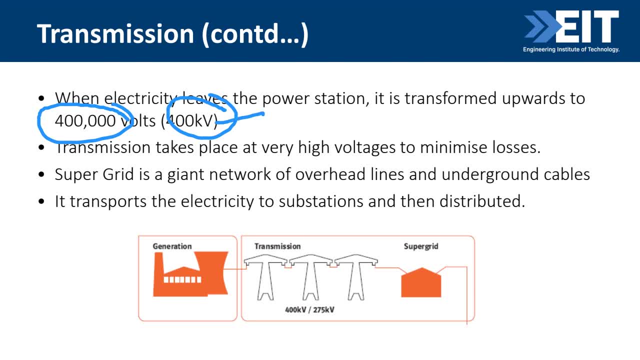 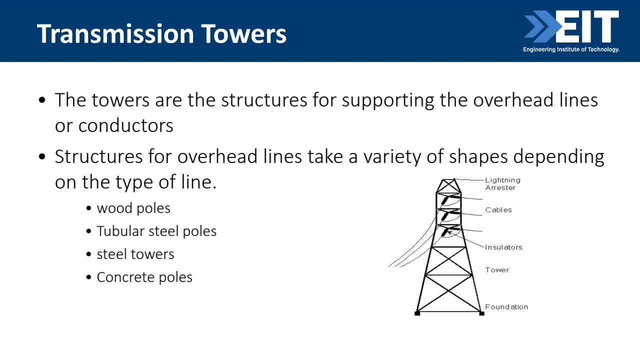 voltage, your current is a lot less, so current is low. once your voltage goes up, your current is very low. so that's really important. owns law. yeah, thanks, greg. thank you very much, absolutely right, so you've got different. uh, transmission towers, uh, lightning arrest at the top cables, insulators tower. 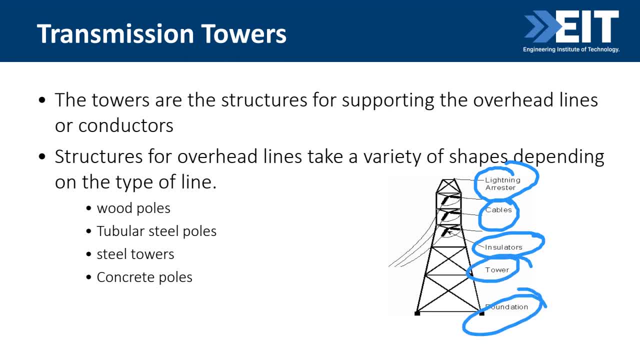 foundation, um, and you could have wooden poles, tubular steel poles, concrete poles, um. why have wooden poles been a problem in western australia and, in fact, in some countries? wooden poles don't have concrete poles in the south east as they are, uh, in southern part of the world. 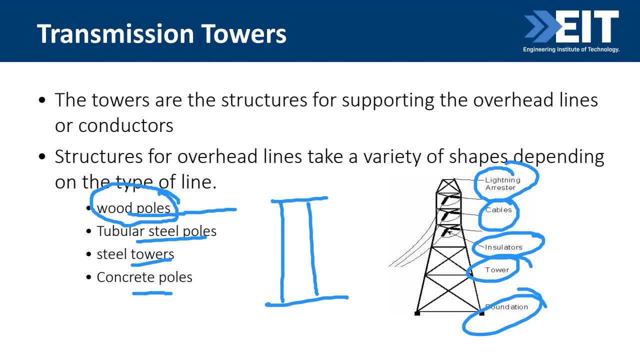 but you've got lots of steel all the way down north. so there's a lot of these things and the problem here is really with this comes from a wind storm from over the south east. we've got three big wind storms. one of them is is blizzard storm, storm fire, storm fire. 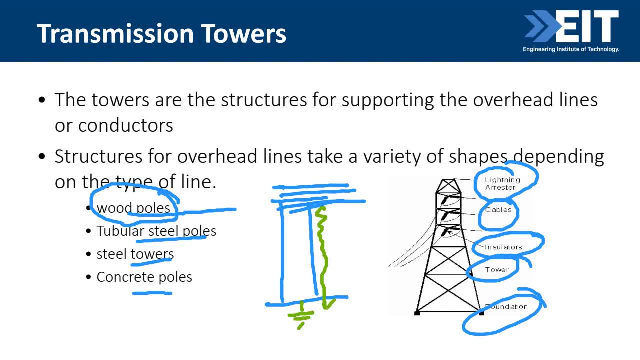 pole, it causes a fire. so electric poles then cause a massive bushfire. so you know it's not um a big, it's not as easy as one thinks. so wooden poles are good and also, um, you can get leakage of current and, as as everyone says, the damage from wear and tears a lot more with wooden poles. 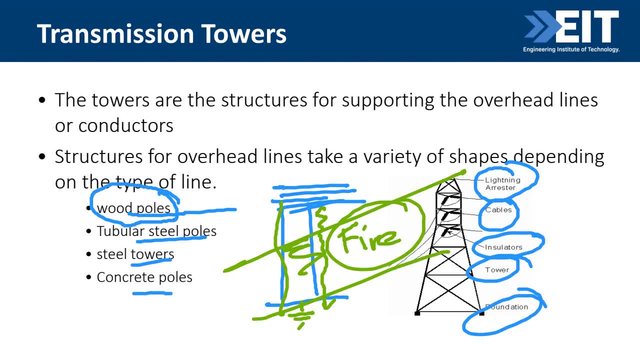 uh, to lower current yep. achieve this the supplies that are high voltage. thanks very much, dr bernushi singh. yep, absolutely right. uh, why wouldn't poles? yeah, so wooden poles are a problem in western australia because not only can they get burnt by bushfire, but they could. 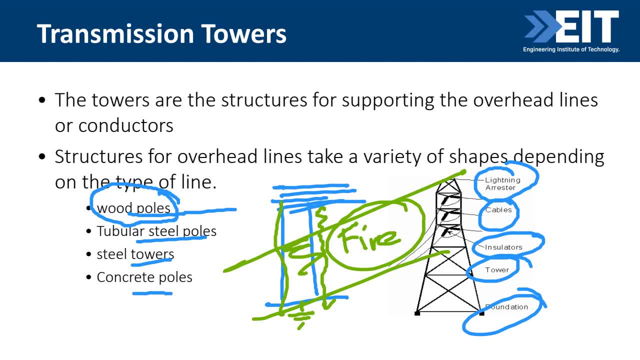 also create a fire. if you get leakage from the um, leakage of current, down through the, from the distribution of the current, from the distribution of the current, from the distribution of the current, and wires here into the ground, they could cause some uh uh fire hazard of the pole itself. 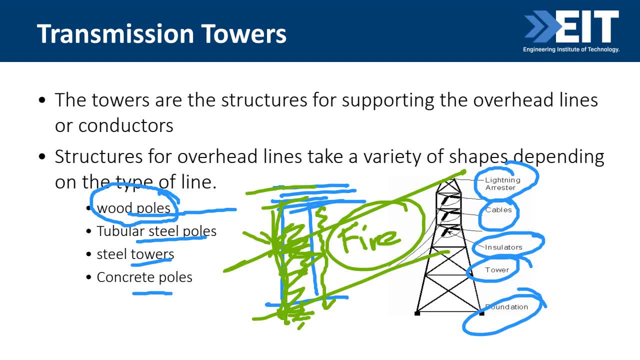 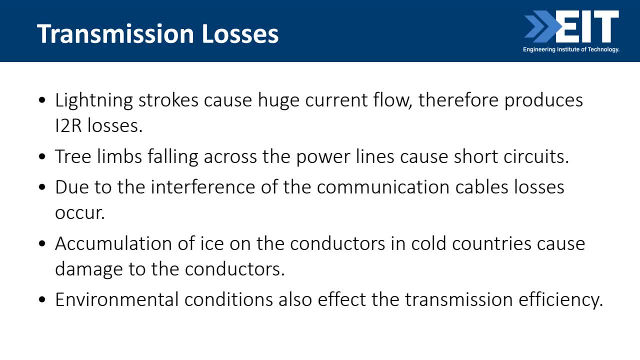 and it could be likely to cause a bushfire. uh, drop there, yep. so. so basically, um, wooden poles are probably not always a good solution. so lightning is another issue, cause huge and produces what they call i squared r losses. that should be i squared r, which basically means um, i squared r. can you want to tell me what i squared r is referring to? 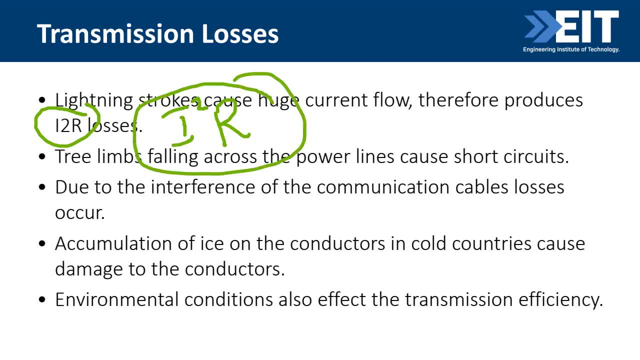 power. thank you very much, nagazi. i've got, i've got a whole team of gurus here and obviously tree limbs can cause problems. uh, interference, communication, accumulation of ice and accumulation of ice can cause problems with conductors in cold countries. what does it do to the conductors? it can pull the whole up down. so obviously those are all big issues. 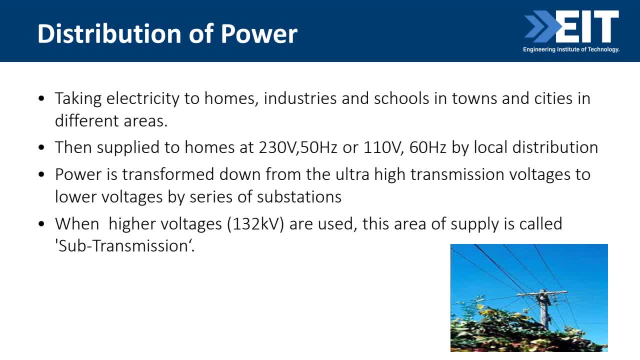 losses. then we've got distribution and we want to distribute at 230 volts in australia or 115 volts, 110 volts in uh, usa, so obviously different voltages, and we will then bring them down. so the voltages i'm going to quote here are probably not. 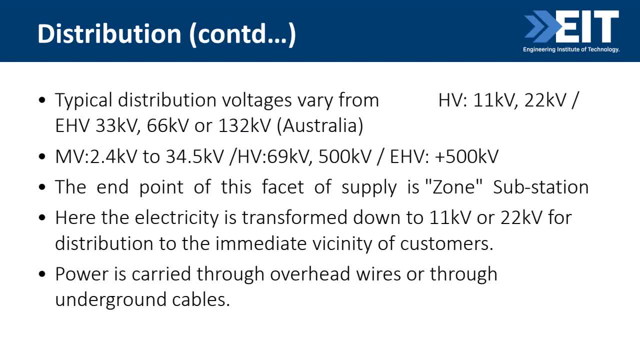 always the usual one. so in australia we would have things like 11 kilovolts. you're here 11 000 volts, 22 000 volts, all the way up to 500 000 volts. in fact, in australia you have 500 000 volts. 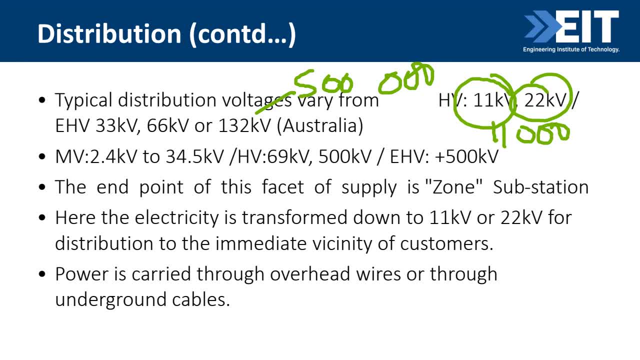 in fact, in australia you have 132 000 volts, 220 000, 275 000, 330 000 and three 500 000 volts, and then the states. we have a thing called medium voltage, high voltage and then extra high voltage, and you've got different. well, that should be usa. can anyone tell me in australia when? 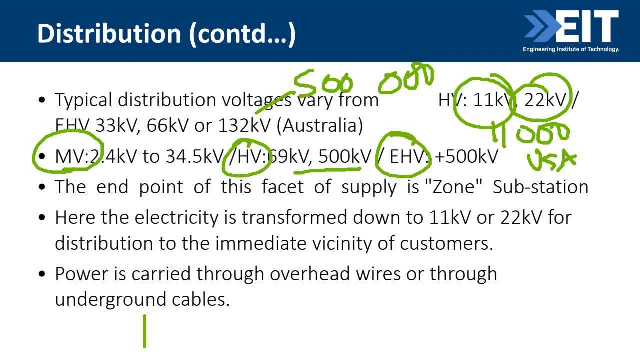 you talk about high voltage and low voltage. what is the gap between the two? 500 volt dc. yep, yep, in fact you can get 500 kilovolt dc volts as well. thank you very much, michael. yeah, thank you very much. so, as michael says, there, up to a thousand volts. low voltage in that. either way, it's 20 volts power and this is being streaming over here dc. there is no power power at the moment, as i mentioned, if you'll leave me at the box for a moment, it's only performance. typically, you're getting higher terms of. 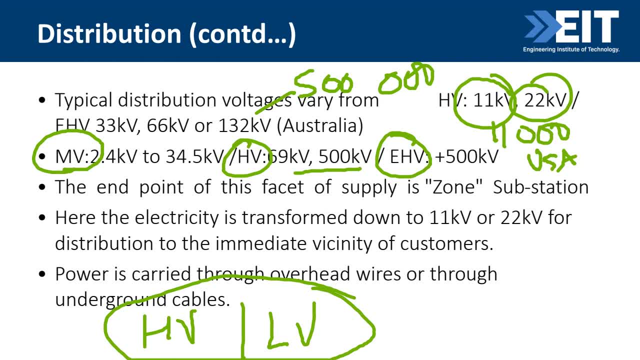 over a thousand volts you've got high voltage. We used to refer to medium voltage. You don't hear that referred to much anymore in Australia And they've tended to avoid the medium voltage refer. They still talk about it but it's really high voltage and low voltage. 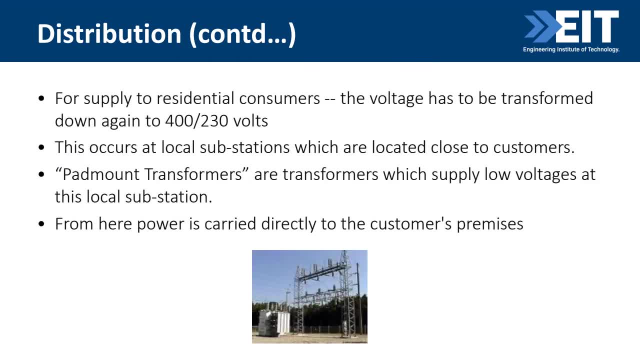 So distribution is the next thing. So we get transmission and then we go down to distribution and we want to bring the voltages down with what we call substations and pad mount transformers. And believe me, getting a substation put in your area can be a long process- two years. 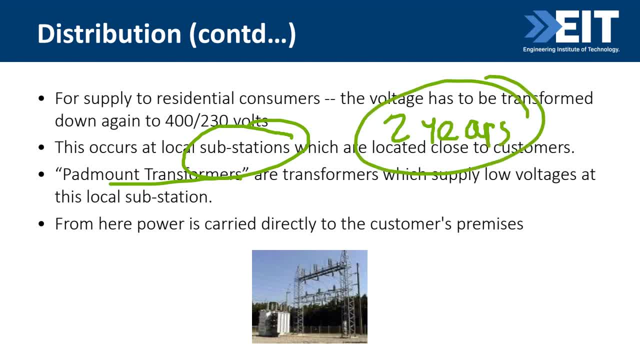 maybe So if you're planning to increase your capacity of your building, you may be very disappointed if you go to the local utility and say, hey, mate, I need more power. I've got 238. Amps at the moment- three phase. I want 400 amps And you may have to wait two years and 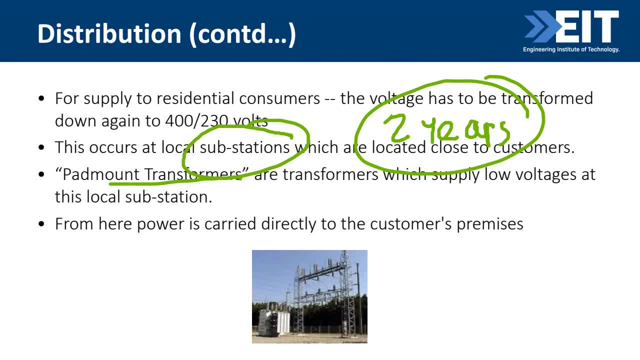 you may have to pay for a substation And they might say you're going to have to find some space on your premises to put the substation. You say ooh. Or they may say, look, mate, we've got no energy in this area so it's not going to happen. So what's the purpose? 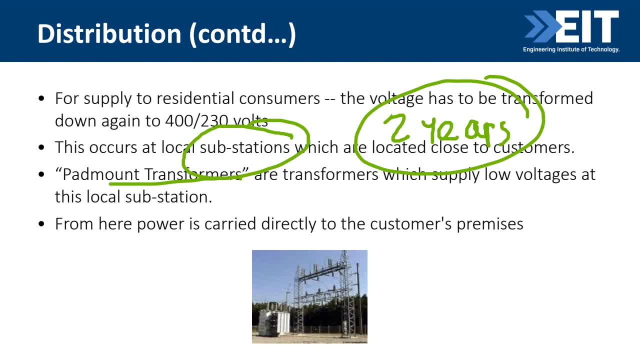 of the substation. Can anyone tell me Why would you have substations? Is it just a waste of time? Set up, Step up, You have transforming. Yeah, so basically, a substation is a way of distributing current in your area- lower voltage, Step up, step down, So you'll always have associated. 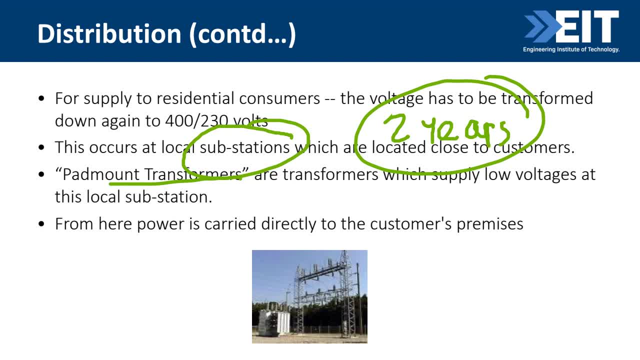 with it transformers High voltage down to low voltage to feed into your premises in Western Australia- 230 volts. Can you tell me what Western Australia used to have as a voltage? How high did they go in the old days, The very old days when you see my grey. 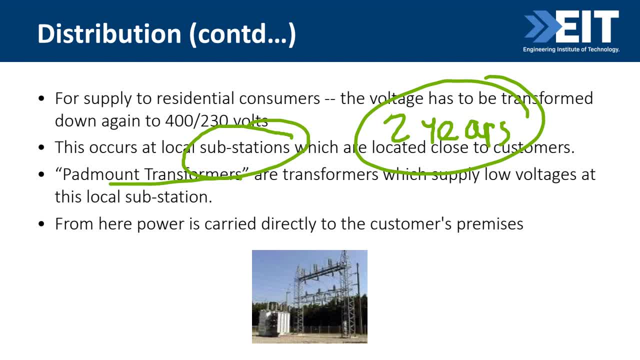 hair. What is the voltage they went up to in Western Australia? Okay, Dr Banishi Singh has got a comment there. Substation designed to accomplish change voltage from one level to another, regulate voltage to compensate for systems. Thank you, Dr Singh. Precise. 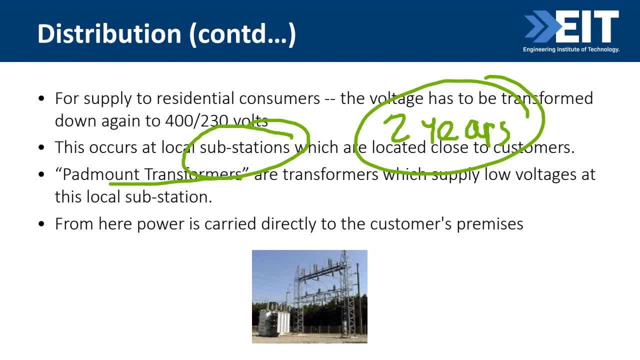 In fact, I should hand the microphone over to you. I think you know a lot more than I do. Yes, Okay, so in Western Australia we actually went up to. we typically run at 230 volts, And 230 volts is a sort of uneasy compromise. A lot of Western Australia was 240 volts. 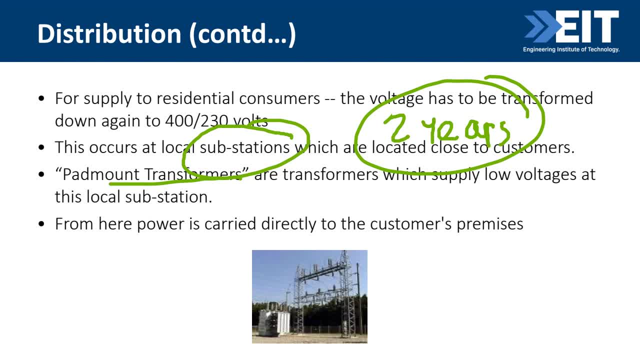 It went up to 250, 260 volts in some of the northern part of Western Australia And a lot of the European standards is 220 volts. So we've now got a nice compromise of 230 volts. Why is everything about? just about Australia? I'm sorry, I'm just living in Australia. 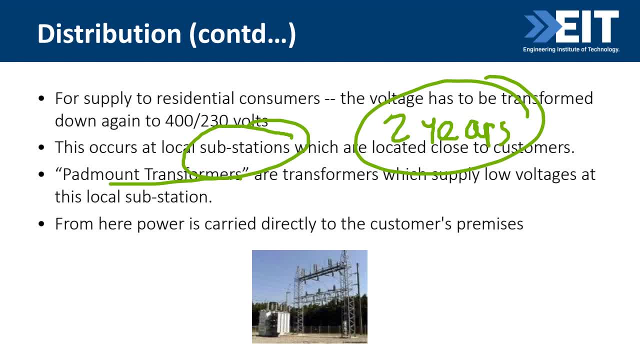 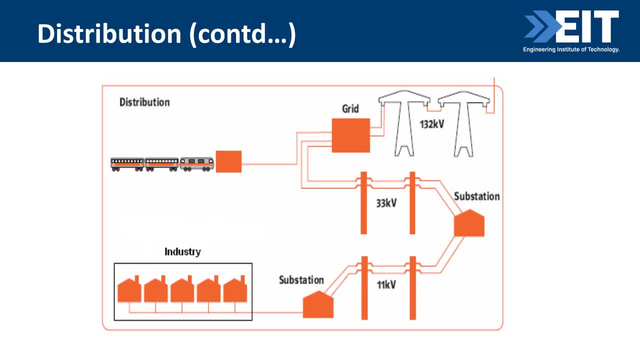 That's why I'm talking about it, But my slides refer to everything. Abhina, Thank you very much. It refers to the whole world. I've got references to everything, So, my apologies, I don't want to be sound Australia-centric, So here's the typical. 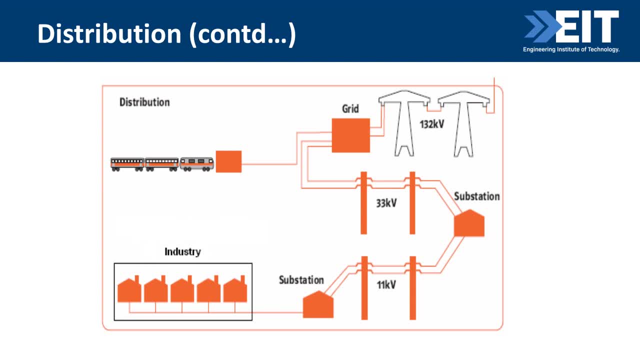 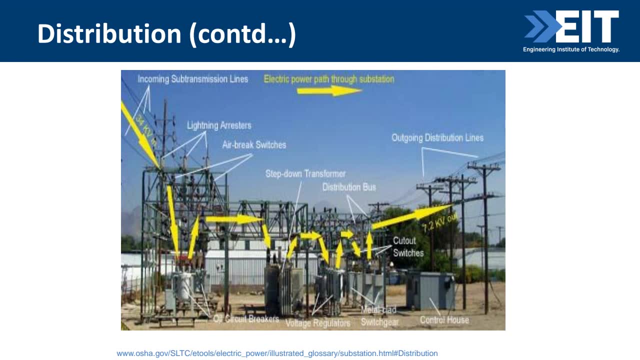 distribution industry, the substation. As Dr Singh says, we will reduce the voltage And here's a typical example of a little incoming sub-distribution lines coming in here, Lightning arresters and, of course, outgoing distribution lines. So we've got sub-transmission. 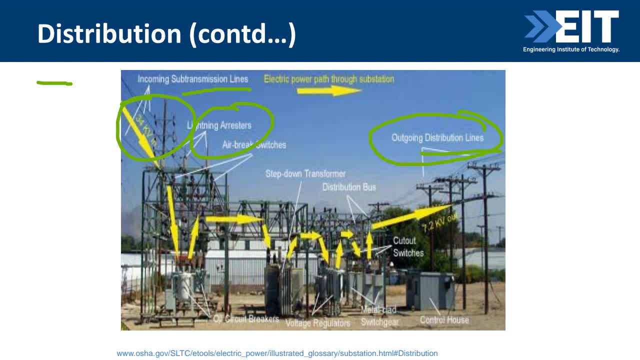 coming in distribution there And before then we've got transmission. Is the splitting of? Okay, so great place to live. Thanks, Michael, I'm sure your heart is where the Yes. so you're splitting the voltages at substation, single phase or three. 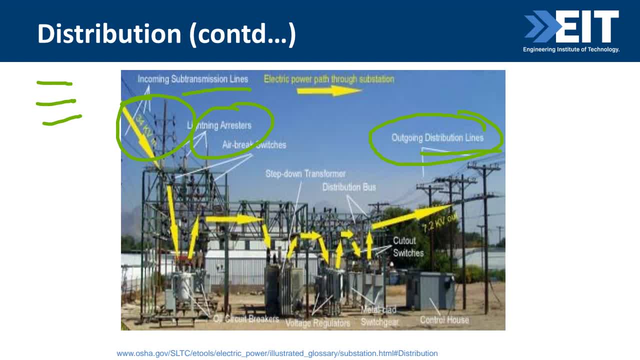 phase. So good question. You can actually run three phase into your building these days. So in the old days we only had single phase, but you often see three phase coming into residential buildings now. So at the street level you'll find the three phase coming in. So good question. So there's. 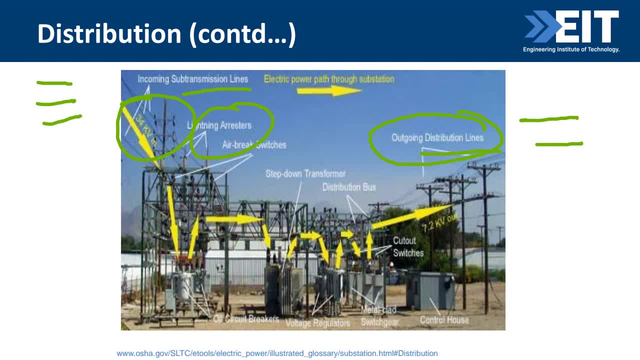 a comment there about three phase. When you're looking at your socket in the wall you'll see single phase, But in fact often you'll see three phase. three phase, which basically refers to a more efficient way of transportation. So if you're working in an industrial setting you'll always have three phase Far easier. 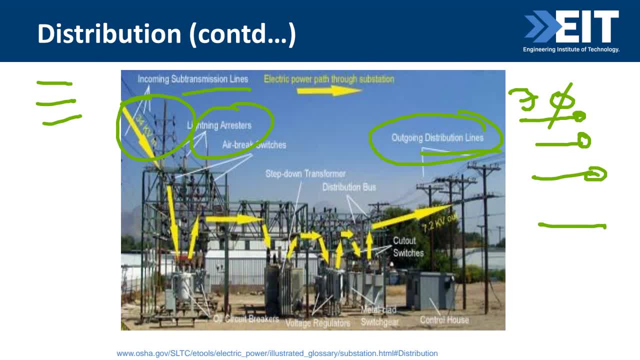 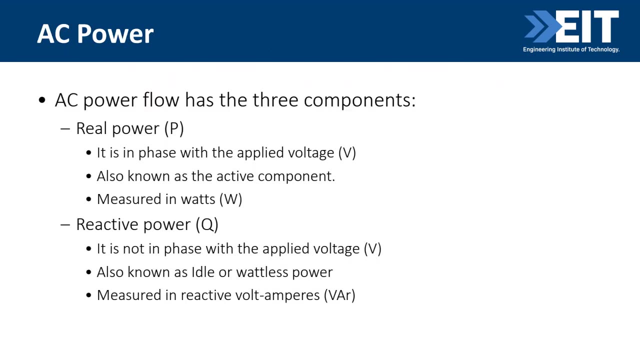 So you'll have a more efficient way of distributing power if it's three phase, three wires, And then you'll hear terms such as delta and star. Okay, so really there's three components to power flow And really I'm not going to go into too much detail on that, But I'm going to go into a 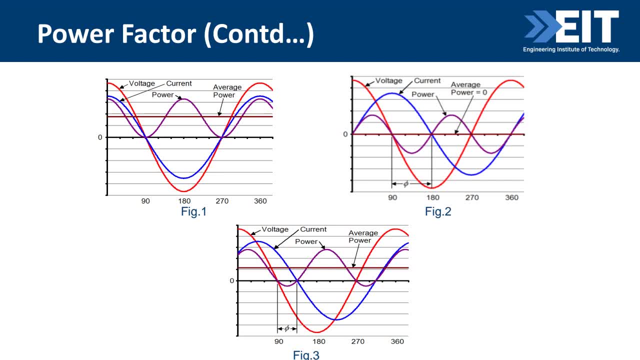 bit more detail on that, But I'm not going to dwell on this. But effectively, you have always a triangle with power flow. You'll always hear terms such as this: S, which is apparent power, Q, which is VARs, which is reactive power associated with capacitors. 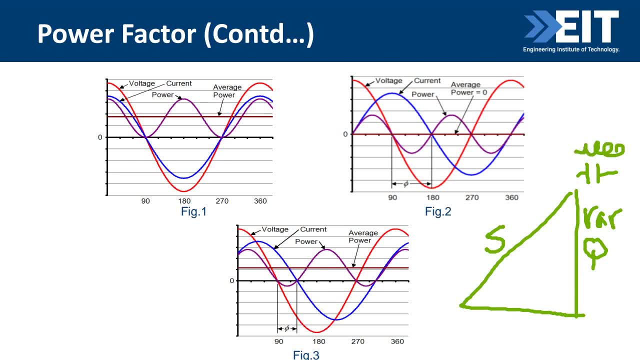 and inductors. And then you have real power, which is associated with resistors And that's in watts And this is in VA. So you'll see all three terms referred to VA for apparent power, Volts, times, amps, VARs. 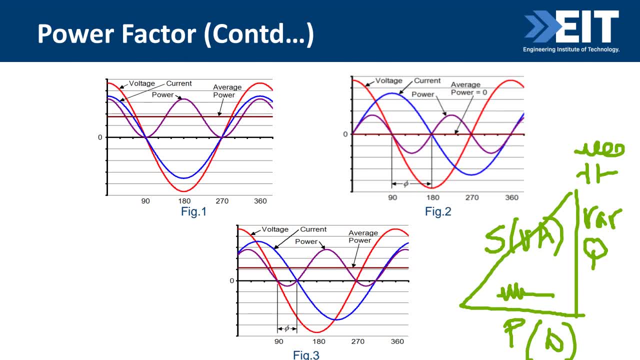 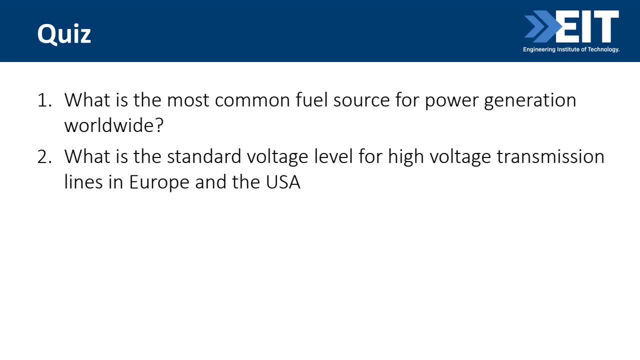 which are associated with capacitors and inductors. So you'll see that, both of those terms. So the question for you is: what's the most common fuel source for power generation worldwide? Yes, Tony thinks is. can we? Yeah, thank you very much, Cole. Absolutely. 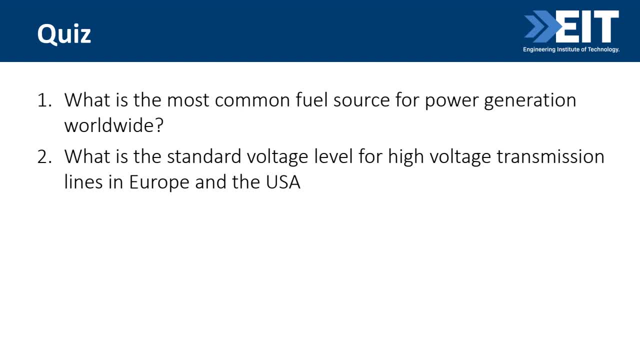 And can I just have a comment from everyone: What are the three color codes for three phase power? Just give me them, Just type them in: Red White, Blue, Red White, Red, Red, Blue, White. Thank you very much. Red blue white. Red blue, white. Red, blue, white. Everyone. 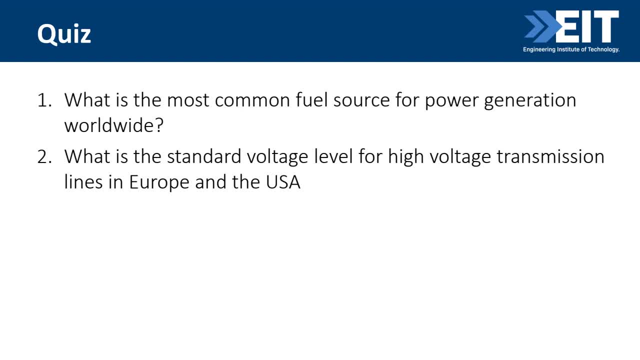 agree with that. Yep, Thank you, Okay, Okay. Okay, That's good. Thank you very much. Okay, So that's the Australian standards. There may be different standards elsewhere: Red, blue, white. Okay, so the most common fuel source and then standard voltages. 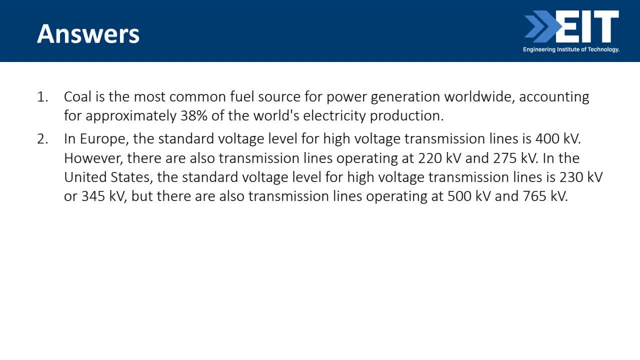 Thanks very much, guys and ladies. So coal is the most common source, unfortunately 38%- And the voltage for Europe is 400 kilovolts, And you get US also different range of voltages as well. So I will clarify all the color codes in a attachment. 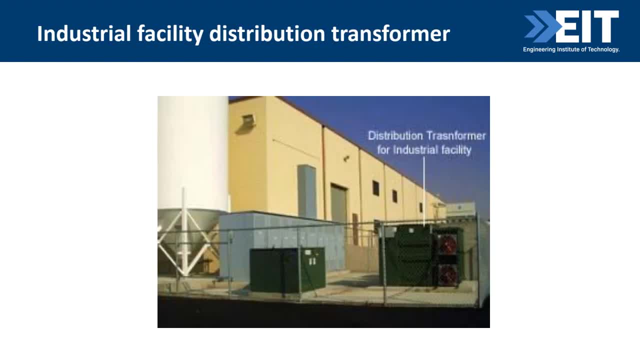 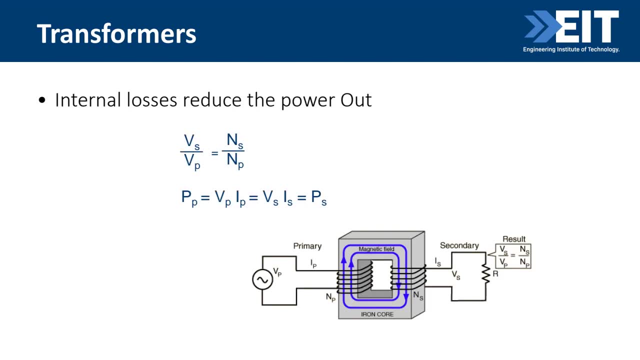 because that is really important. So now I just want to talk about transformers. We spoke briefly about transformers And really what a transformer does is. here's an example of a transformer. This is a key building block of all the engineering stuff that we do. 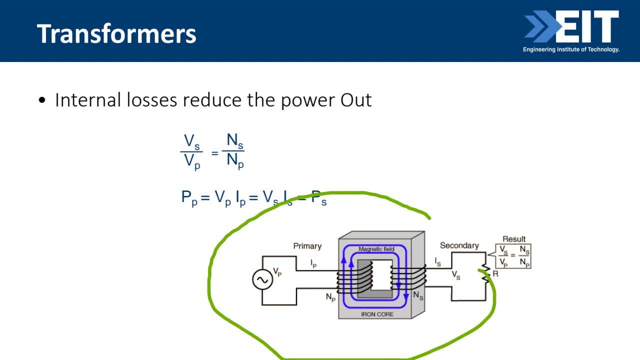 And here you'll see, You've got a coil and you've got voltages, a primary and a secondary, So you can step up, which means the voltage goes up, or you can step down. So this is how you can get 230 volts out. 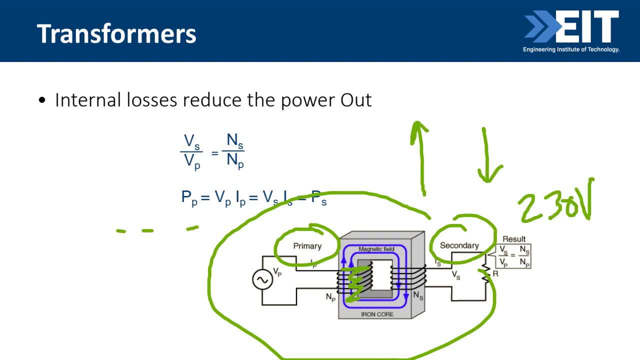 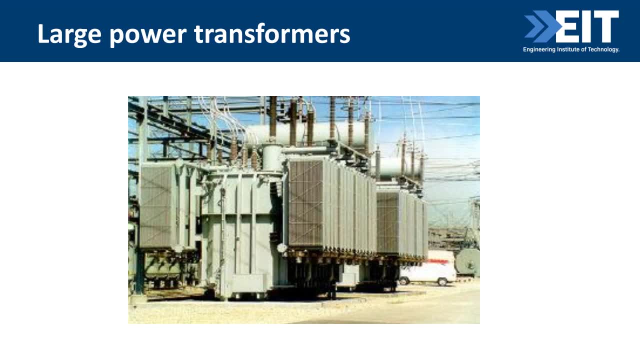 And you can have a higher voltage in. Is it true that if you're colorblind you cannot be an electrical engineer? That's a very good question. I don't know, I wouldn't think so, but certainly that is a A potential problem. 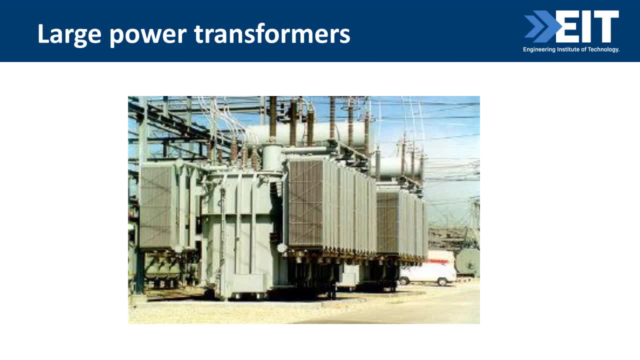 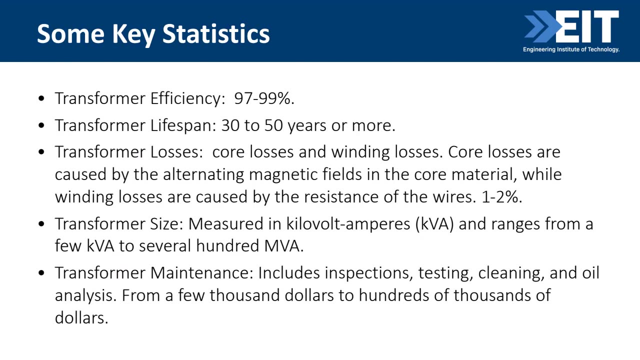 So you'll see the different color codes in the different countries. So rather than Yeah, thanks Michael, Yeah, no, no, that would be discriminatory if you weren't allowed to. So no. so some statistics of transformers: efficiency is very, very high: 97 to 99%. 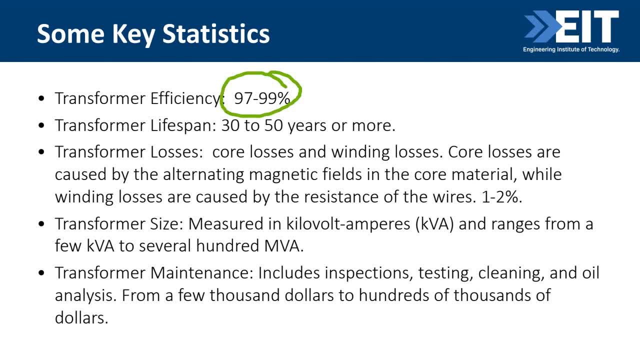 So that means you lose very little energy. You can have them for 30 to 50 years. There's two causes of losses: Core losses- And the size can be is rated in kilovolt amps and ranges from few kilovolt amps to a few hundred megavolt amps. MVA. 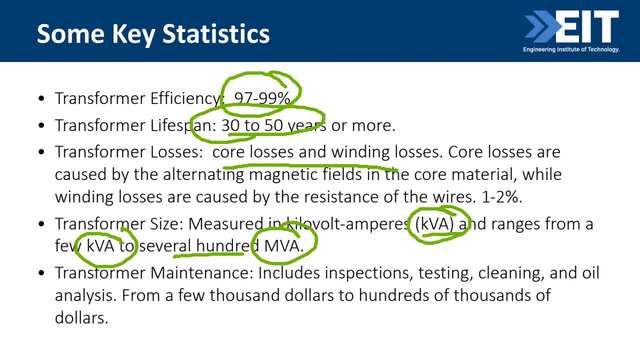 So what I'll do is I'm going to give you the color codes in a separate document, So don't go on anymore. Every country has a specific color code. I am going to give, I'm going to give you the important color codes in an attachment at the end of this session. 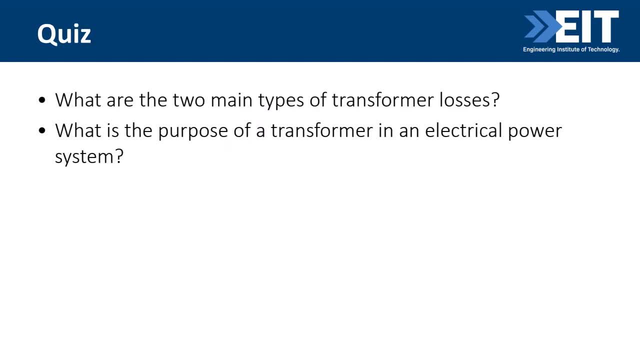 So don't worry, We'll send it out. So two types of transformer losses: Core and winding. Thanks, Scott, Absolutely right. And what's the purpose of a transformer in an electrical power system? Core and winding- Yep, two losses. 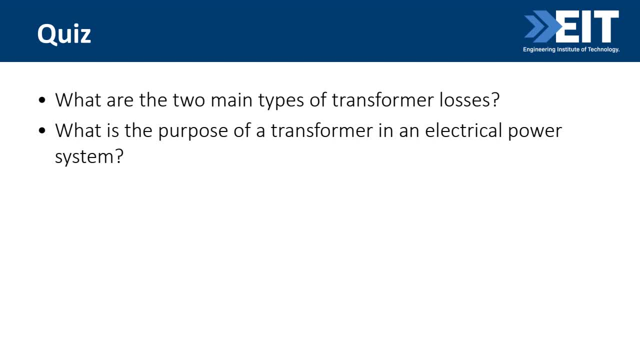 Iron and copper or core and winding, It doesn't matter, Iron and copper. Thanks very much, Alimon. Okay and yeah, iron, Step up, step down, Absolutely. Thank you very much. brilliant, Thank you so much. 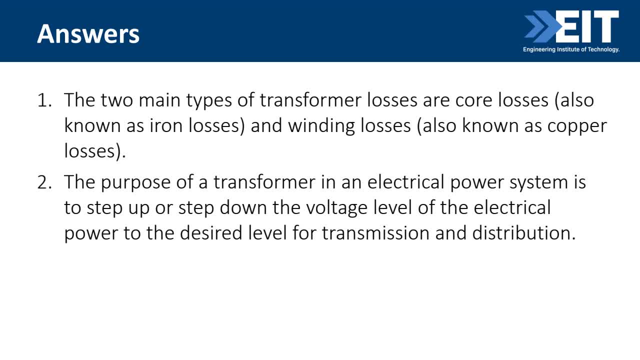 Core losses, And some of you guys offered answered core losses or iron losses. It's because you've got a core. Here's your transformer. So you've got the copper in the cable and you've got the core, the iron, in the piece of metal, the magnetic material. 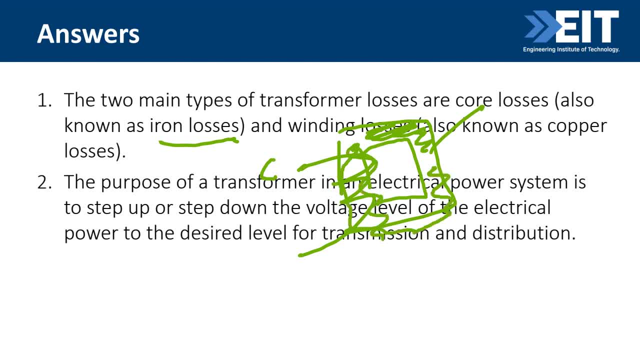 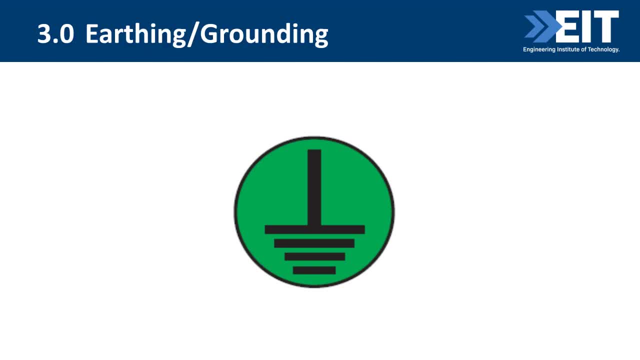 Thank you very much. And obviously, step up, step down. Okay, so the next topic is earthing, grounding, which is why would you have two terms here? by the way, Anyone tell me Why transformers rate in kilovolt amps? 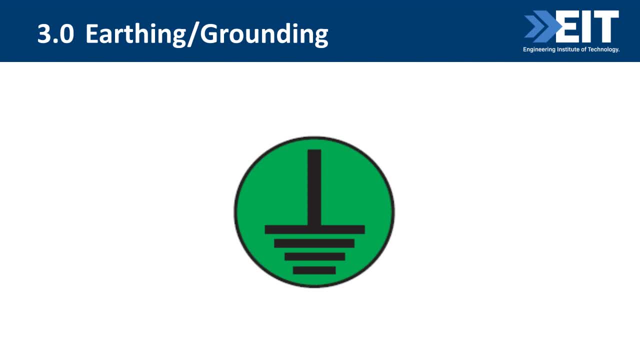 Iron core, Yep, yep, Thanks, safety, Absolutely Earthing, grounding very important. So you'll see the word earthing used typically in Europe and Australia, Africa, and you'll hear the word term grounding used in um North America: the I triple E, I triple E total losses. 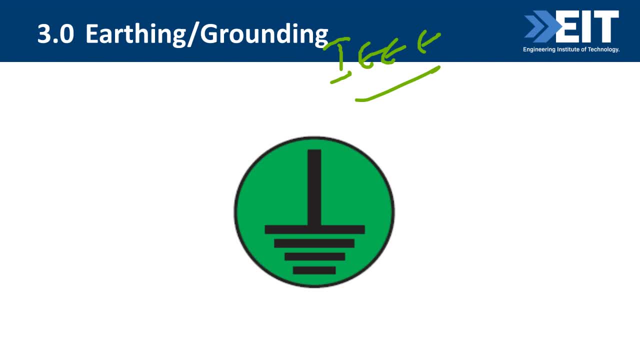 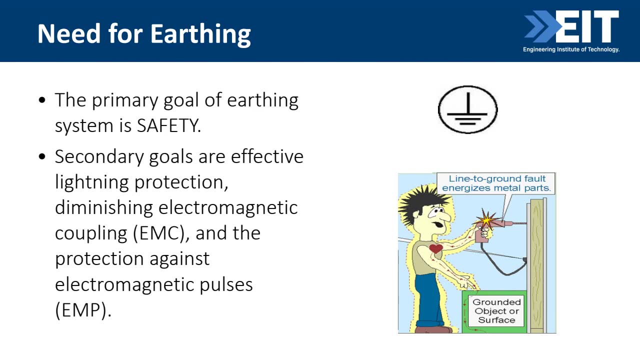 Yep, Thanks very much. Look, I would love to go into more detail on everything, Believe me. So the big thing about earthing is, um, obviously safety, So that's really important: Safety, safety, safety and obviously lighting protection and protection against electromagnetic. 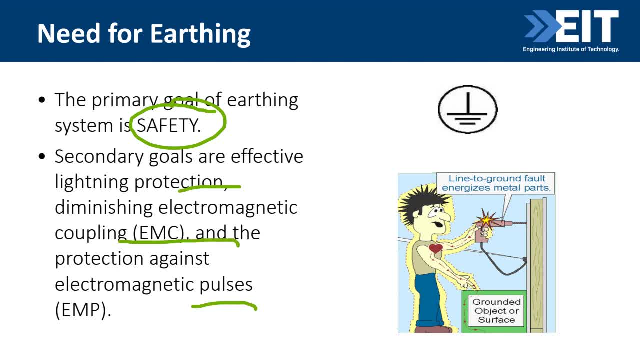 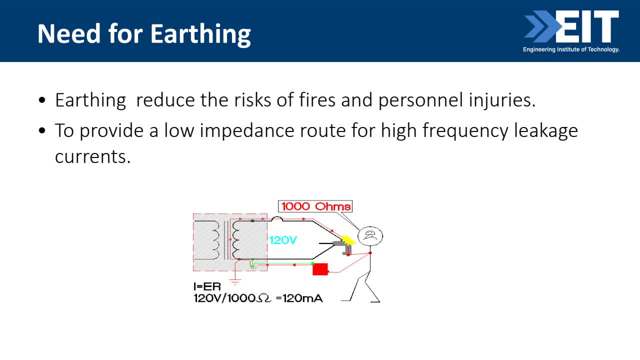 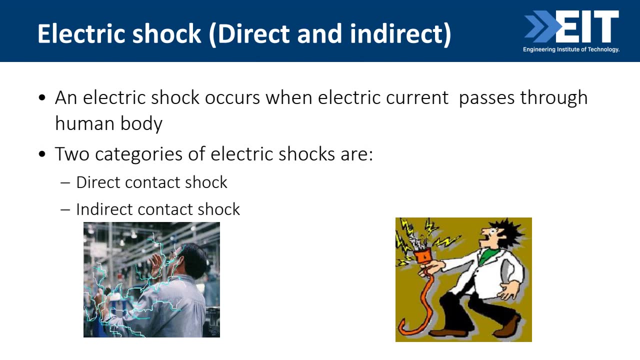 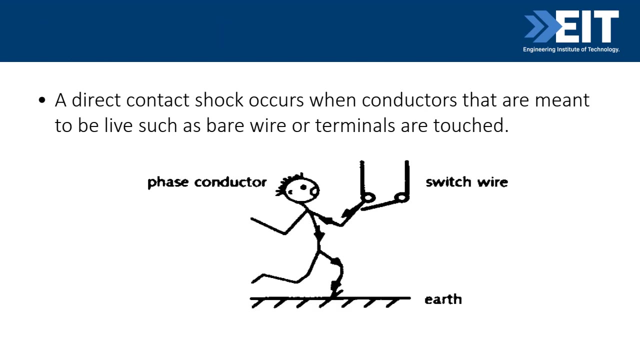 Okay, Pulses, but essentially, uh, reduced risk of fires and the idea is that everything gets taken down to a zero volts. and obviously there's two types of electric shocks: direct contact, indirect, very dangerous, anything to do electrical engineering very, very dangerous. and we have a direct contact when you touch the conductors, obviously to be avoided, and obviously indirect. 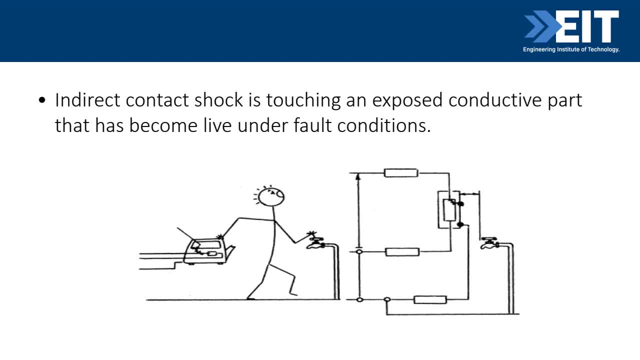 So the direct contact is when you're touching something like a tap, and there has been a very bad case recently around the up the road for me here where a little girl touched the tap and the electrician hadn't done the right wirings, particularly with the neutral cable. 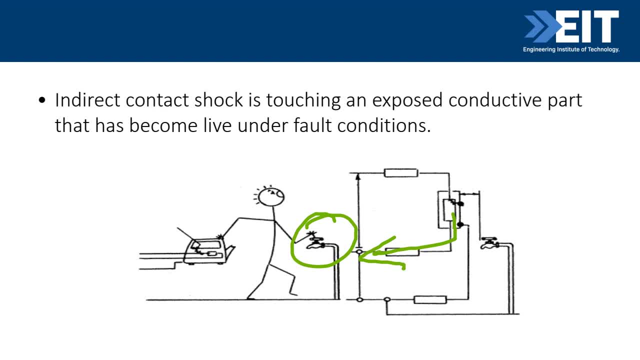 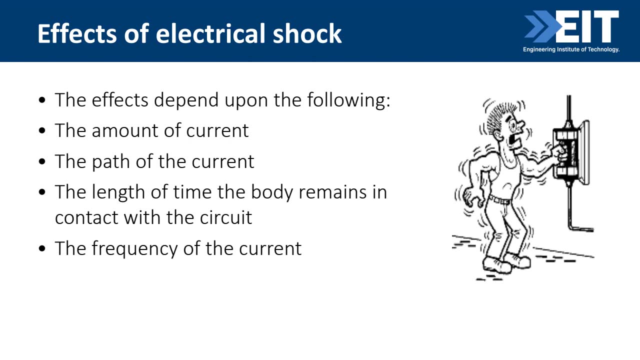 And, of course, bingo: the power went through the, the current went through the tap and this poor little girl was seriously damaged. So very dangerous. Um, and obviously the big issue with um electric shock is what goes through your heart, and it's in current. 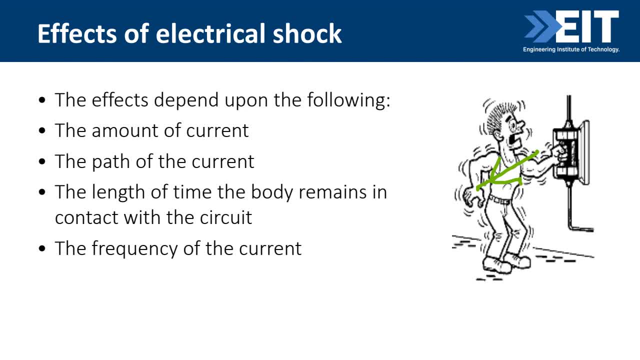 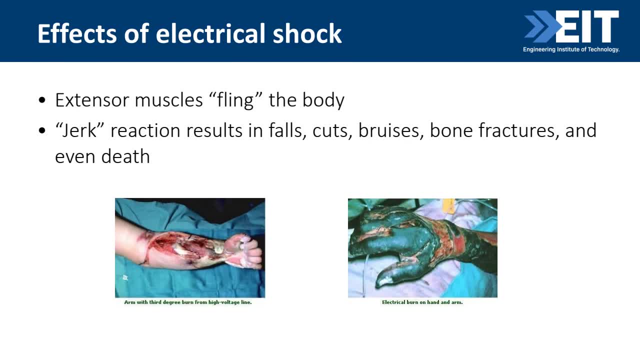 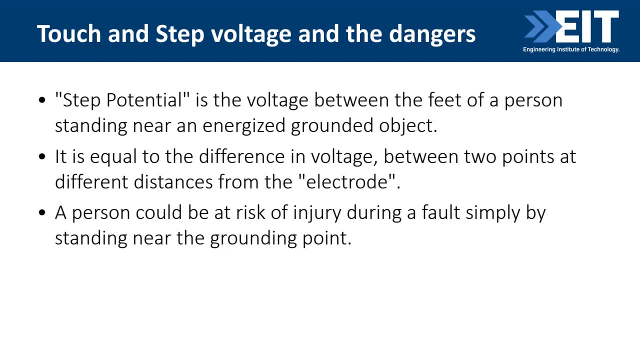 So there's quite a few issues there. the path so very to be avoided and obviously some horrific injuries very dangerous, And that's why electrical engineering is such a controlled thing. Now there's two um voltages which I want to mention at this section. 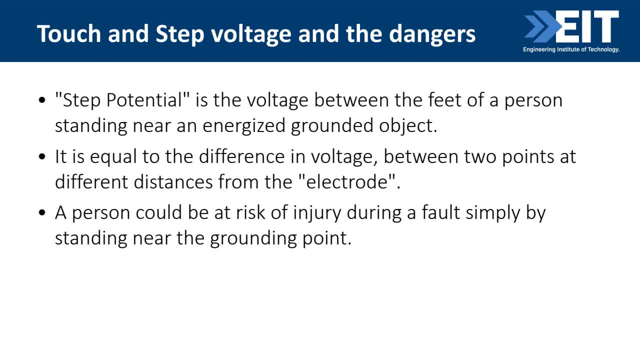 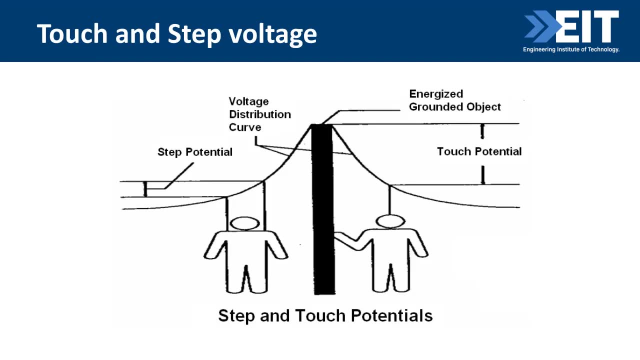 Um, thanks, Tony. uh, obviously, step potential and, um, touch potential. Just want to make sure you understand the difference, and the best way to explain it is a little diagram. Here's a touch potential. So here's, here's a structure here and that's the voltage going down, down, down, and that's what's going down. 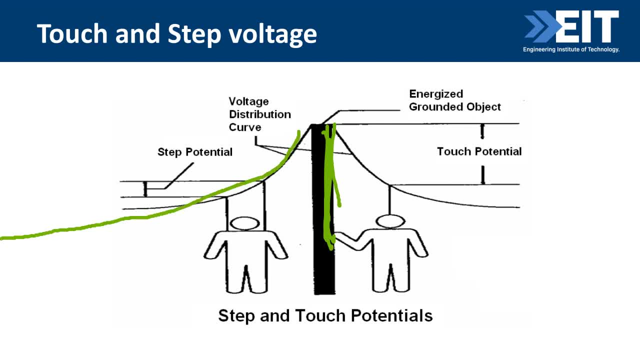 And the step potential is the voltage between your two feet. So if you standing one foot there, one foot there, you have a step potential and obviously touch potential could be far greater. You touching that and you're on some surface and of course you will then have a touch potential. 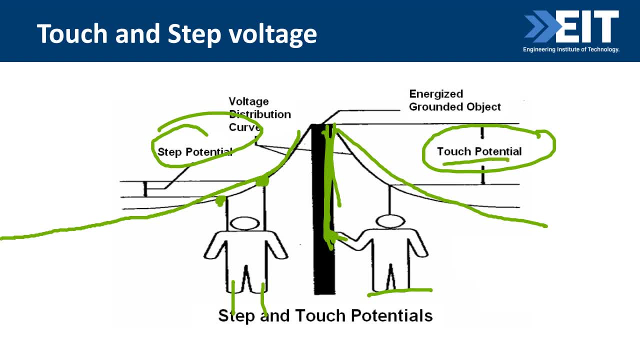 So those are the two. okay, When you touch the current cable, there's a difference between neutral earth. typically in a two corners cable the earth wire will be smaller than neutral. Thank you very much, Tim. Absolutely Right. These by these details are all in the slides. 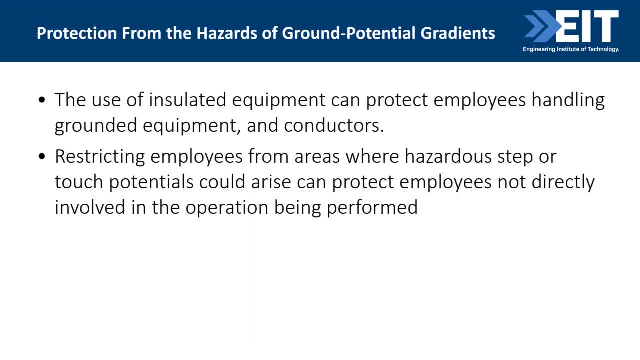 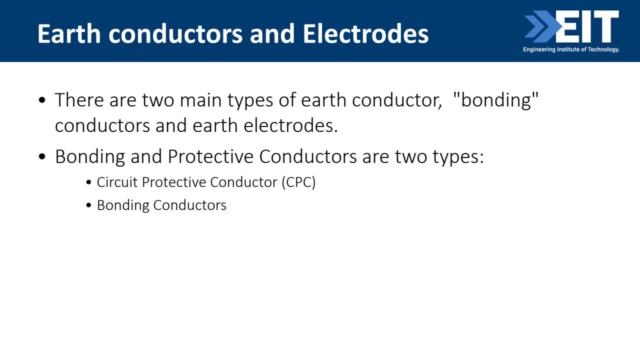 So you'll find it's all detailed here. Um, now there's two types of conductors: bonding conductors and earth electrodes. Um, I'm not going to go into earthing, but basically you I've got quite a few slides here to do with earthing because it's a particular area of interest to me. 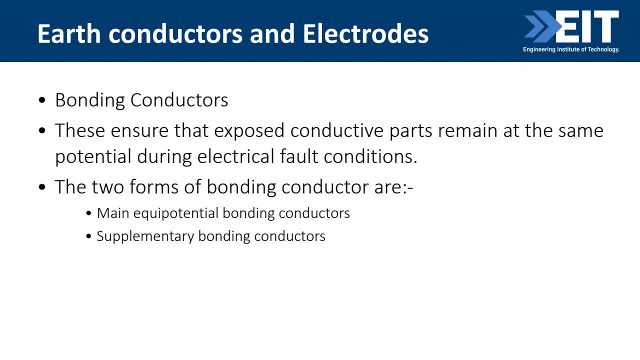 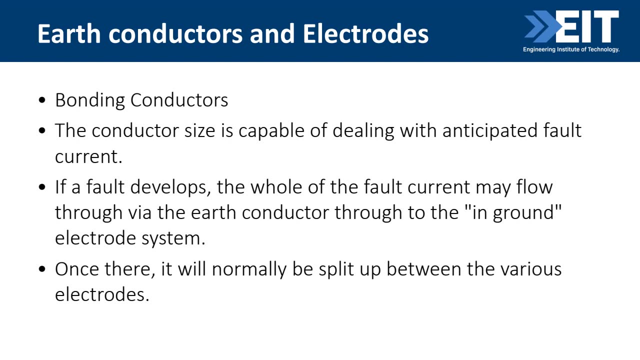 But bonding is when you tie two conductors Together and earthing is when you connect a stake. that goes into the ground is neutral, The same as ground earthing. Can everyone please text and answer in that box? It's not the same thing. 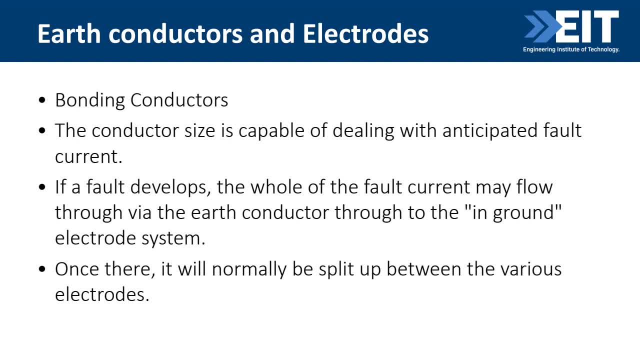 No. So basically the idea is that you have a, you have a neutral cable and you have a earth Cable and you have a earth. So they're green, yellow typically. here you'll see is earthing, and neutral will be Blue and live is Brown. 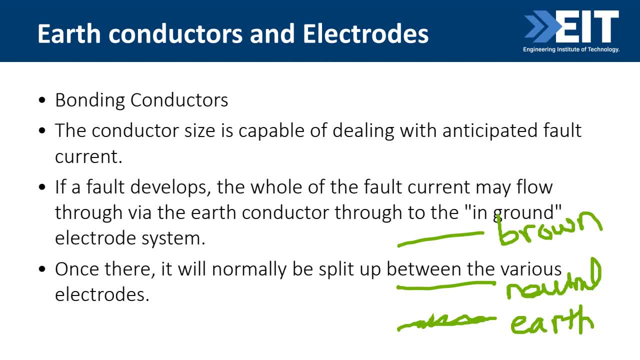 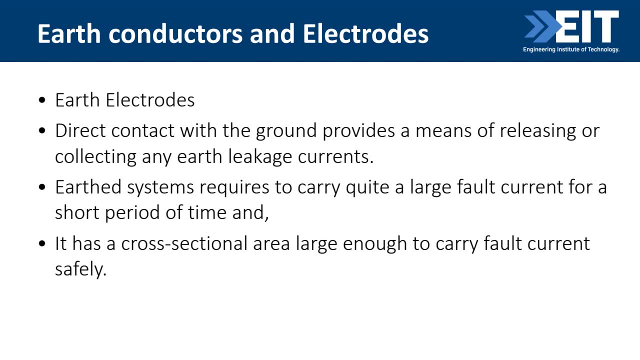 That's in Australia, And we want to obviously connect the neutral down to earth, But they are different, Right, All right, Thank you, Thank you, Bye, Bye. So earth electrodes are very important. It's a whole area of its own. What would be the? 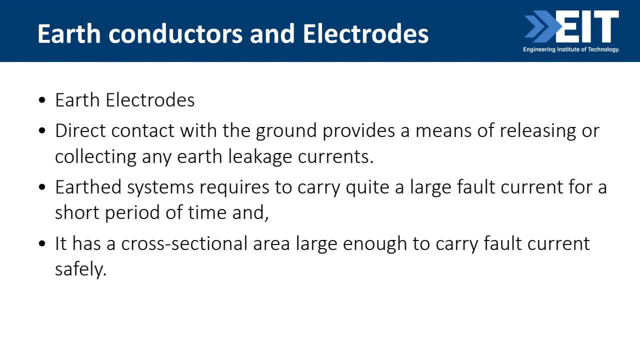 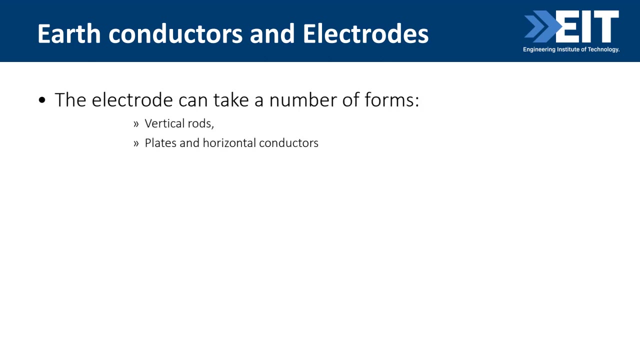 resistance for an earth conductor to ground. So an electrode is a stake in the ground and we then tie our earth conductor to that. And again, there's a lot of slides here relating to it. I'll just go through a picture here. Typically we have lots of different electrodes. 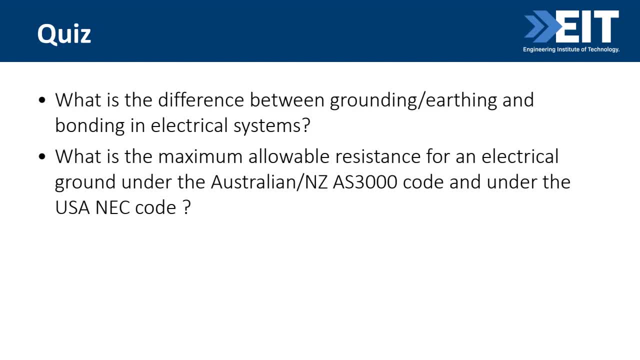 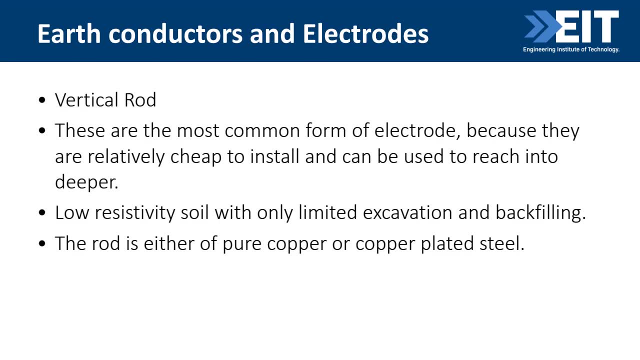 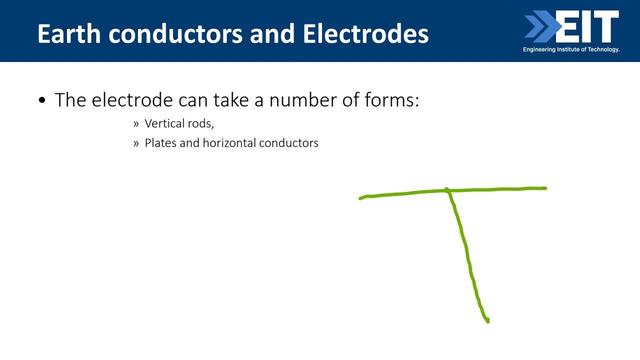 vertical rods and let me just have a quick look here, if I've got an earth. So basically what we'll do with an earth is you can have a vertical rod. typically a vertical rod goes into the ground and typically we would like a probably maximum of one ohm, but preferably 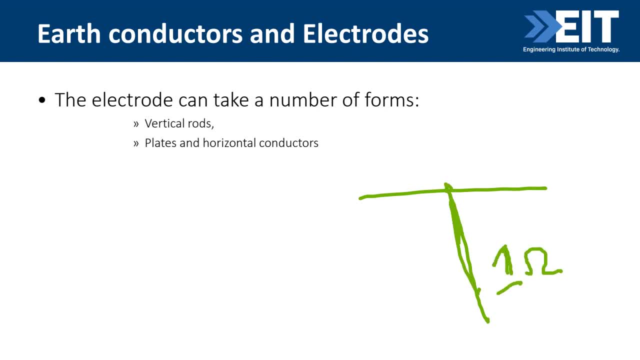 zero ohm, So you can. actually one of the biggest challenges with earth conductors is trying to get the resistance as low as possible. Thanks, zero ohms. You want it as low as possible because you want to make sure it's, and Pete has made a really really good point there. 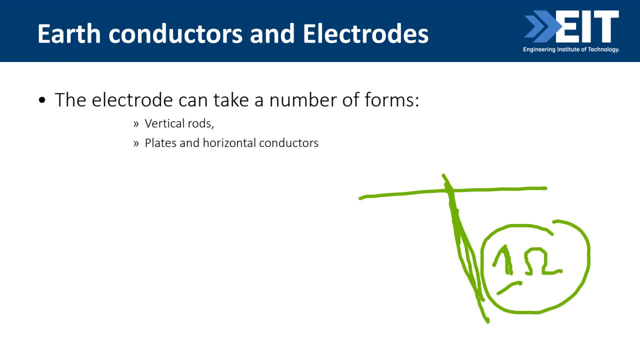 Thank you, Pete, for bringing it up. Sandy areas are more difficult to achieve a decent earth compared to wet soil, So it's a whole area of design really important. Thanks, Pete, Really important that. So earthing is very important. Yeah, Australia must be. 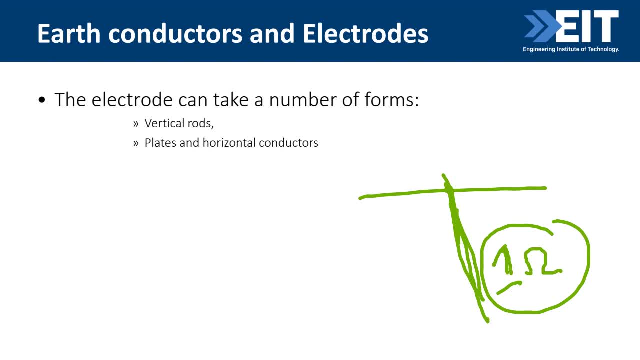 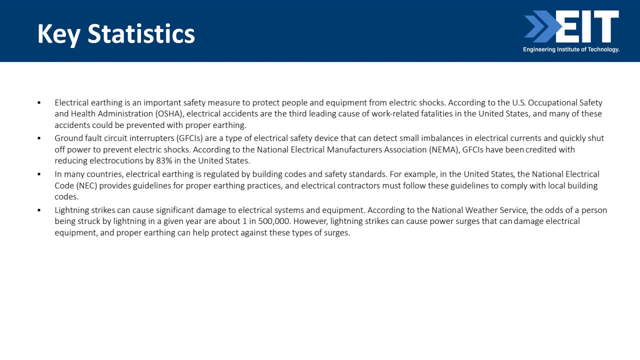 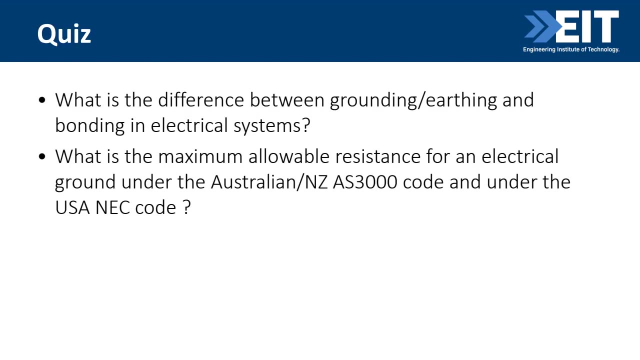 less than 0.5 ohms. You want it as low as possible. Use some bentonite. There are techniques to reduce the resistance to ground Okay. So obviously it's a really important issue and I suppose the question for you to answer in this little box: what's the difference? 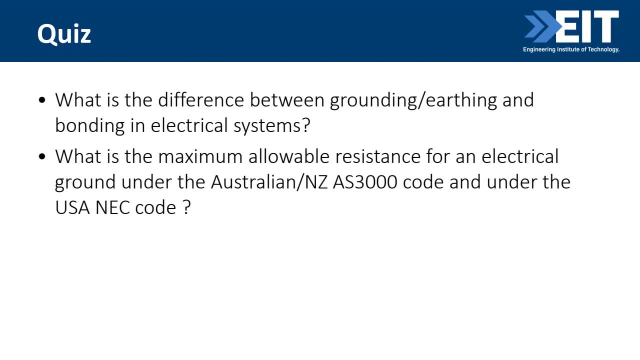 in grounding, earthing and bonding Electrical systems. Yeah. So what's the difference? Just type in the box. first one: How do you measure ground earthing? Yep, That's a very good question. There's a whole technique where you actually 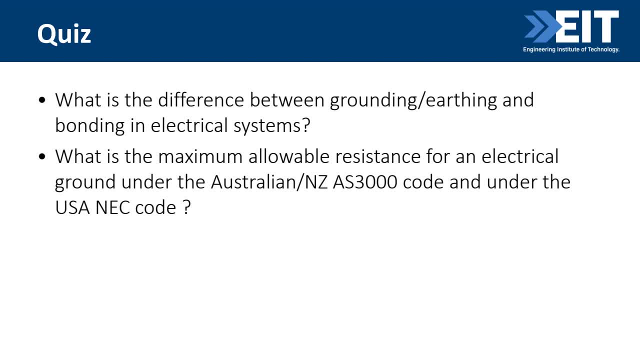 there's different techniques to measure the resistance, basically using an ohm meter, But there's a whole approach, because one of the biggest challenges- more, more, more- is measuring earth resistance, which I can tell you from personal experience is, if you've 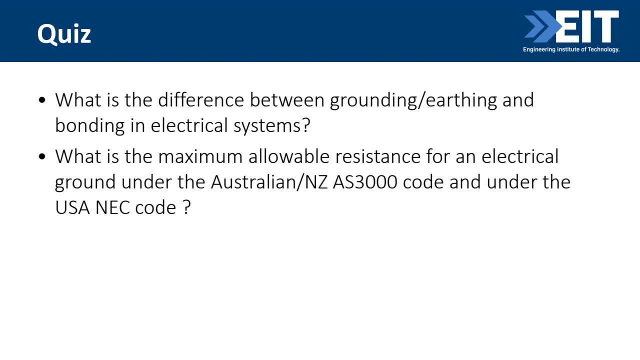 got any stray electric currents in the area, you could have a problem. So Dr Banishi Singh has got a really comprehensive answer. Bonding is a connection of non-carrying conductive elements like enclosed structures. Grounding is the attachment or earthing is the attachment. 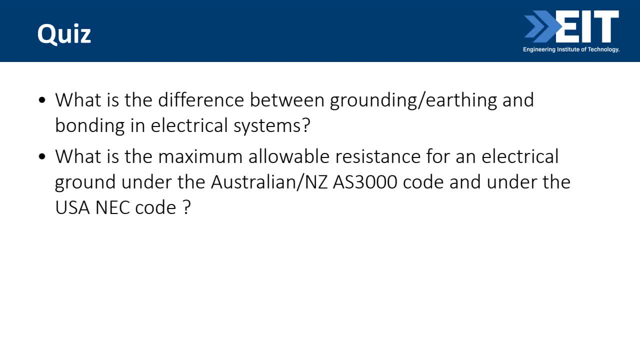 of bonded systems to the earth, both on estuary, to safeguard people and property from. Thank you so much, Dr Singh. Very comprehensive answer, And what's the maximum allowed resistance for electrical grounding? Yeah, So what's the maximum allowed resistance for electrical? 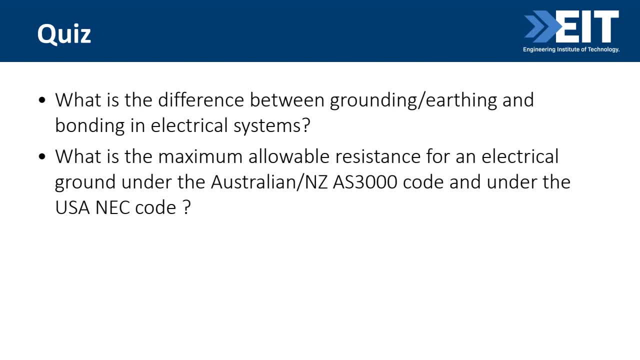 grounding. Is it around under Australian and under the USA code Anyone? I'm sure the Australians won't care about the US, but it'd be interesting just to know. Yeah, So as far as I know, the Australian maximum resistance, where you can't go above, is one ohm It's. 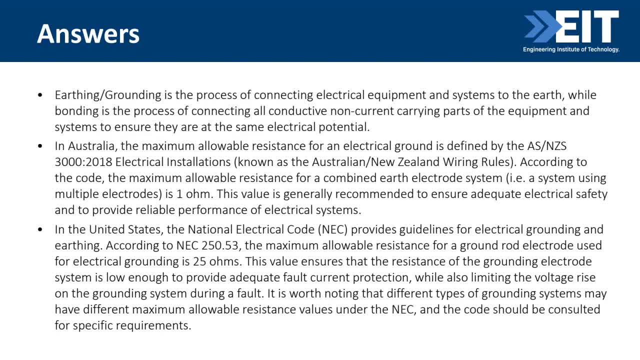 as far as I know, it's one ohm. So the ANZS2018 is one ohm, I believe, and in the States 25 ohms under the NEC code, So it's high. Obviously, 1 ohm is not a good one. 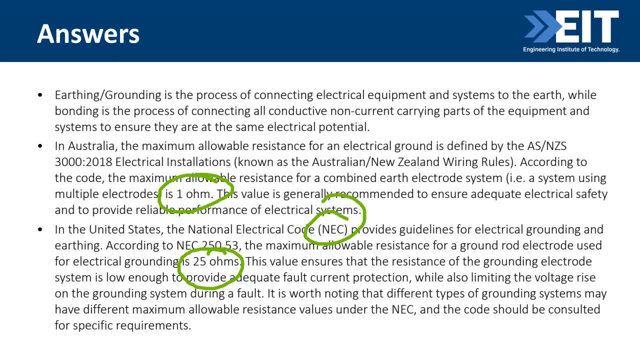 You want it 0.1 or 0.01, but that just gives you an example of the resistance. Just to give you, why would the US be 25 times higher? So, Scott, a very good question. That number is the maximum. 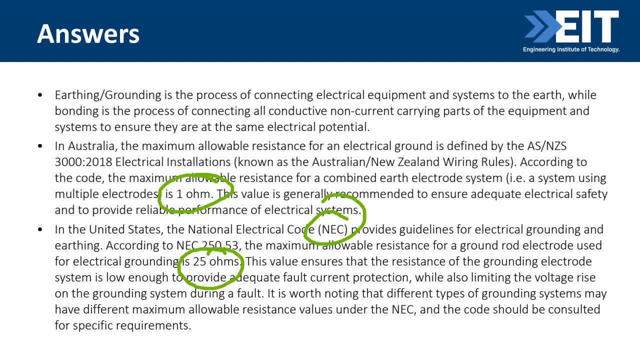 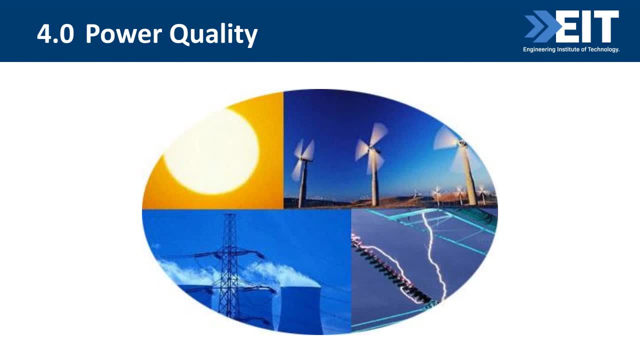 and the NEC code actually defines each individual area with specific numbers, which I haven't quoted here. So it's actually a lot more complex and, as Pete said, everything's bigger in the US, Pete. Okay, so power quality is the second last item. 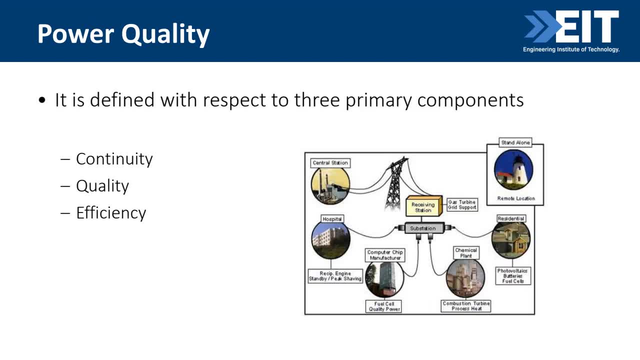 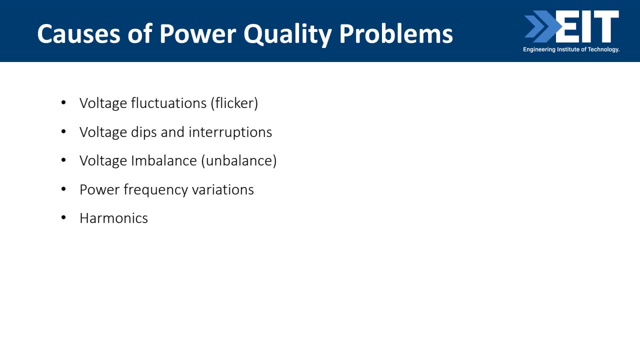 I've got to run. unfortunately, I know people are getting irritated. I can't carry on forever, So I just want to go through two more items: power quality and power system protection. So power quality is trying to say we want to try and keep the quality of power. 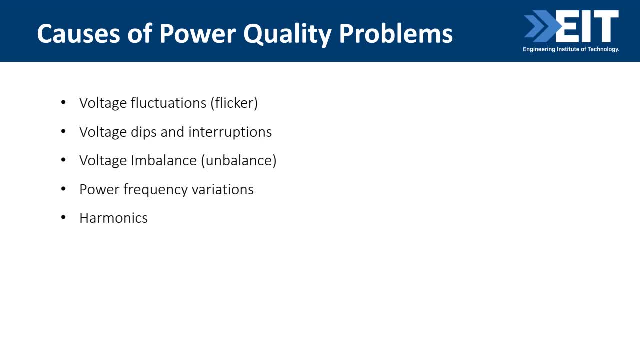 as clean as possible. So you get fluctuations, dips and interruptions, power frequency variations and harmonics. So there's different variations here. I just want to look at a few of them. I'm not going to look at them. You hear things such as voltage sags. 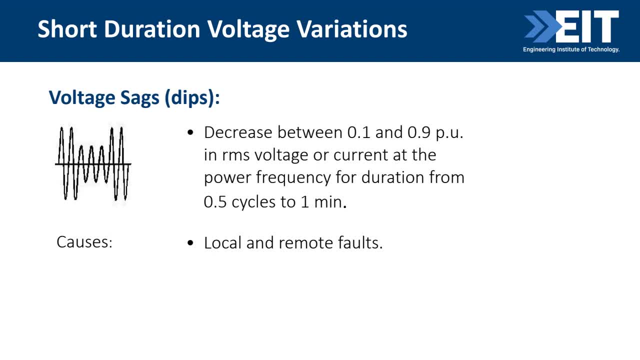 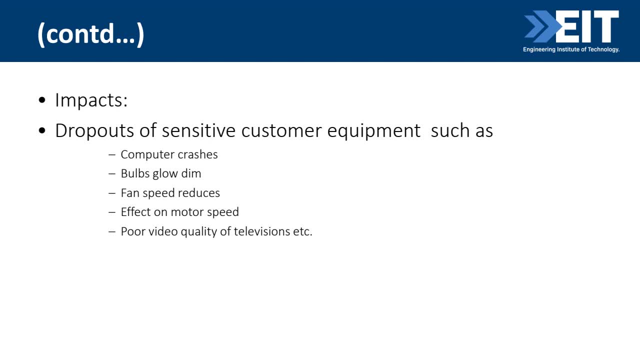 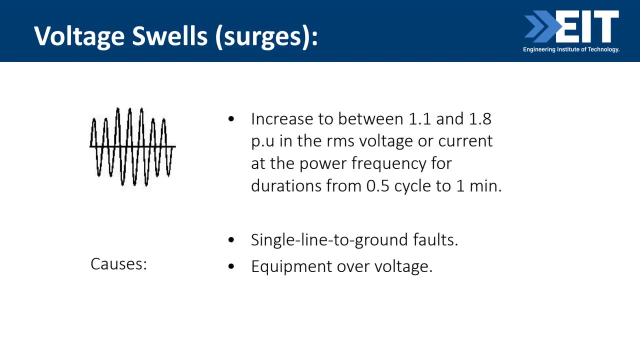 So it's a decrease in the voltage due to local and remote faults And you could have the result could be that your computer crashes, bulbs glow, dim, fan speed reduces, The voltage swells. Thanks, Dr Singh, Very good point there. 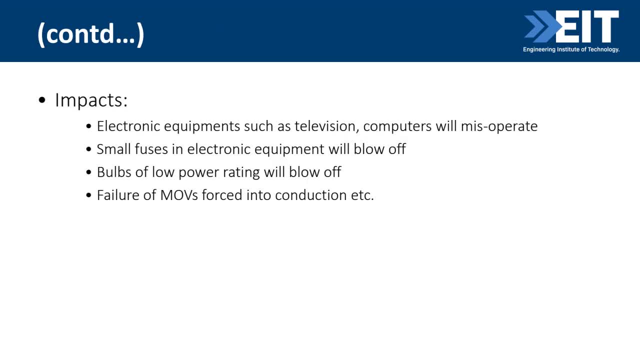 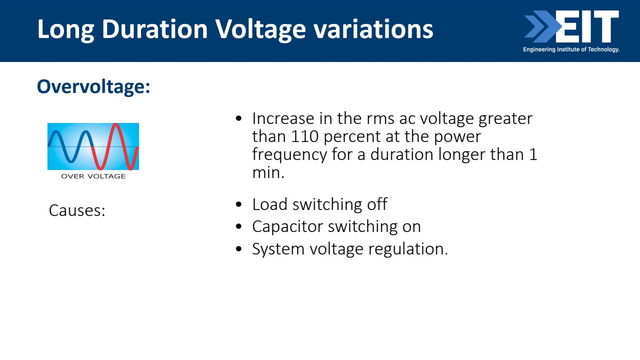 Single line to ground faults would cause this problem. here Equipment misoperates. So basically, with these issues with power quality, you can have some unhappy issues with your equipment Over voltage load switching off and on Capacitors- switching on is another one. 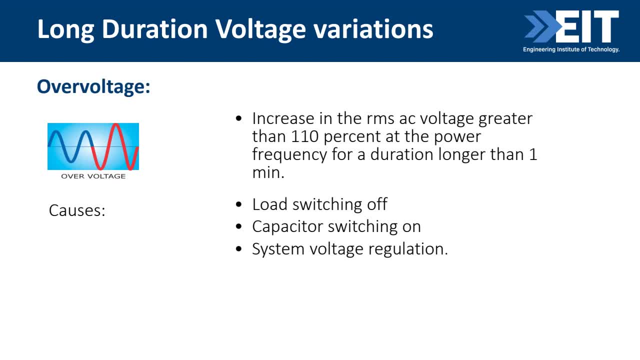 You may say, why would anyone worry about capacitors on your power system? Can anyone tell me I had a particularly bad event with capacitor? Yeah, voltage spikes. Why would you have capacitors on your system? Yeah, thank you Absolutely. 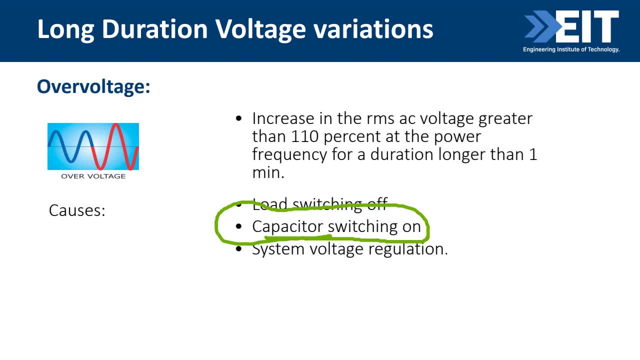 Who was that? Varun and Varun. Yeah, thank you. Power factor correction. Thank you very much, Yep. And in fact I had a particularly bad event. I won't mention the installation, but we had these guys doing some testing with. 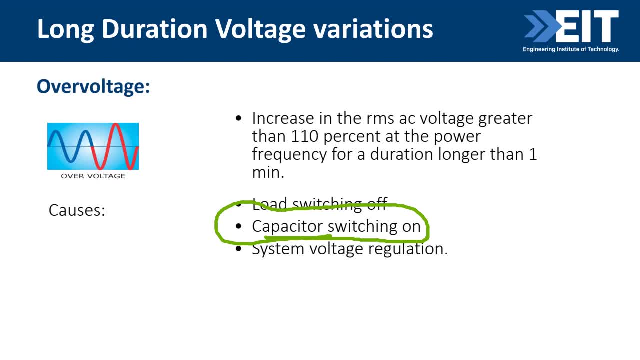 capacitor banks, some consultants, I won't mention their names. Anyway, they connected all the capacitors onto the end of the transmission line or the distribution line. Give me, let me get it right. And I was testing my variable speed drives. 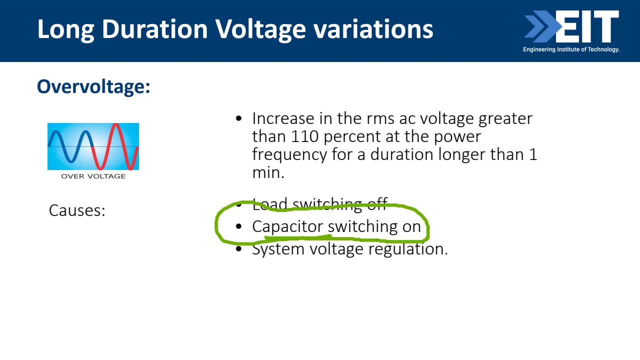 I had 15 variable speed drives In my MCC motor control center. I walk in and I see to my horror, every one of them overvoltage, overvoltage, overvoltage. They'd all had a spike going through them due to these guys. 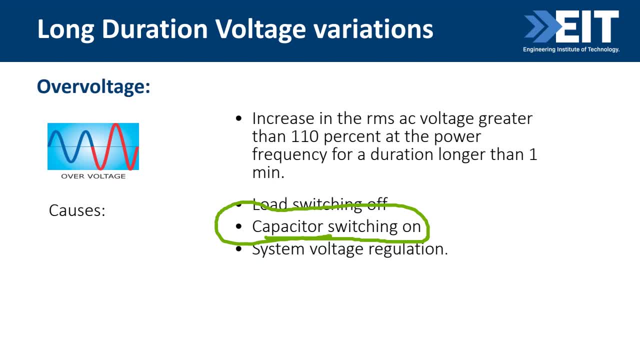 putting the capacitor bank on fully charged So I had the spike going through my whole plant and I was just installing. I had to bend. It was an absolute disaster And of course we fortunately could pin down height. I was measuring the voltages at the time so I could pin down. 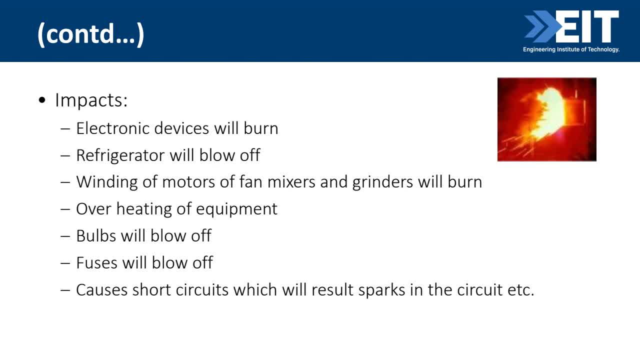 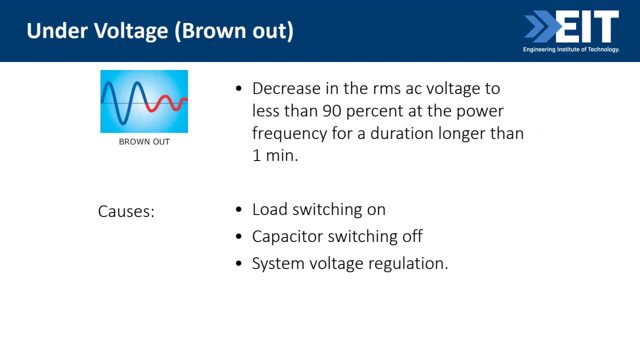 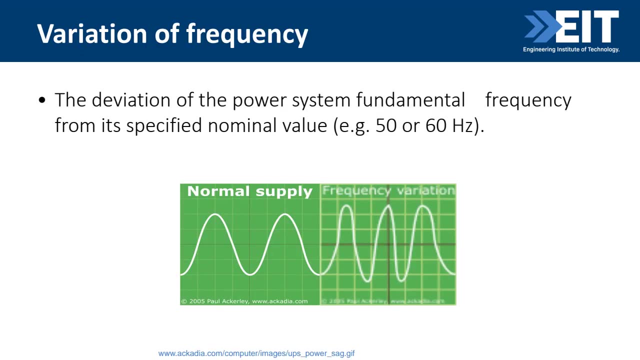 exactly when the spike came through and I could pinpoint who did it. It was a very awkward situation because it was a colleague of mine from these consultants. Anyway, undervoltage is another problem. Brownouts, as you sometimes hear referred to mixes and grinders, may not start. 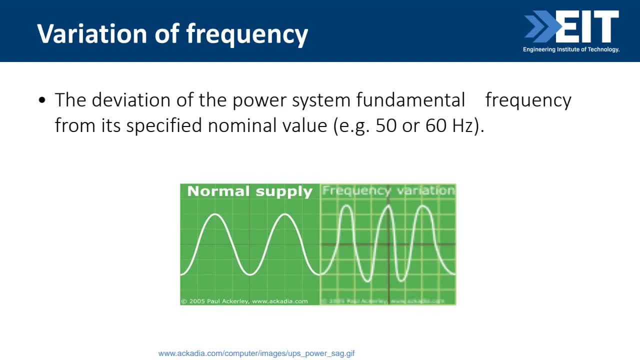 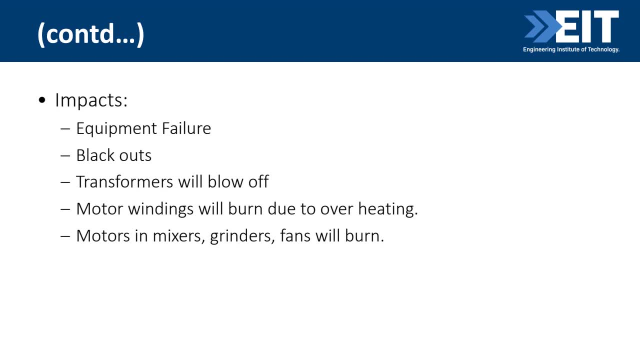 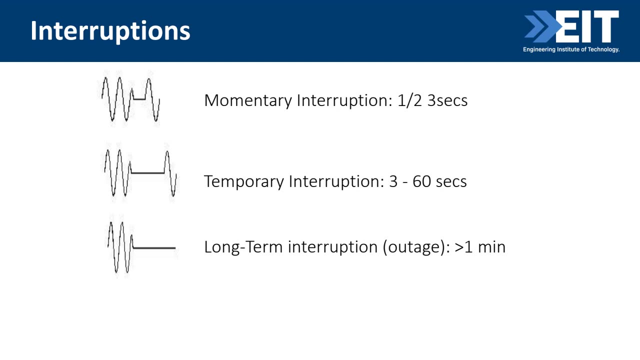 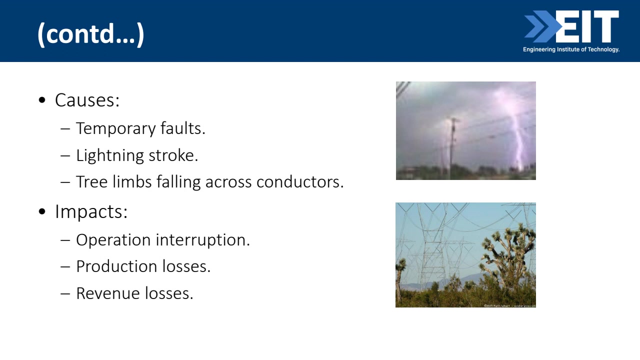 Variation of frequency from the fundamental frequency. That's another potential issue. Equipment failure would result. So these are all Issues that you need to watch out for. Solar impacts: Yes, that could be an issue as well Surges. So this is an increase of 110% of the normal voltage. 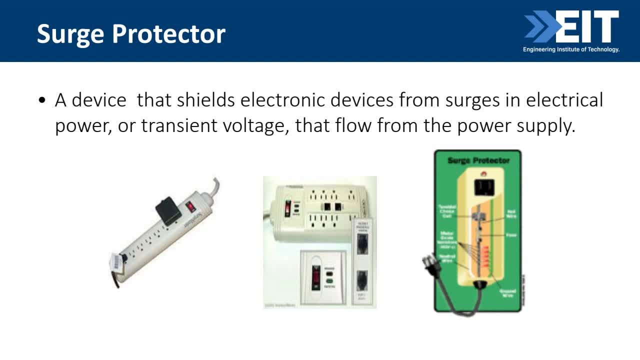 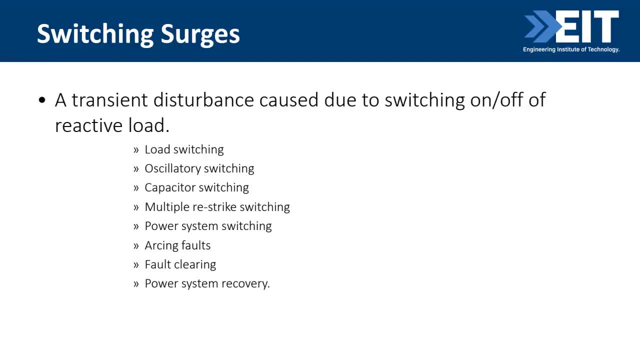 Surge protector can help you, So it's particularly important. So some countries where you have a lot of spikes, you need surge protectors as a critical part of your life. One issue here is you're dealing with data Communication systems. What's the best form of protection? 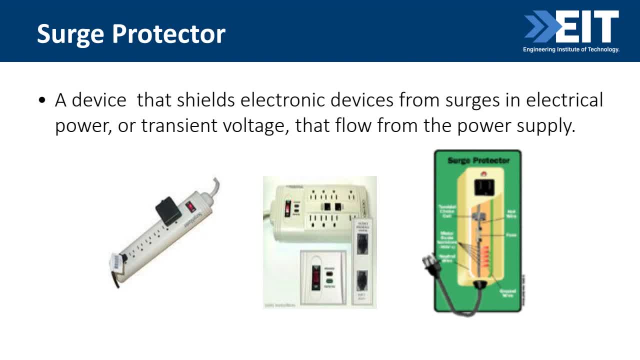 Can you want to tell me DC block? Yeah, surge arrestors are helpful. Best thing is to go for fiber. fiber optics- Beautiful. No connection to the for your data communication systems. What's the difference between batteries? How to improve power quality. 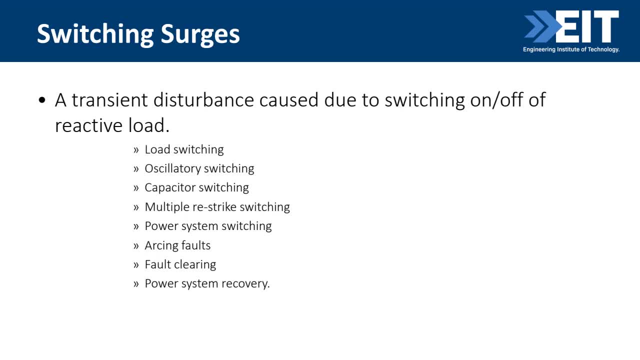 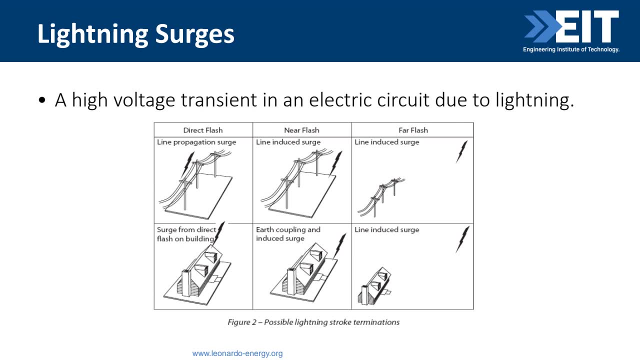 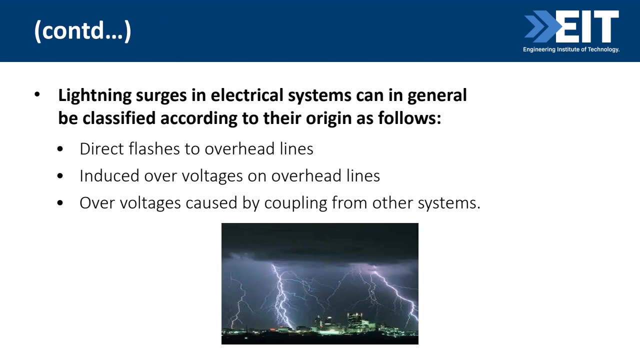 Yep. So these are all issues: Issues with switching And obviously lighting can be a problem And there's different types of flashes- High voltage, transient And obviously Potentially big problem. So you need to make sure you put surge arrestors in. 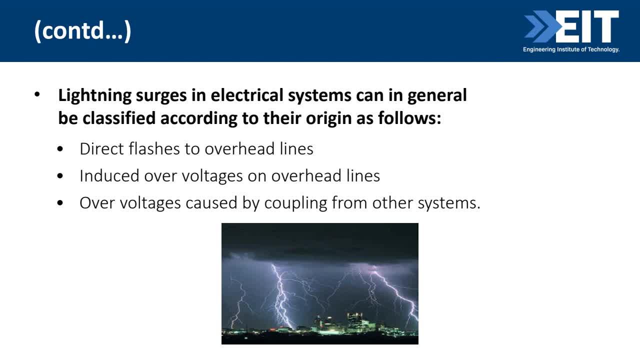 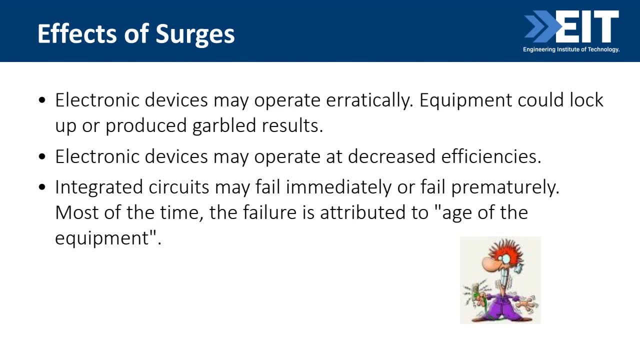 Otherwise you will pay a price. And, as I said, try and use fiber for any communication systems. So make sure your computer's protected. And also, sometimes you find your computer Locks up, your equipment Locks up. It may be a spike coming through your data communication system. 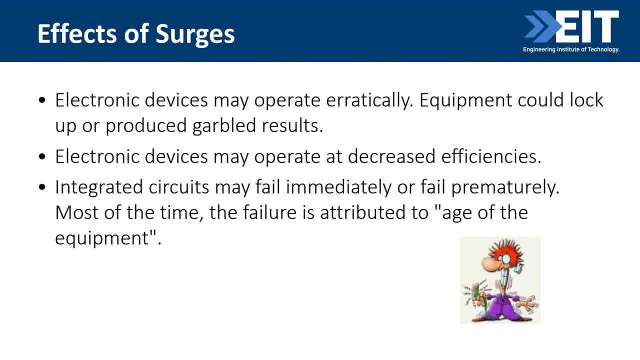 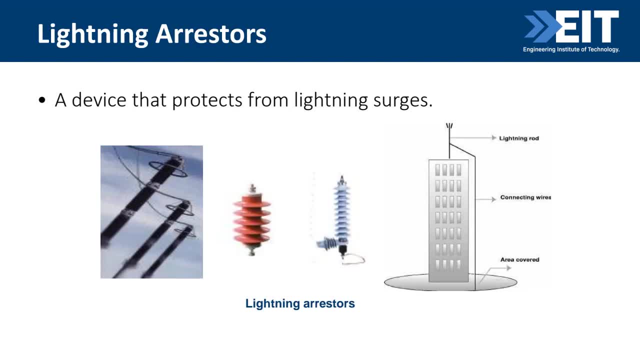 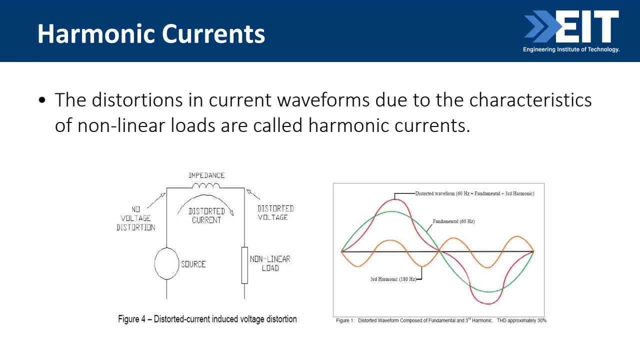 Fiber will solve that. So obviously to be avoided at all costs. So slightly assert arrestors. Um, and obviously what I want to show you is that if you put your oscilloscope on, what a poor power quality will show you is something looking like this: 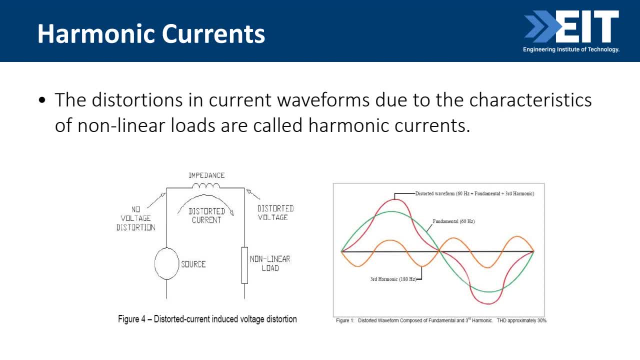 So that's the sort of signal. So you should see a nice clean sinusoidal signal. but you see that, Yeah, you get all the slides. Don't worry. Galvanic isolation can help, but, um, fiber optical isolation is the best. 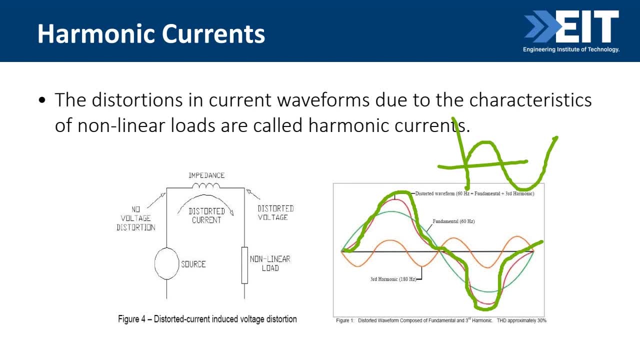 Um, so you want to clean signal and you get that, And basically this thing you can actually use what you call a Fourier decomposition. So you want to clean signal and you get that, And basically this thing you can actually use what you call a Fourier decomposition. 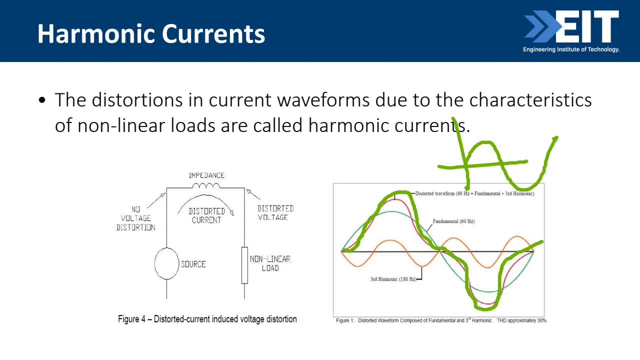 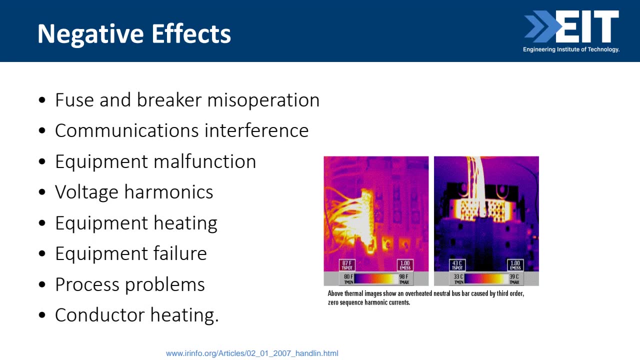 And basically this thing you can actually use what you call a Fourier decomposition And you'll see that a signal like that is decomposed into a whole series of harmonics, different frequencies. So when you hear harmonics, it's basically a bad, badly distorted signal voltage which is broken into a whole lot of different harmonics, different frequencies. 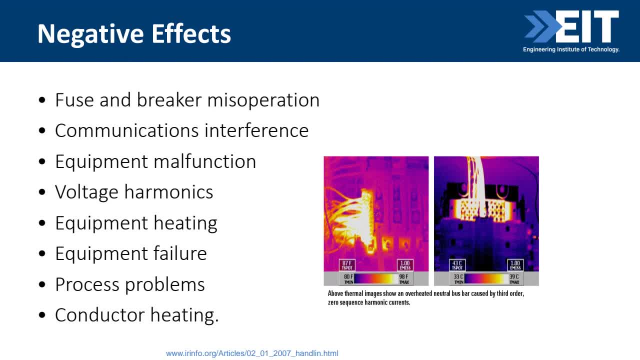 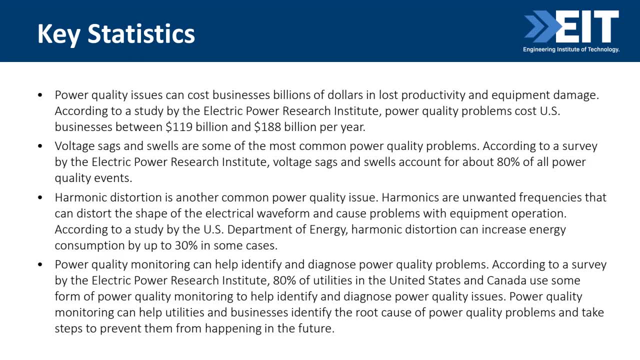 Not all comms have fiber interface. Yep, that's true, Absolutely right. So lots of issues. So lots of issues with um power quality and obviously the point to make is that, uh, billions of dollars. Obviously, the point to make is that, uh, billions of dollars. 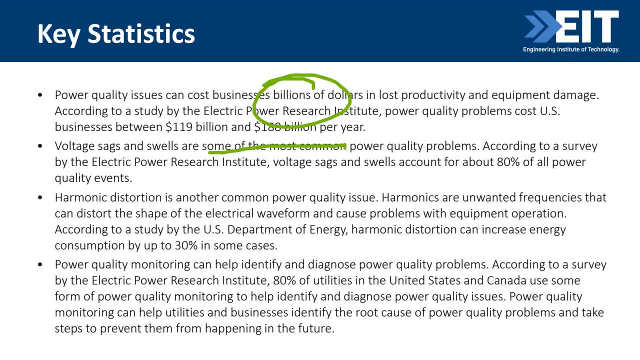 Most common is voltage sags and swells- 80% of all power quality events. Most common is voltage sags and swells- 80% of all power quality events. And the other point is um power quality monitoring can help. 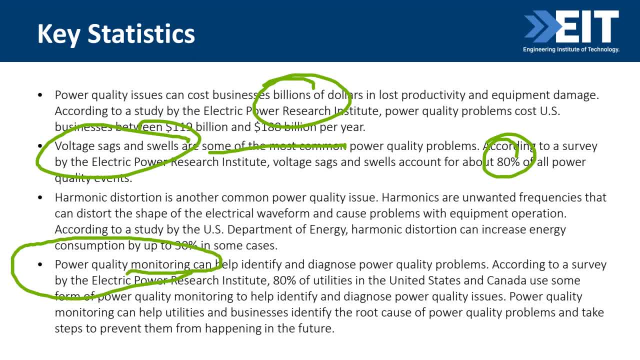 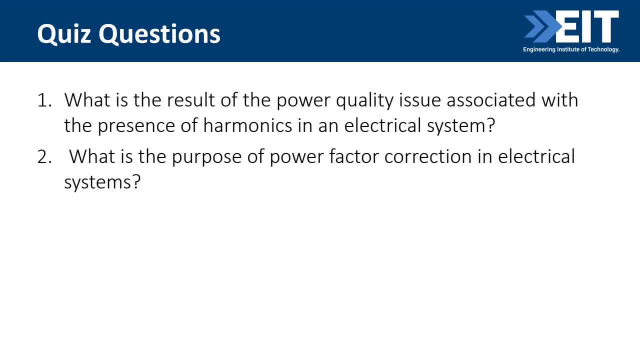 So you can use the to monitor and diagnose. So I suppose the first question for you there is Okay question is: will there not be clean power from the generating station? Absolutely right, Locke The generators, the suppliers have to have clean power. but unfortunately, with all the electrical disturbances, lightning, people switching on and off their power, it all creates lots of rubbish, electrical rubbish on your lines. So that's the problem. 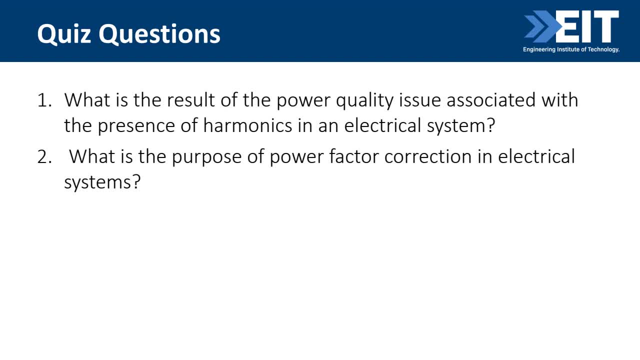 Okay. so question is: what is the result of the power quality issue associated with the presence of harmonics in an electrical system? Can anyone tell me? Yep, okay, so high electricity costs, noticeable decrease in equipment reliability, power surge- Yeah, thanks, Michael, That's what I was looking for, But all the other comments are quite right as well. Extra heating: 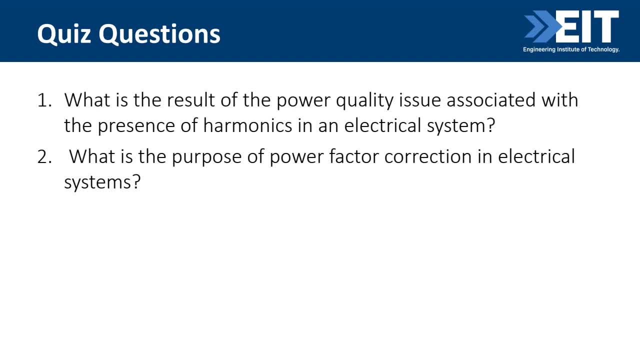 Thank you. Thank you very much. And what's the purpose of power factor correction? electrical systems For our compensation? Yep, absolutely right. So basically, the idea with power factor correction is really putting capacitors in. means that if you plot your voltage, that's your voltage and this is your current. we try and keep them as close as possible. 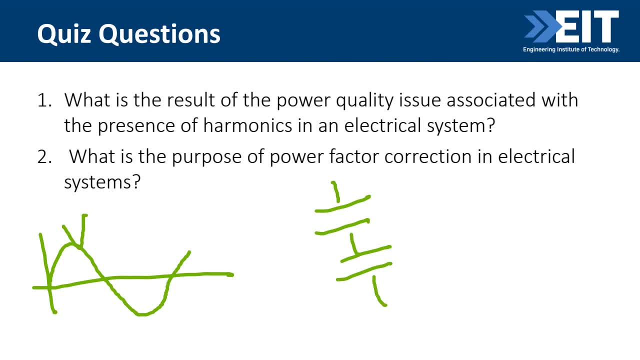 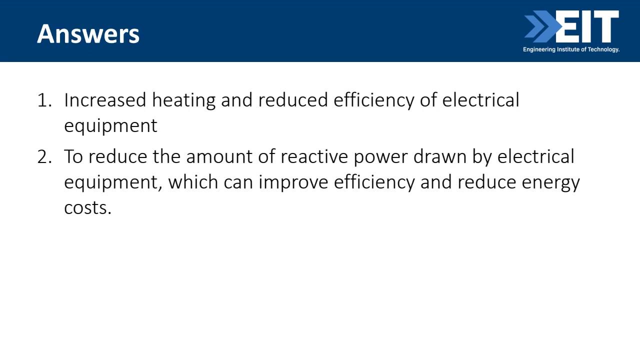 So we want them basically as close as possible to each other. So power factor correction always helps because most of our loads are inductive. So putting power factor correction in we can actually line them up. Thanks very much. The suggestions from everyone are just perfect, Thank you. So increase heating, reduce efficiency. So I think everyone got that. And power factor correction is. 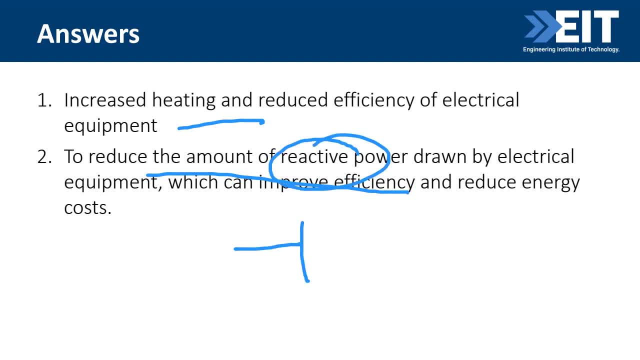 So we want to reduce the amount of reactive power, So reactive power is associated with inductors and we put capacitors in and that cancels out the effect of the inductors. So inductors, you have lagging power factor, capacitors, you have leading power factor and you bring them together So your current and your voltage waveforms just line up. Yeah, you can get all the slides, No worries, Don't worry, All will be well. 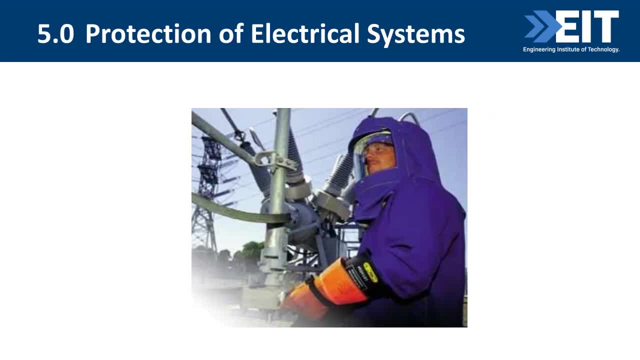 Okay, so the last section I want to do and, Barry, I'm so apologetic I've overshot by 15 minutes. I'm probably going to be shot at dawn. I just want to finish off with the last component here. Barry, are you still with me? 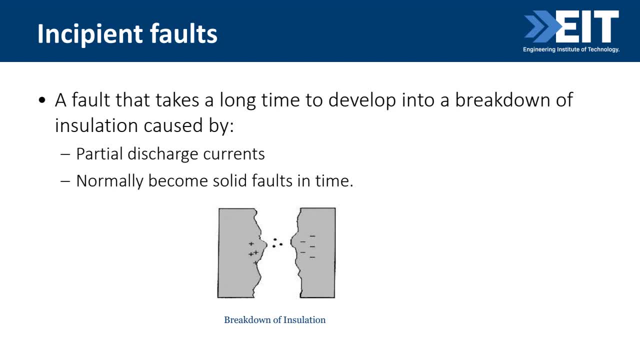 It's okay. It's okay, Steve, I'm still here. Yeah, You're still there. Thank you very much, Barry. I'm sorry to overshoot Another seven, eight minutes. I just want to cover the last topic, which is protection. 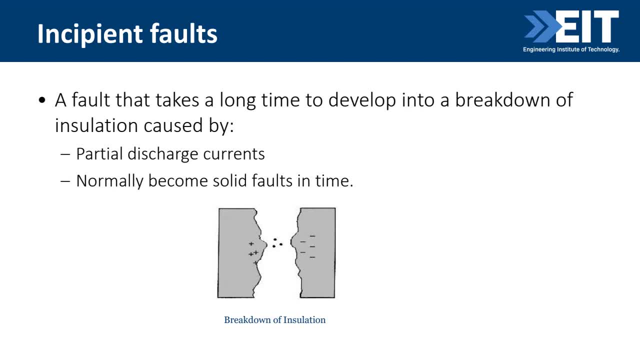 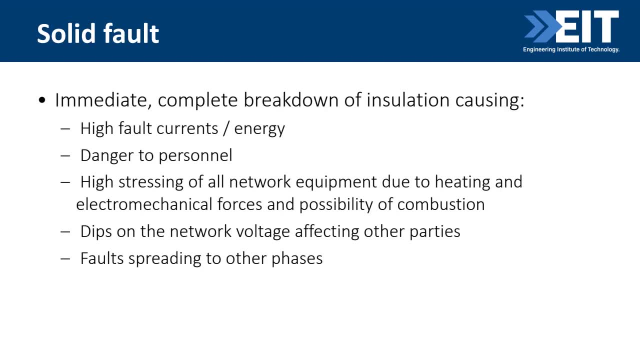 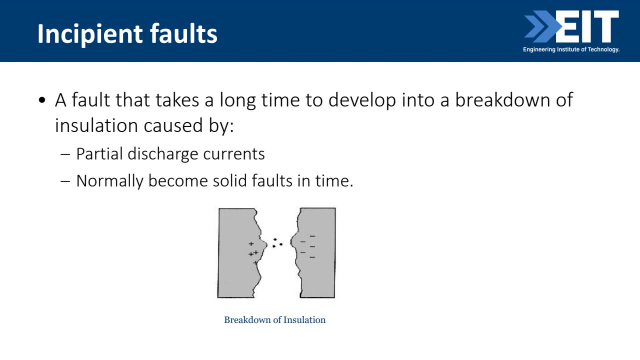 And protection is so important, Absolutely critical, And it's a very, a topic very close to my heart, So I just want to mention it so you know what protection. So you've got two types of faults: Incipient faults, which is a breakdown, insulation- And some of you may remember, if you've got gray hair like me- insulation, which is sort of paper insulation around cables, And of course old cable PVC is worn down And of course you get slow leakage of current. 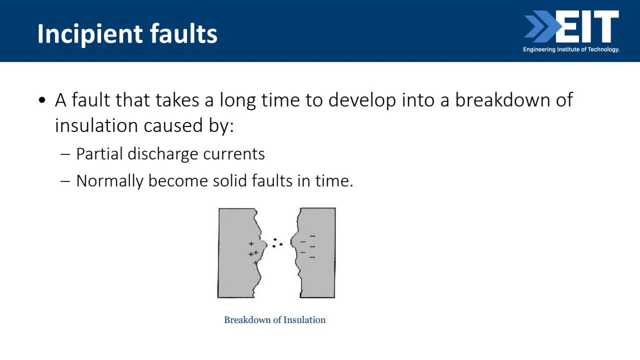 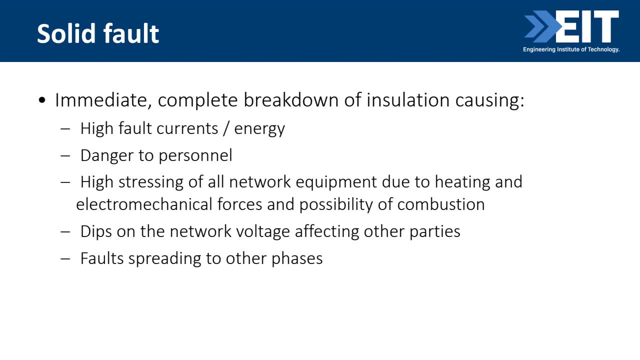 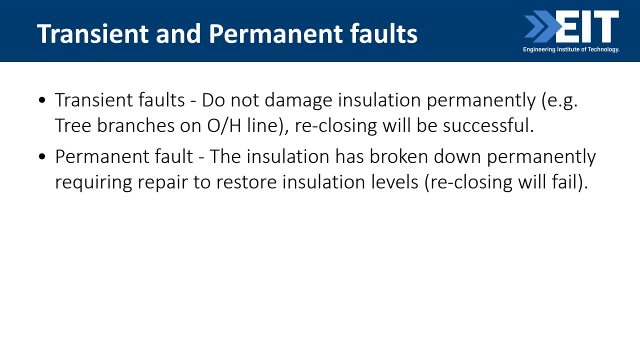 And solid fault is a fault from something damaged, complete breakdown of insulation, solid fault. So really transient faults are. you know, tree branch falls across your power cables, It will all be sorted out, Just temporary. Permanent fault is something where you've got a permanent fault And as soon as you try and recalibrate. 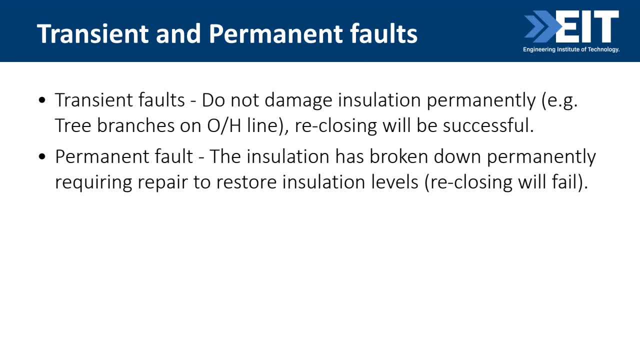 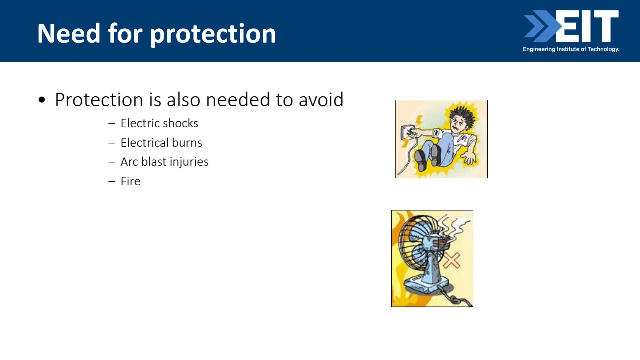 Close with power, it'll trip out again. So we've got two types of fault: transient and permanent faults. So just want to spend a few moments. What about a six ohm snake? Thanks very much, Michael. Thanks, Garth, for coming along. I'm sorry I was overshot on time. Protection is needed, obviously to avoid electrical shocks, electrical burns, And obviously every household has protection- earth leakage protection- which I'm not going to be spending time. 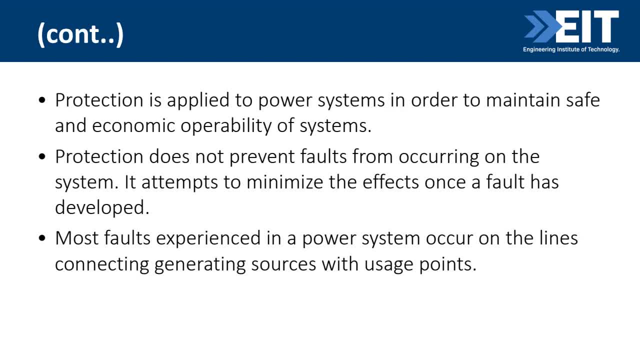 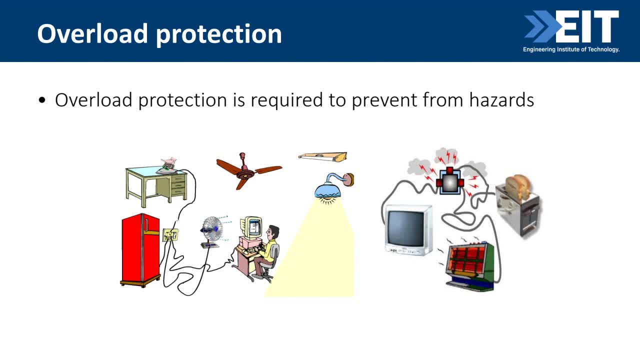 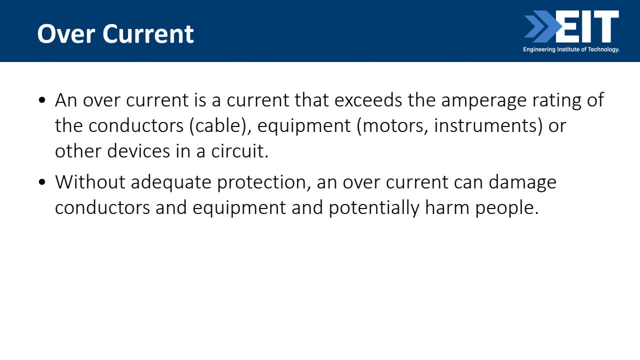 And we obviously need to look at overload, overvoltage, overload protection, protect from the hazards and overvoltage, So overcurrent, where the current goes up and it goes beyond the rating, and we need to protect the cables and the equipment So we can damage and overvoltage can also be damaging. 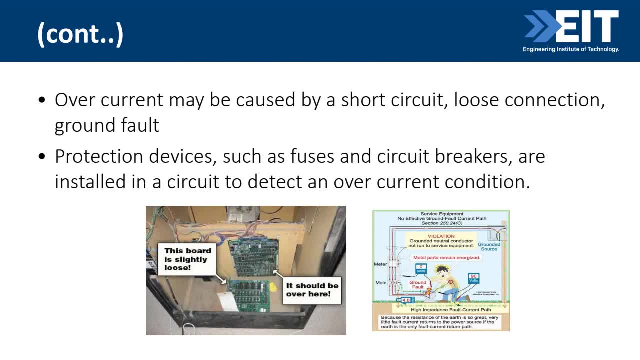 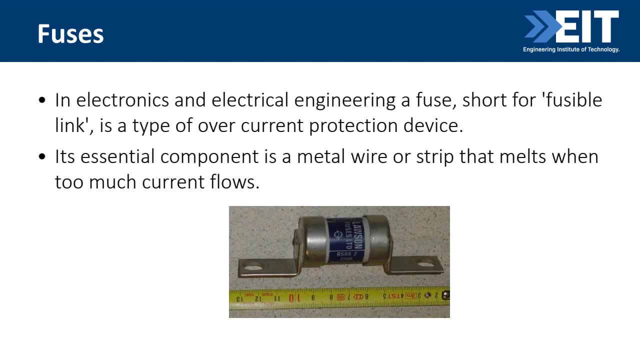 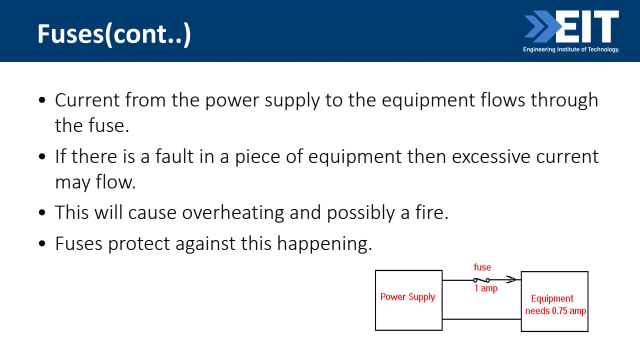 So the best, easiest device is: thanks. so much, Pete, I'm sorry. Thanks, Garth, for coming along. Pete, thanks. Fuses are obviously a very important protection, But the problem is, once you blow your fuse, that's it. You have to replace the fuse. 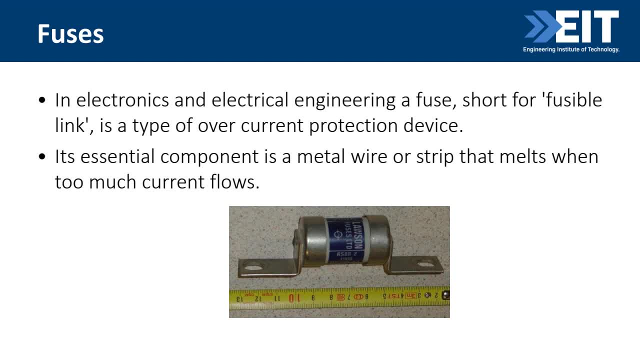 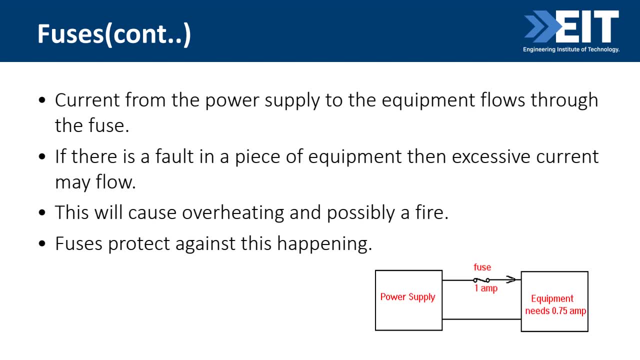 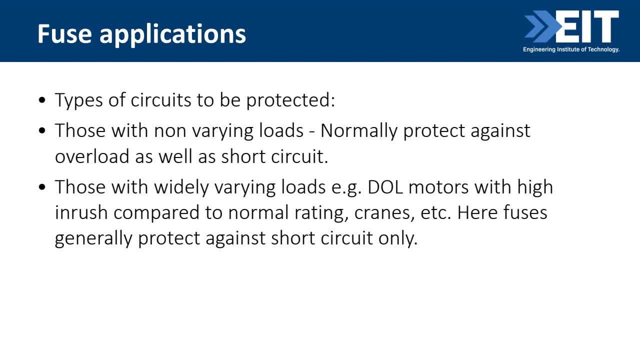 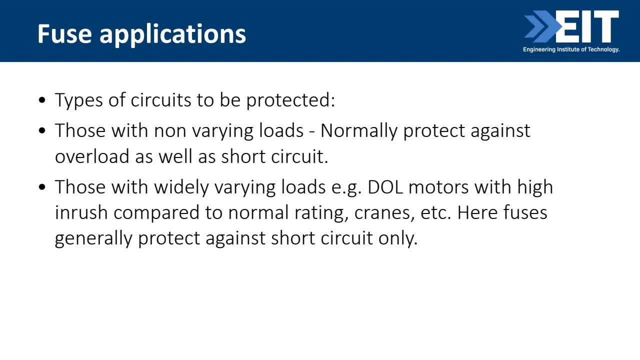 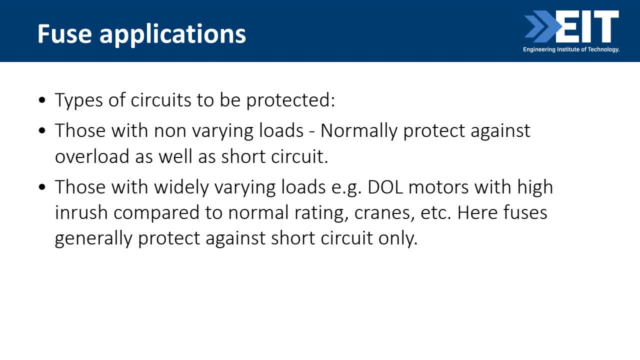 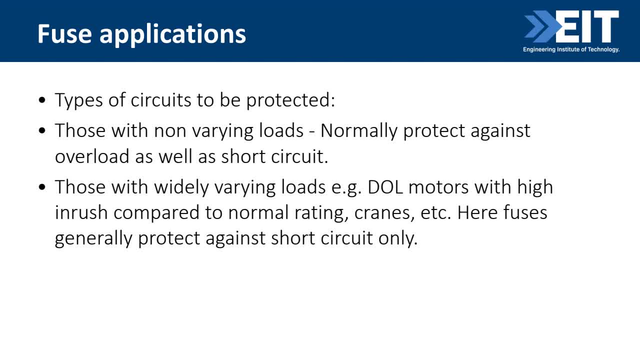 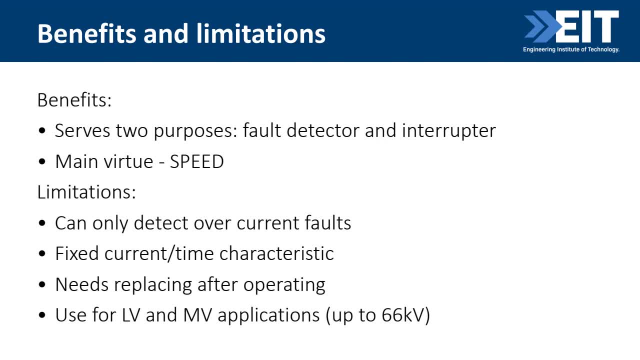 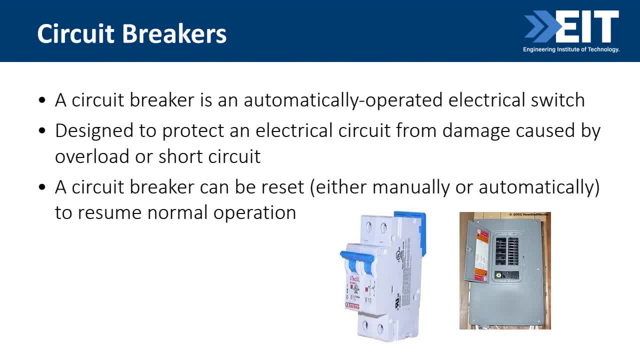 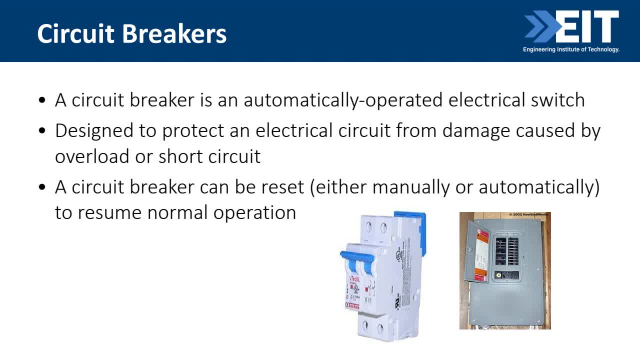 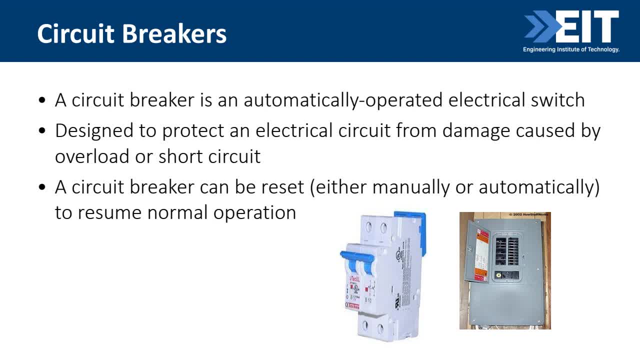 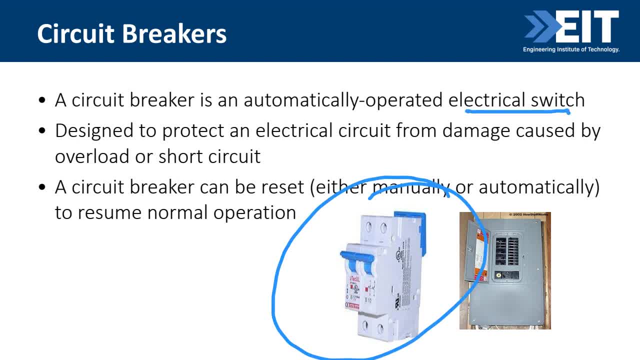 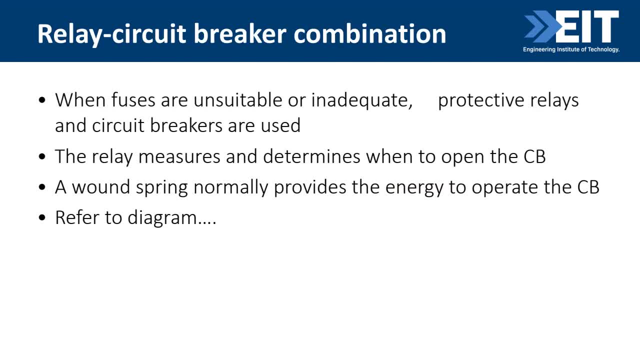 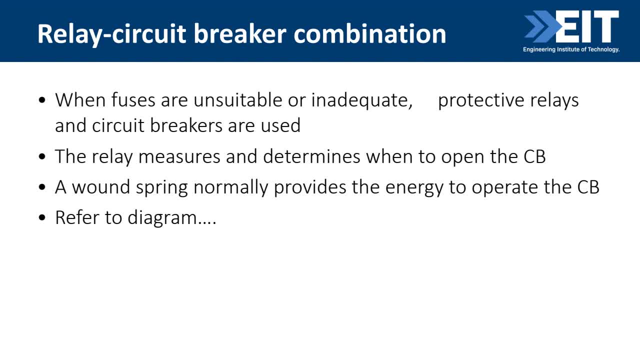 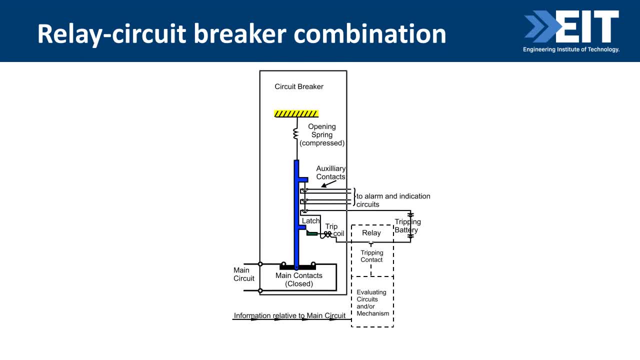 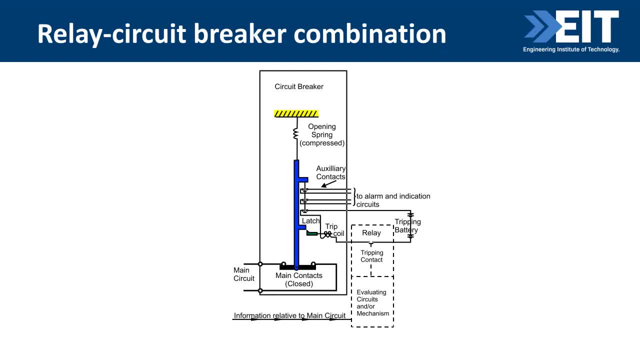 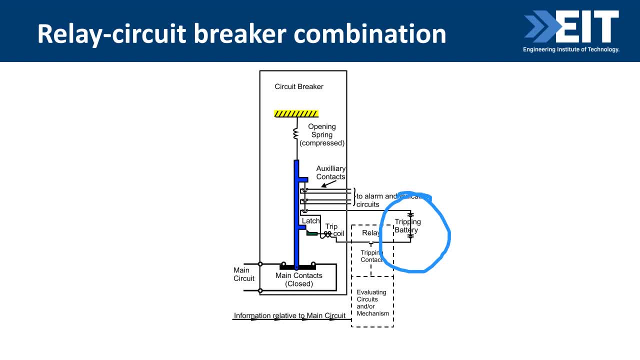 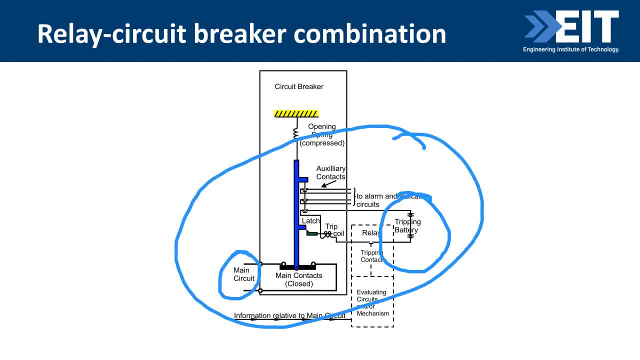 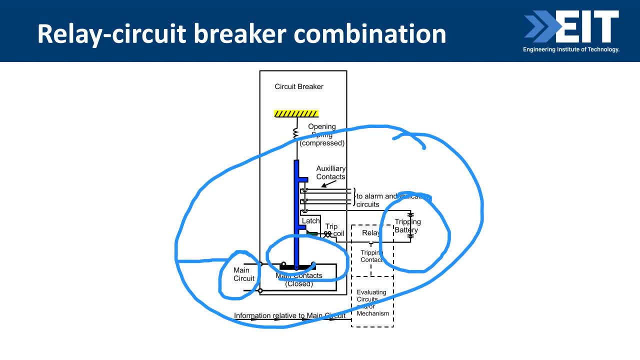 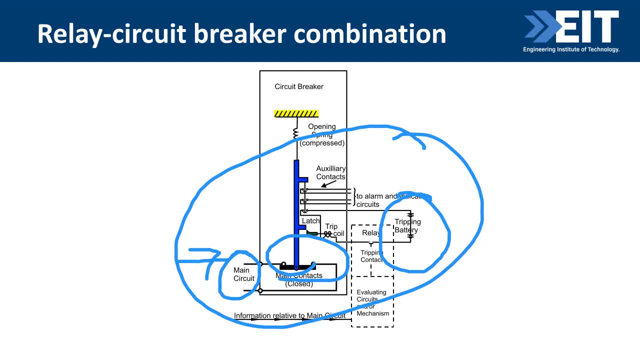 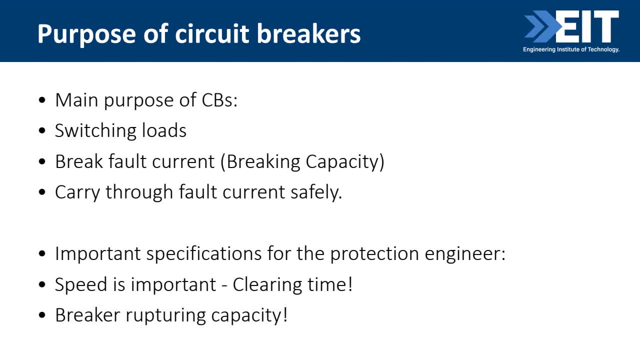 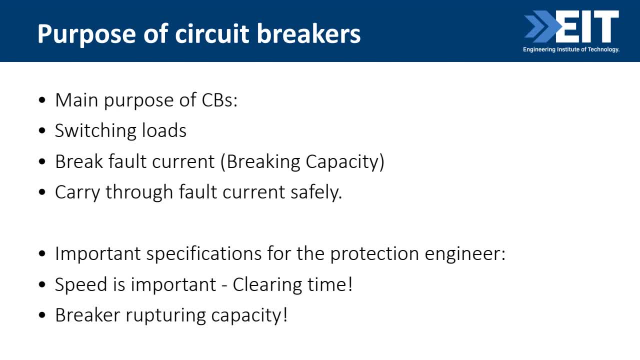 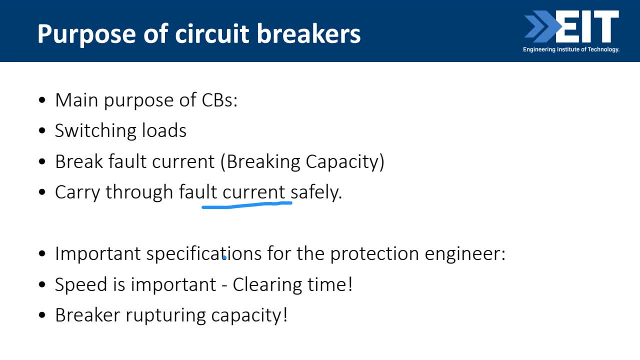 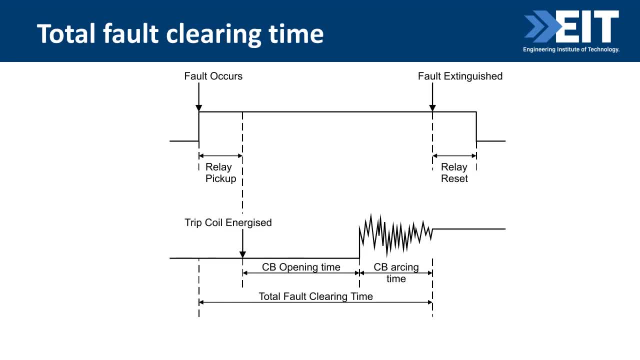 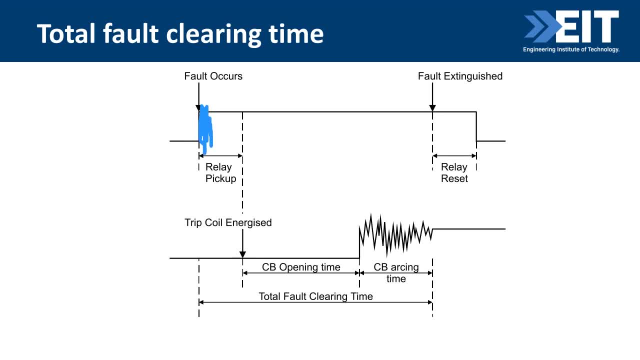 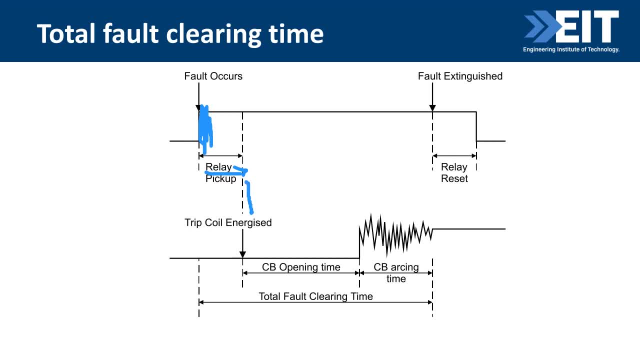 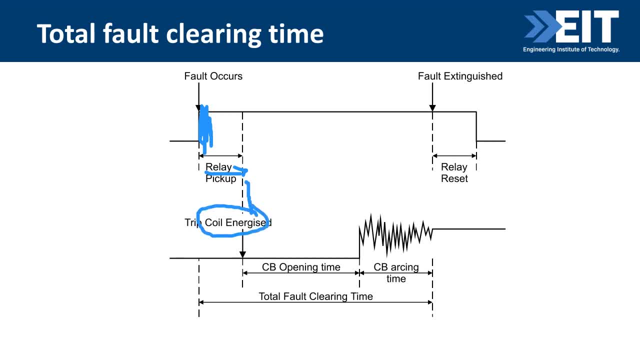 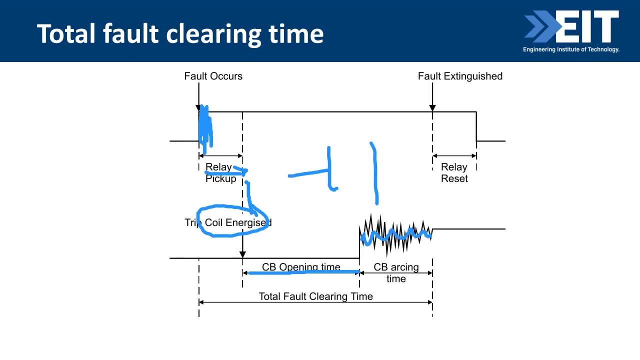 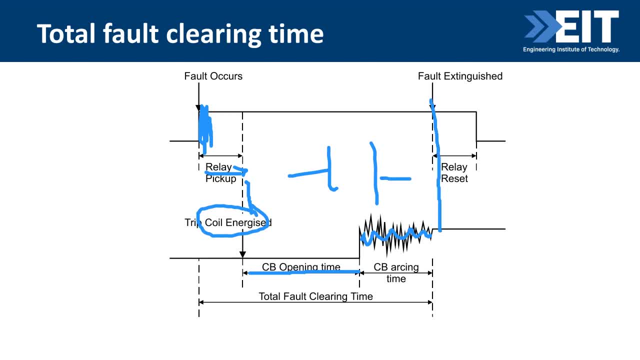 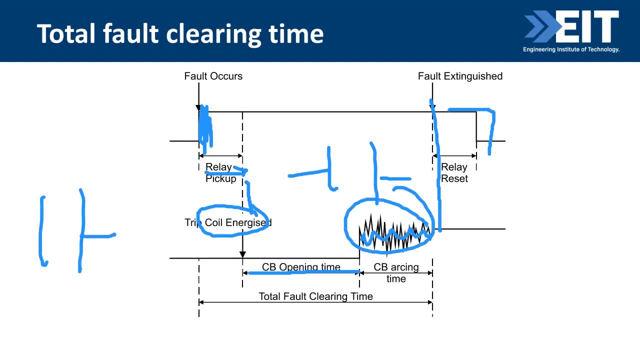 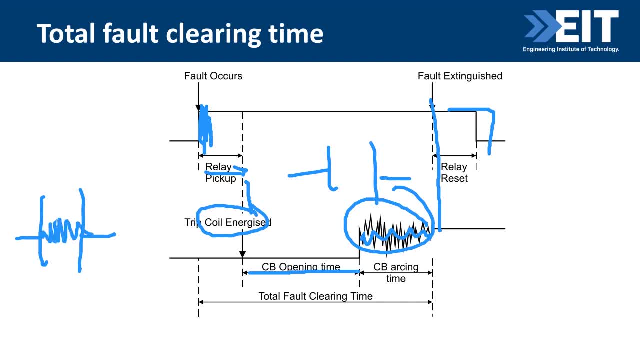 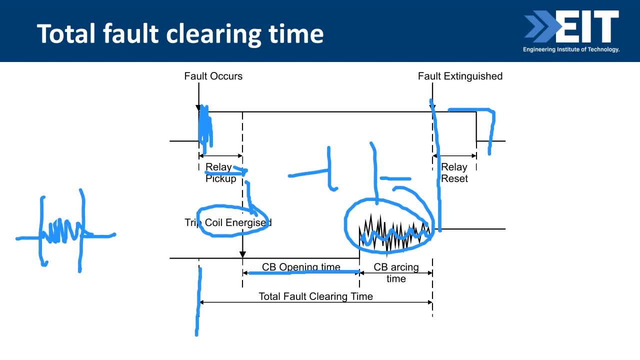 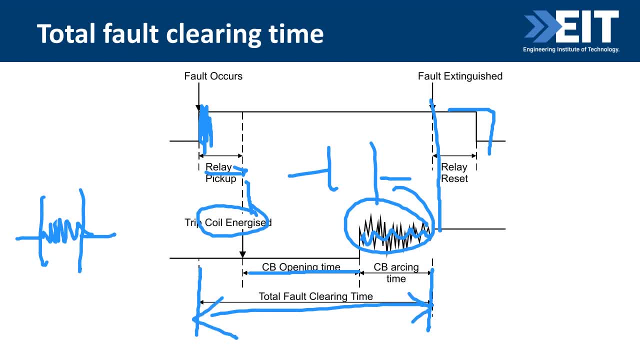 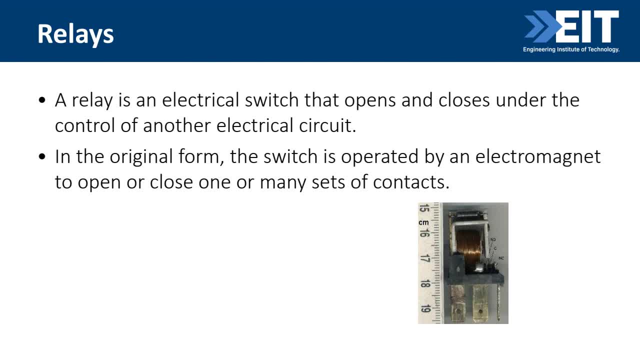 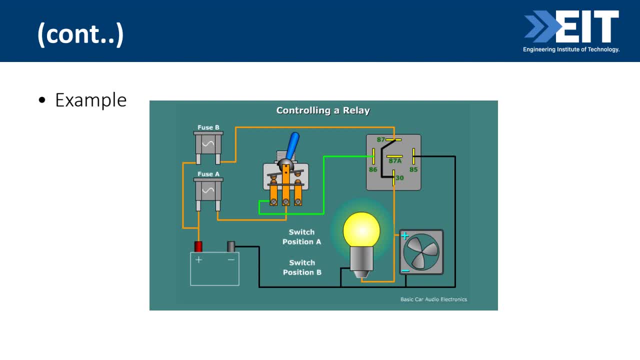 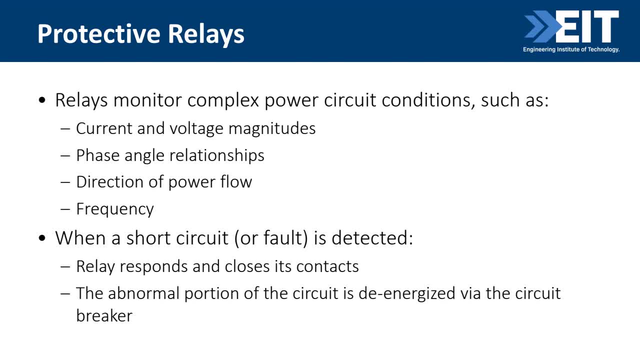 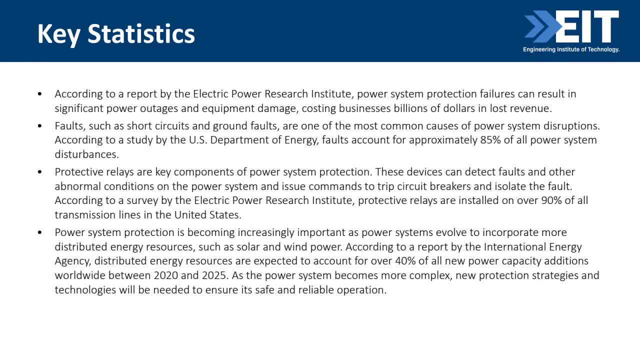 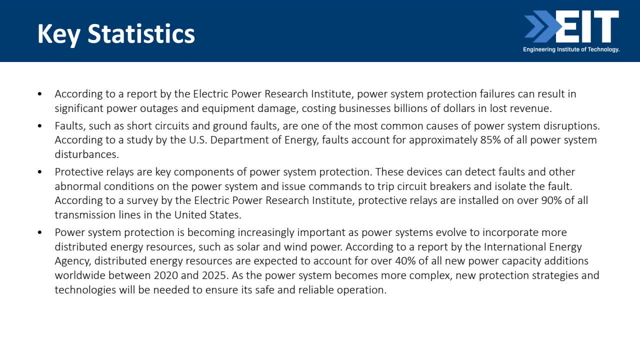 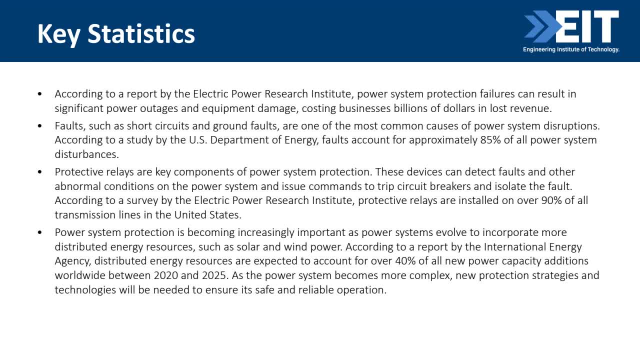 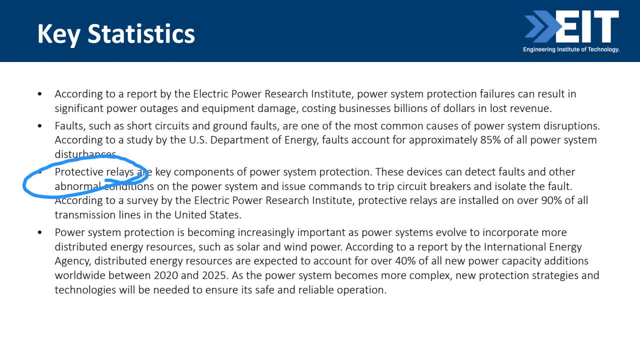 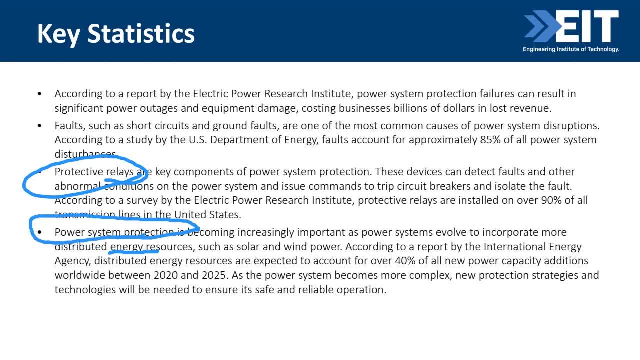 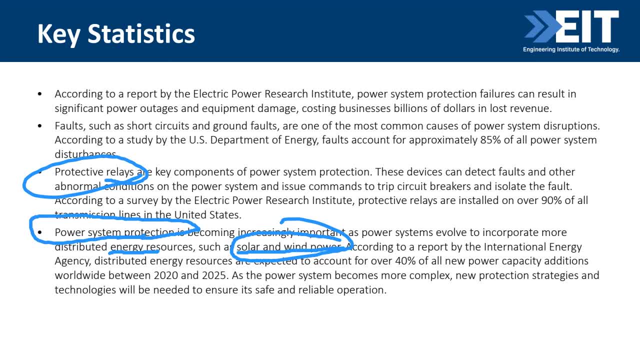 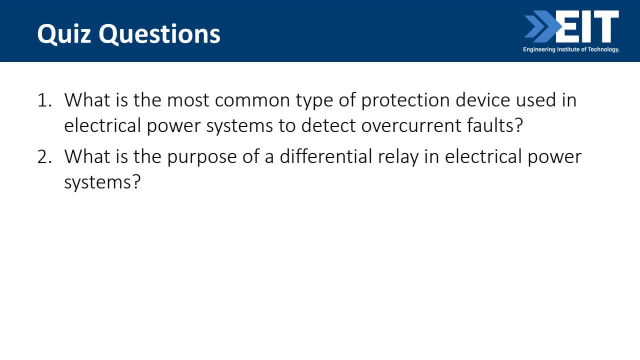 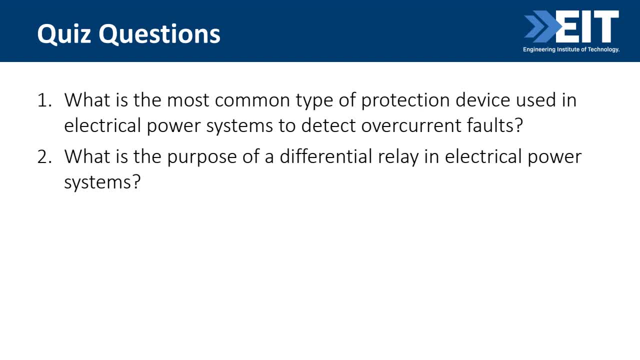 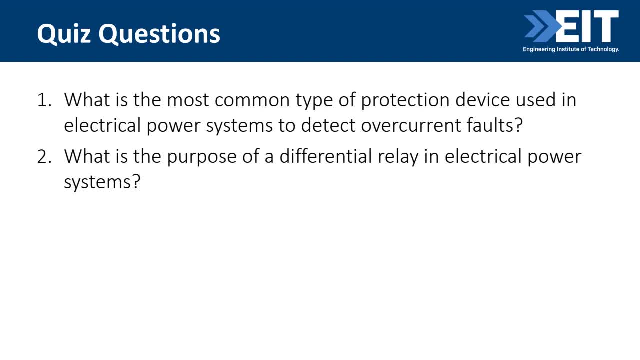 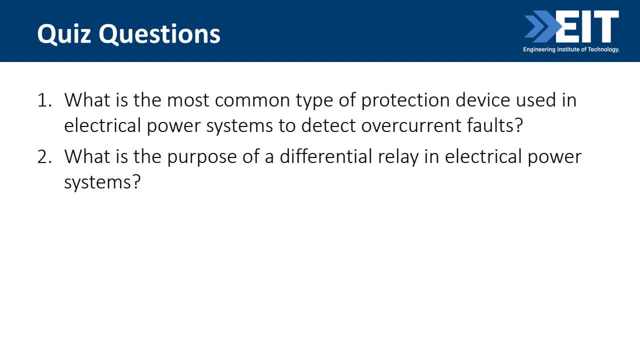 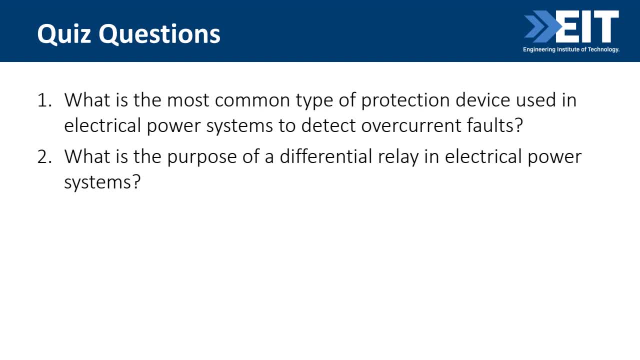 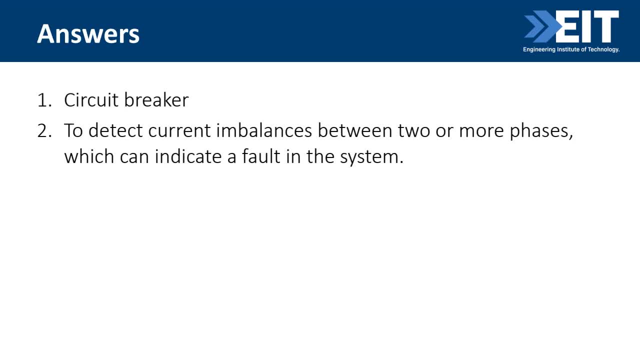 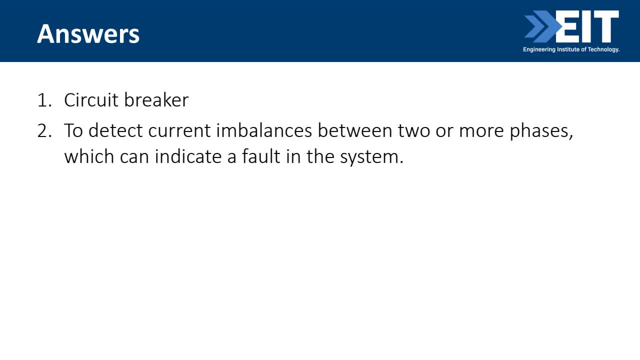 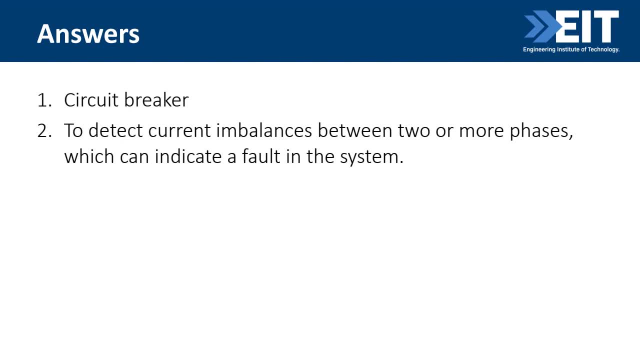 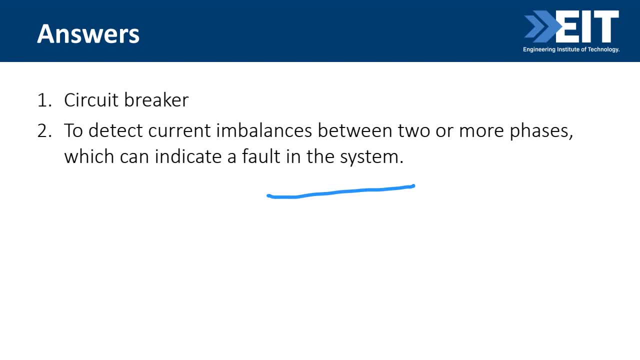 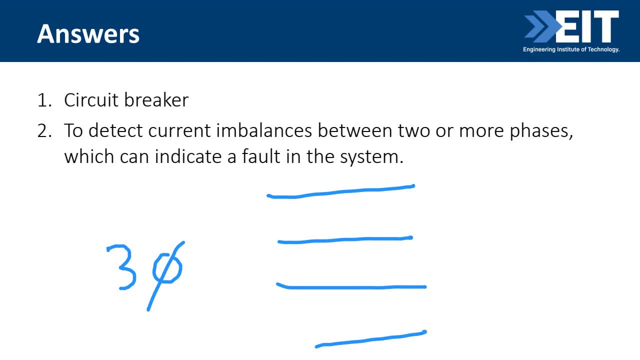 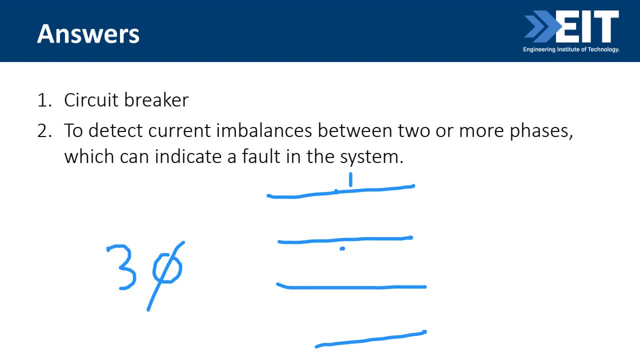 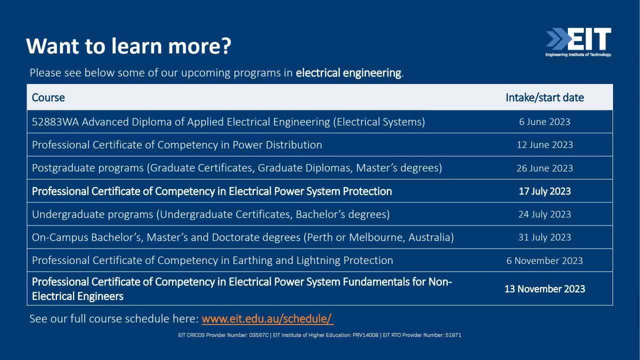 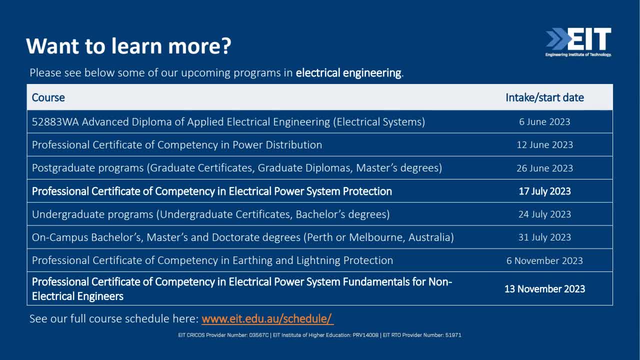 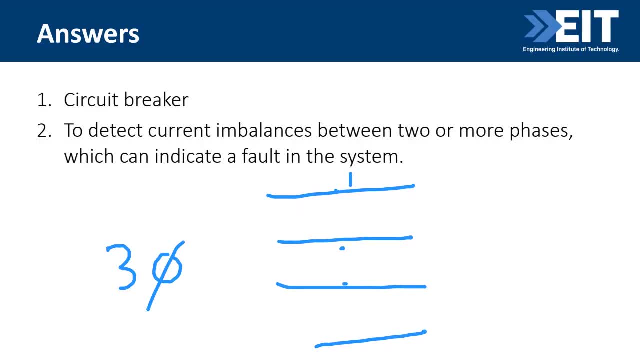 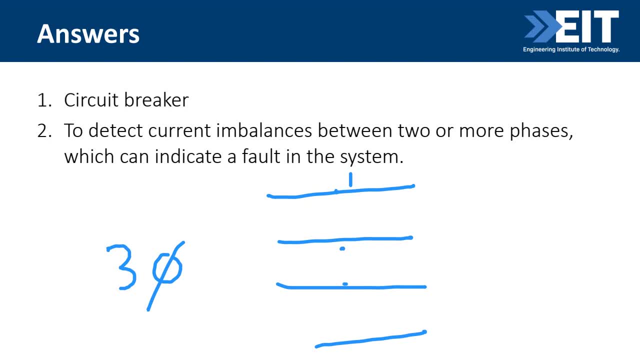 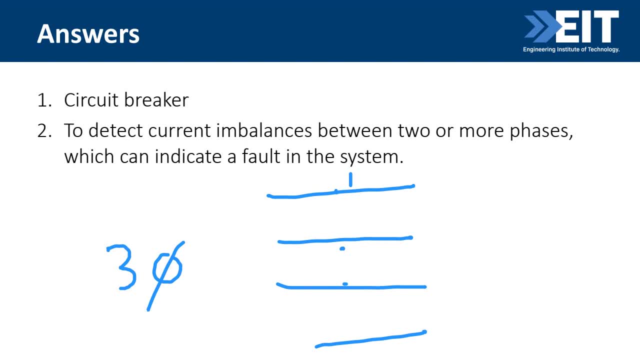 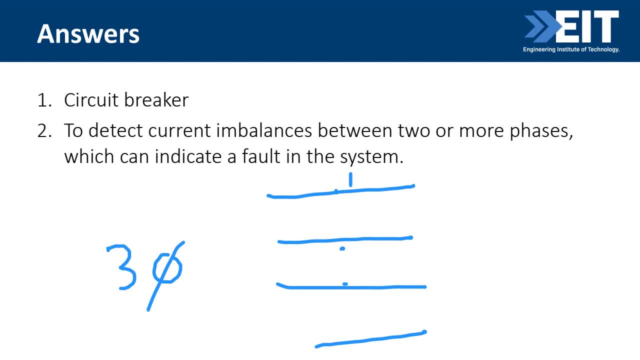 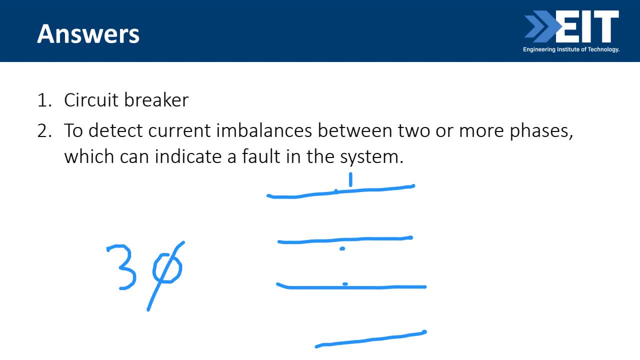 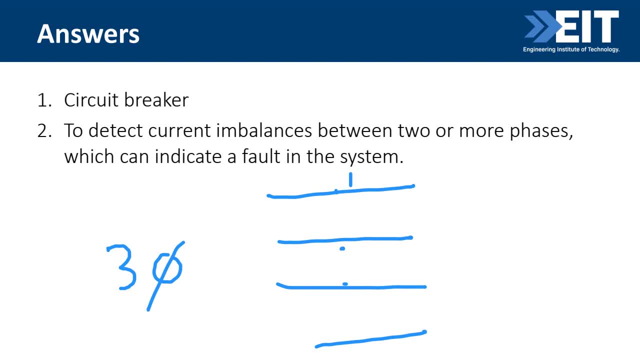 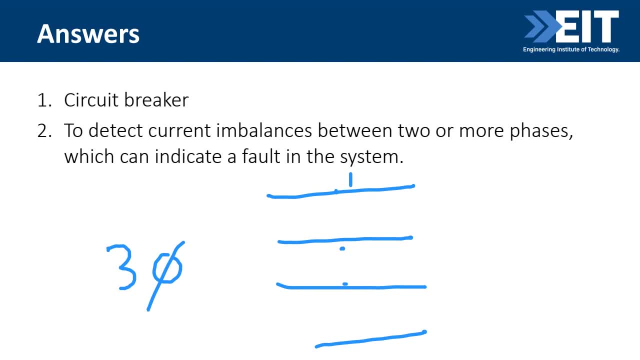 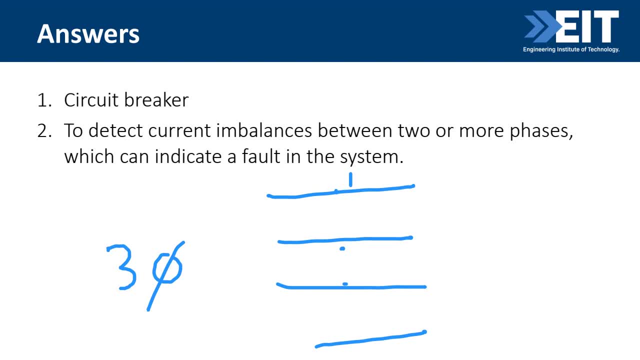 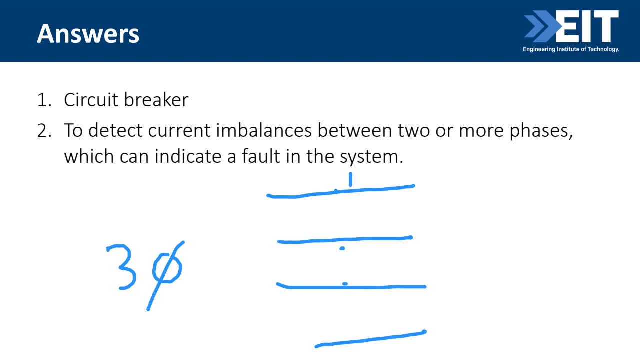 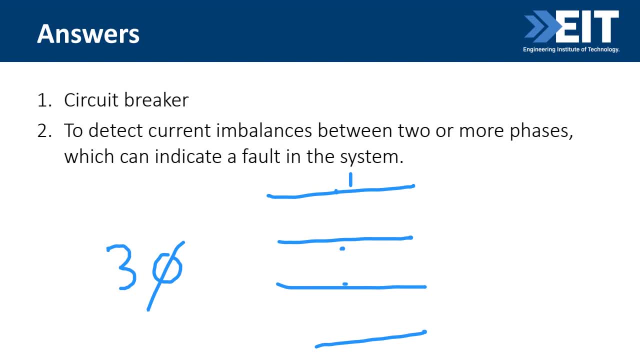 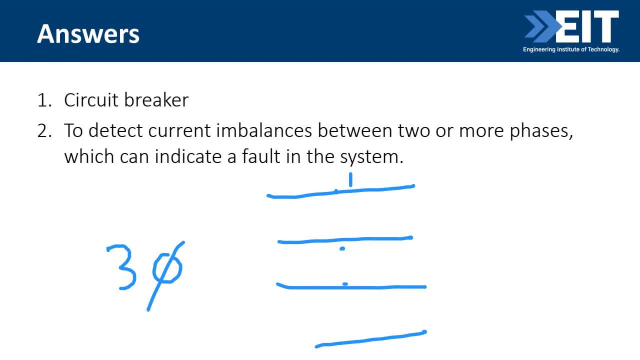 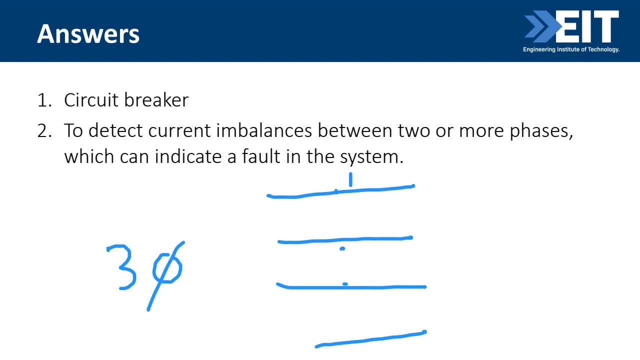 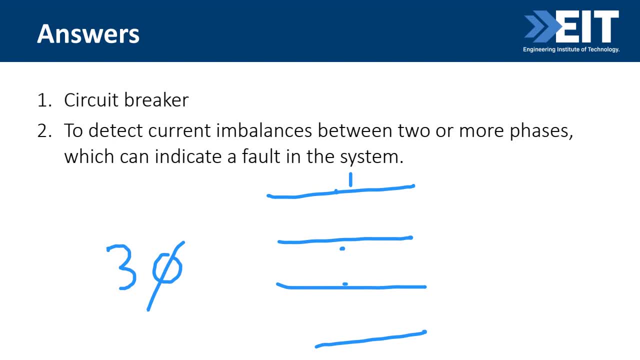 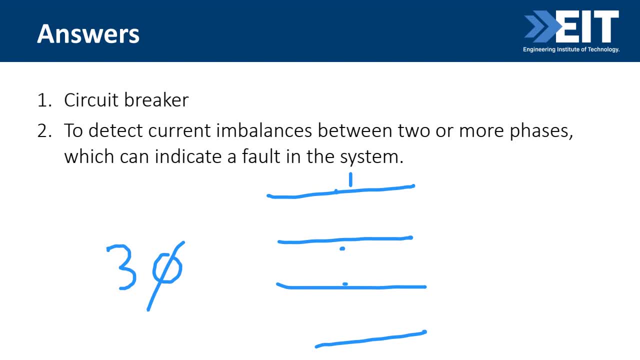 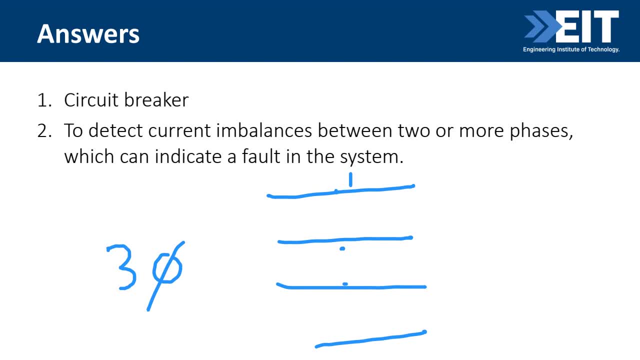 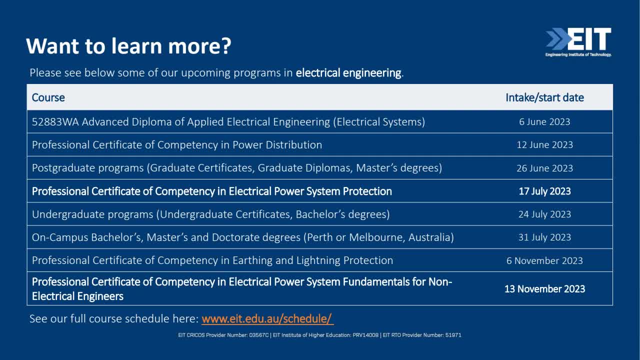 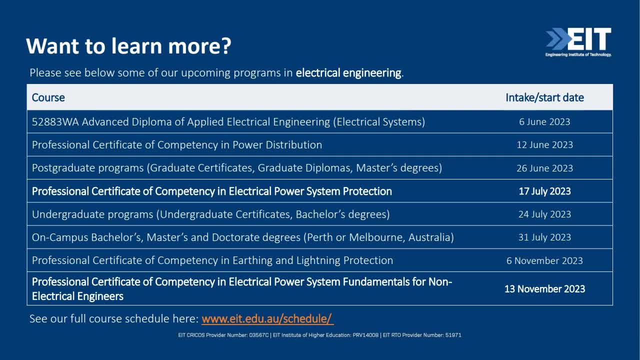 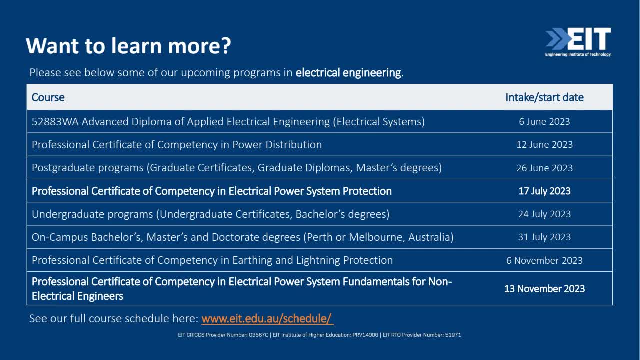 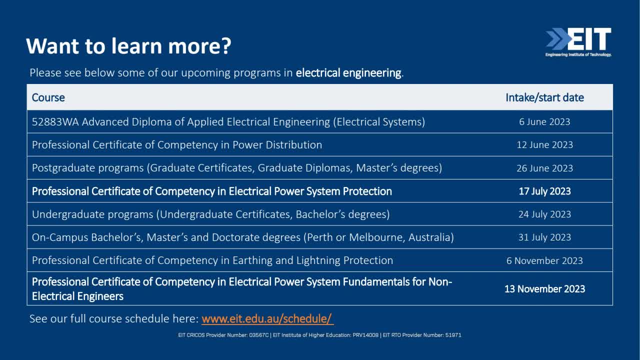 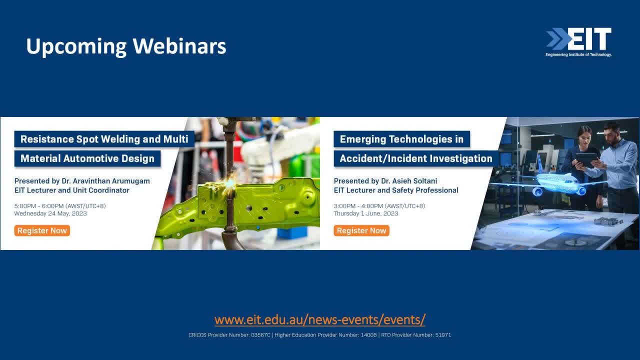 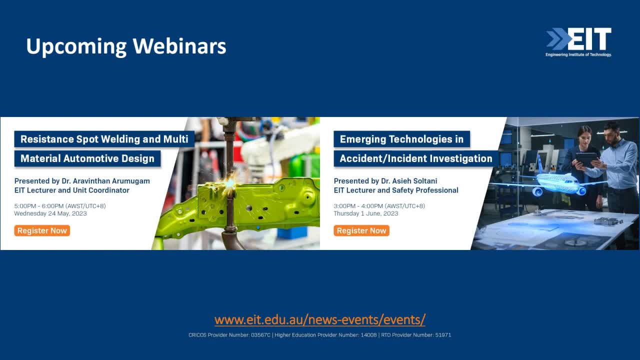 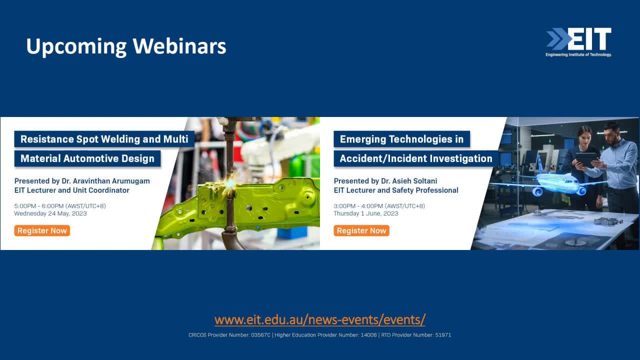 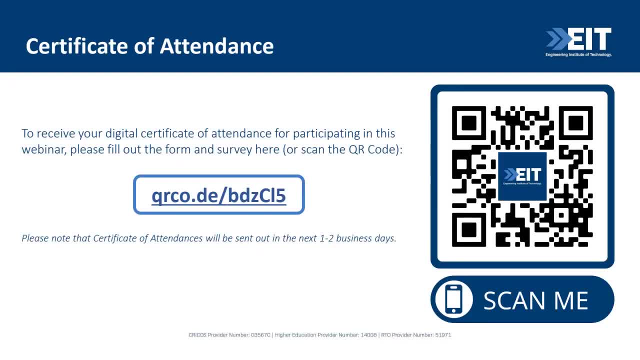 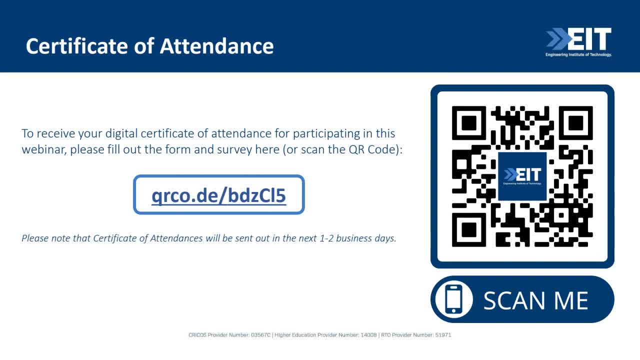 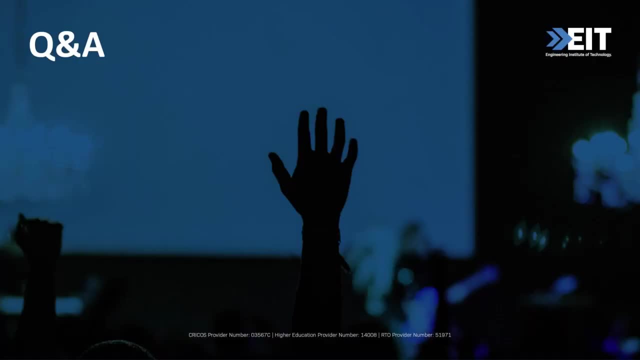 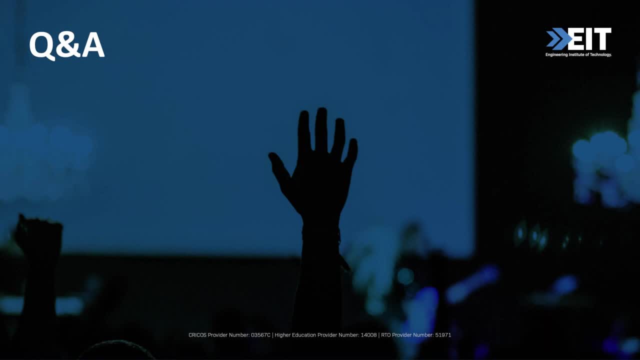 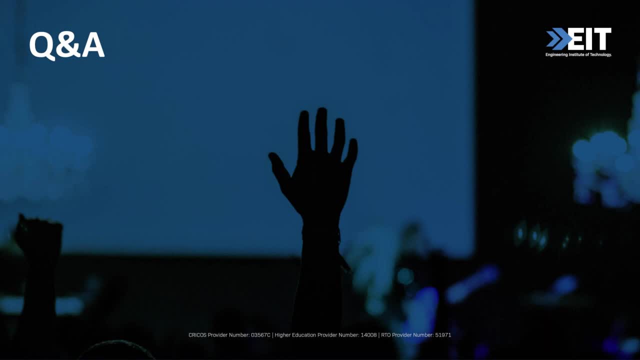 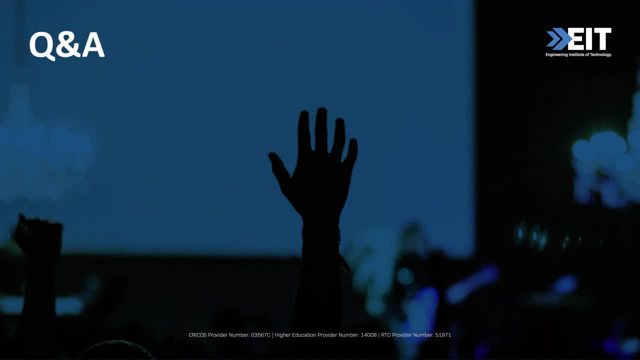 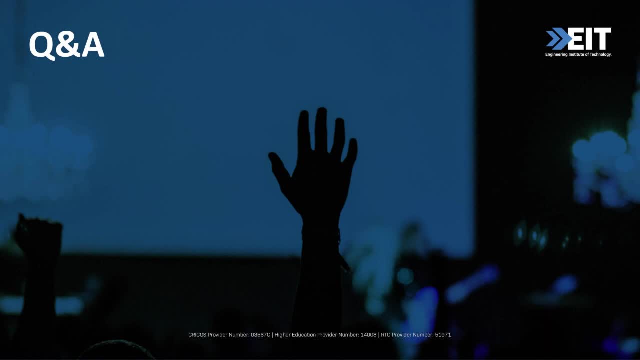 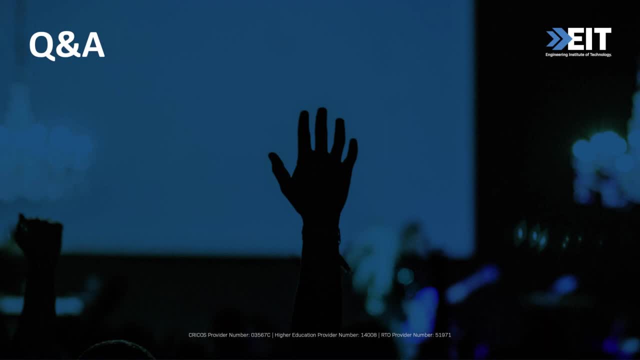 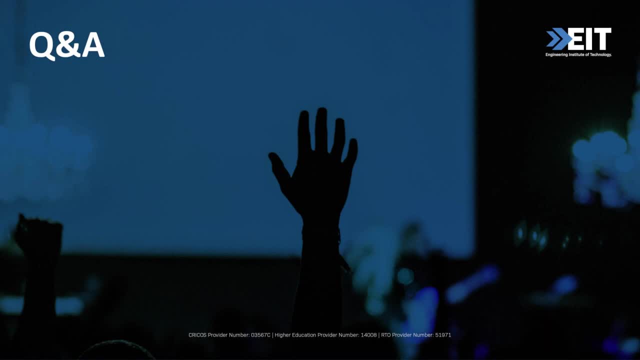 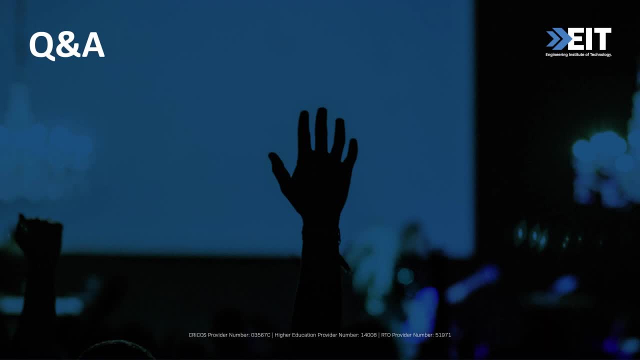 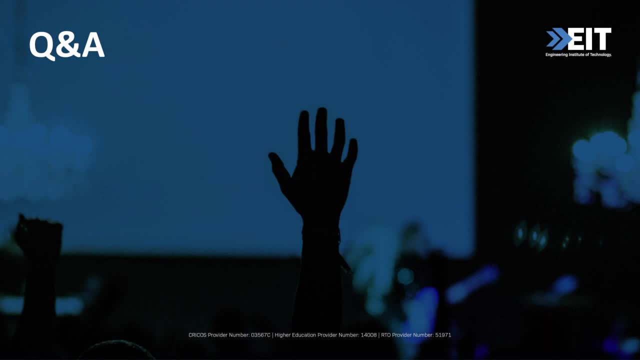 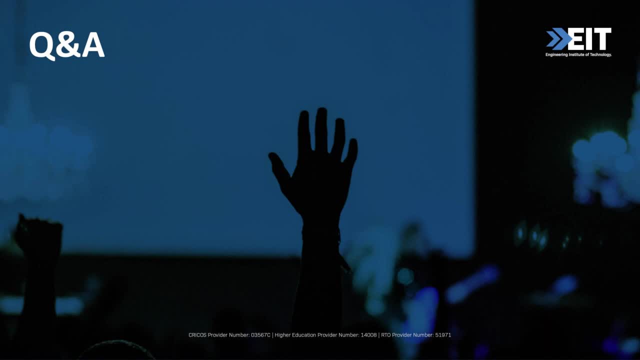 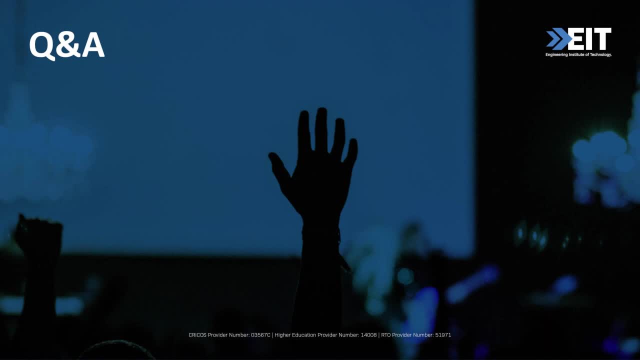 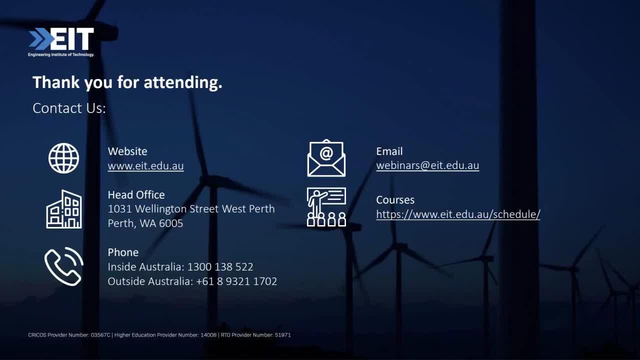 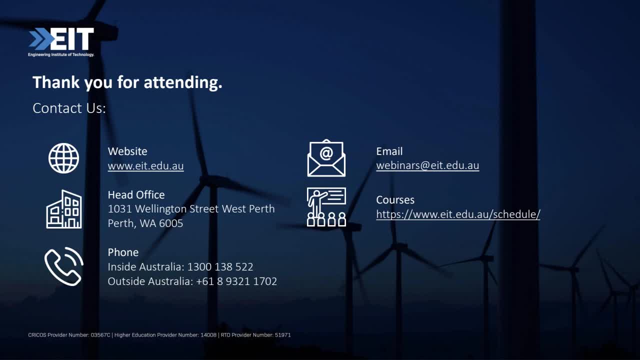 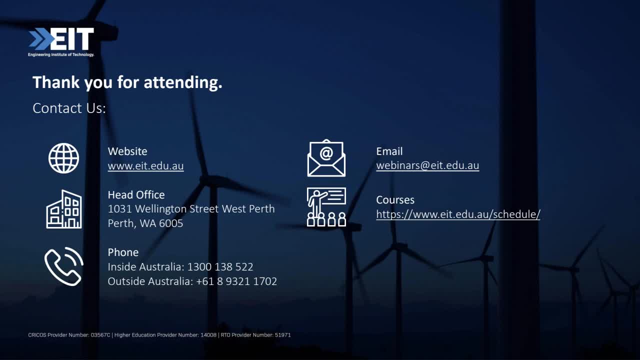 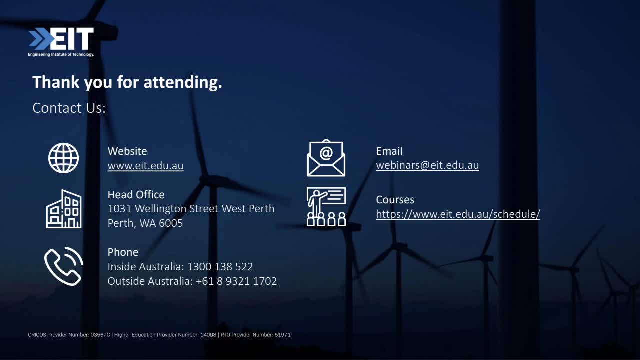 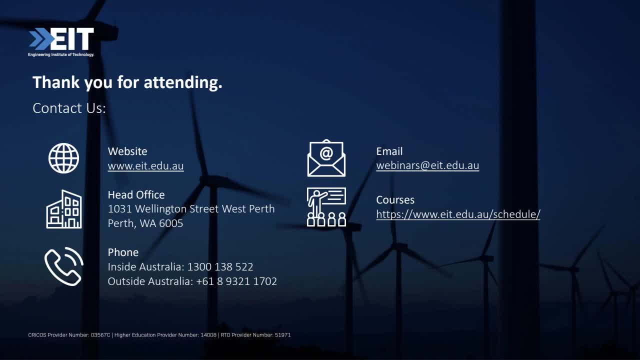 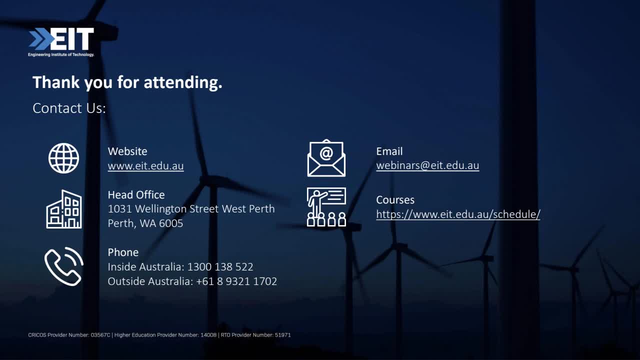 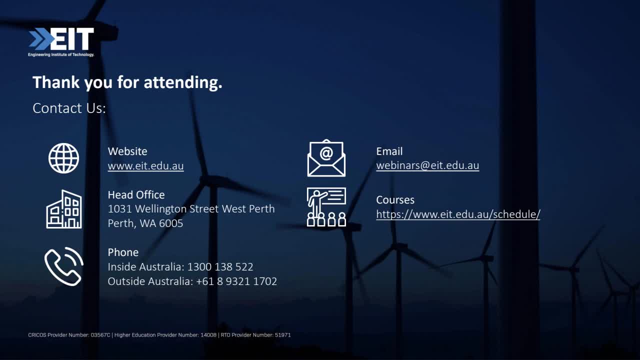 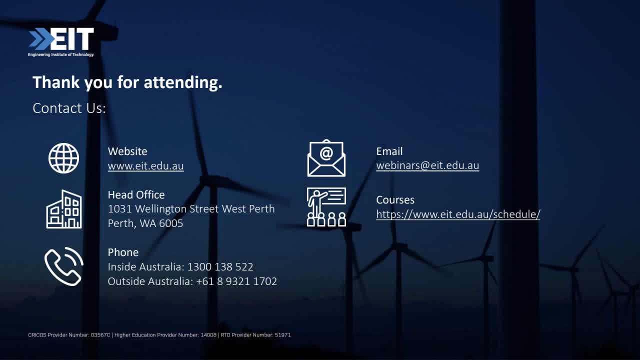